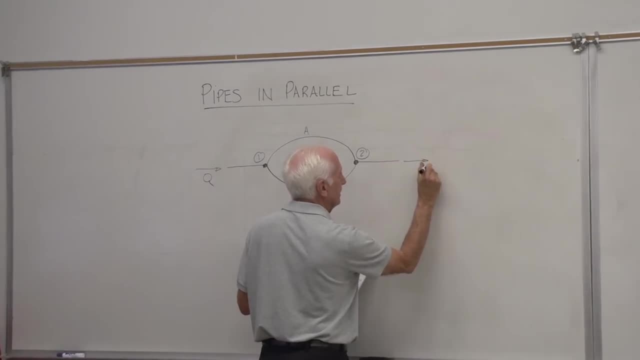 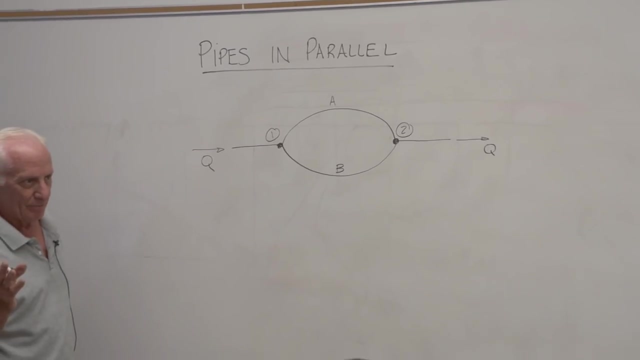 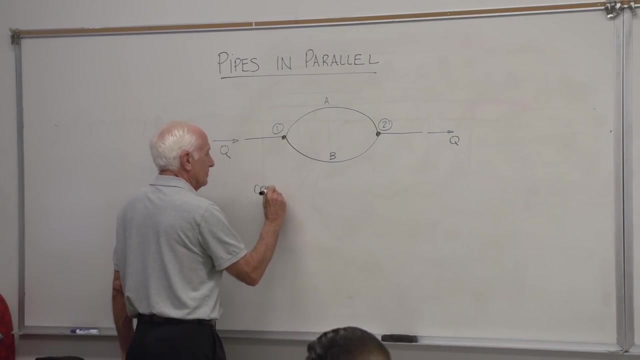 and the flow rate leaving the parallel pipe, of course, is Q steady state. Some of the flow goes through pipe A, some of the flow goes through pipe B in parallel. First of all, continuity: The flow that comes in Q equal QA plus QB. 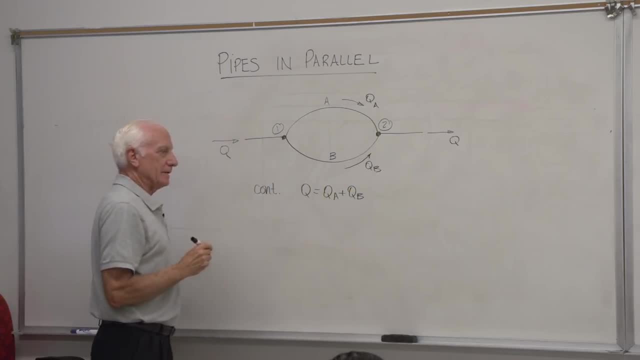 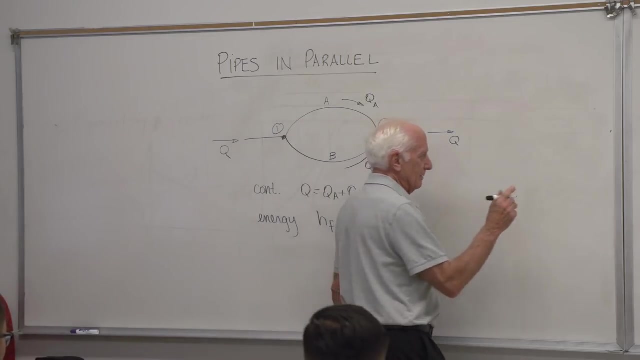 The head loss equation: energy HFA equal HFB. The head loss due to friction in pipe A: equal the head loss due to friction in pipe B. Okay, that's energy equation Contract. I'll go back and I'll contrast that with what we did for pipes in series. 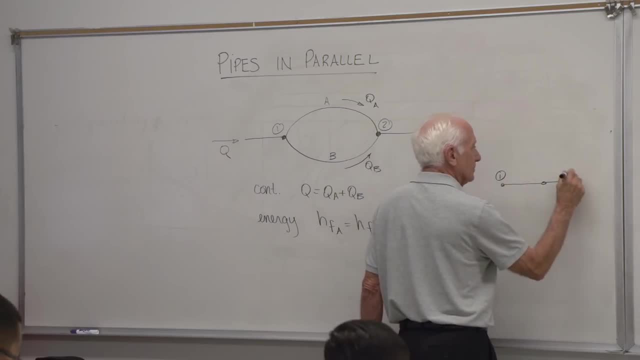 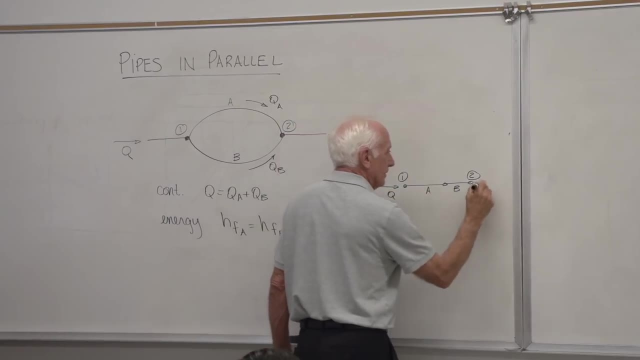 Real quick, I'll do this. This was point 1,, this was point 2,. this was pipe A, this was pipe B. This was the flow rate: Q. this is Q. this is QA. this is QB- Conservation of mass. The flow that goes through pipe A must equal the flow that goes through pipe B. The head loss equation- The total head loss due to friction- is equal the head loss due to friction in pipe A plus the head loss due to friction in pipe B. 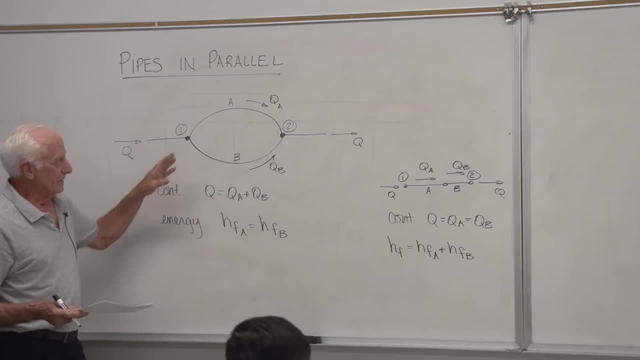 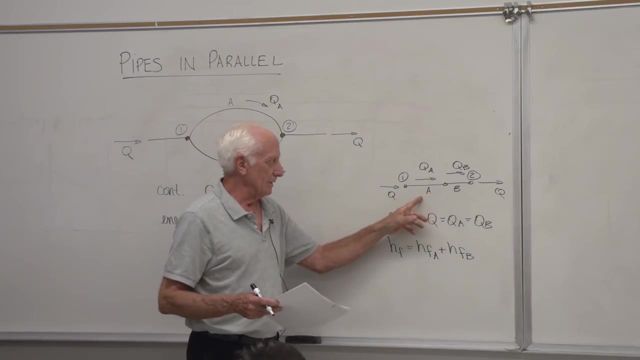 Okay, so there's two simple ones: side by side, parallel, and series- Conservation of mass. If they're in series, the flow rate in each pipe is the same to the flow rate coming in. If it's in parallel, the flow rate coming in equals the flow rate. 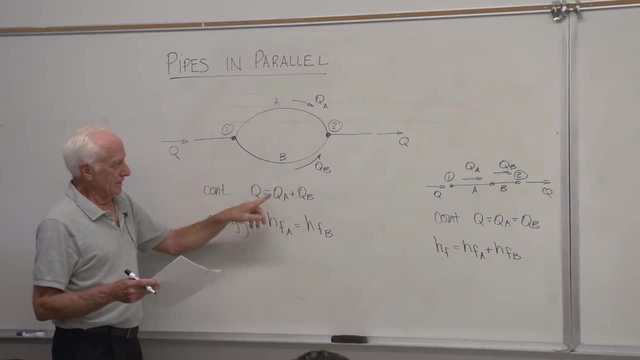 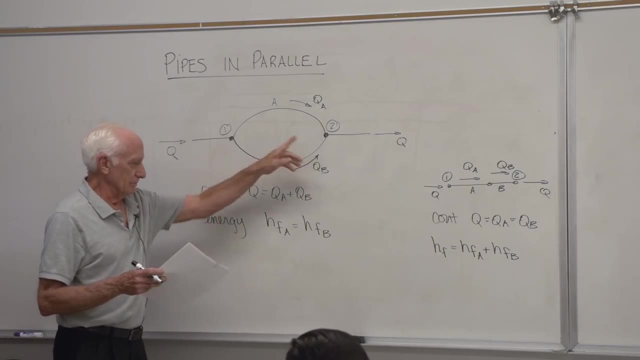 through pipe A plus the flow rate through pipe B. These guys add: these guys are equal. Now the energy equation from one to two: Okay, assume it's horizontal. Okay, HFA the head loss through pipe A, equal HFB the head loss through pipe B. 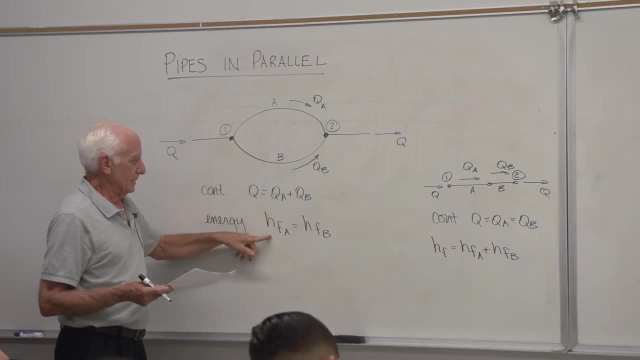 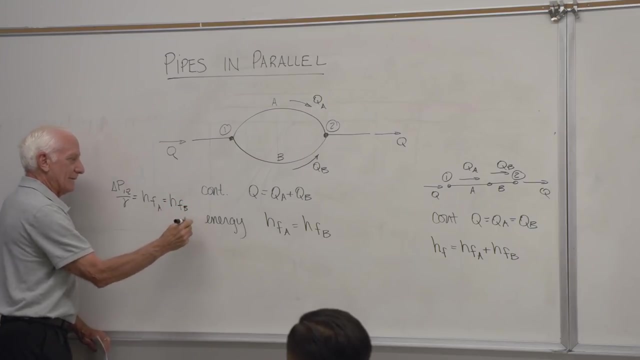 Maybe to put it in more general terms, because the head loss can be related to the pressure drop. Delta P one to two over Gamma is equal to HFA, equal HFB. That's the energy equation from one to two. So HFA is related to the pressure drop one to two. 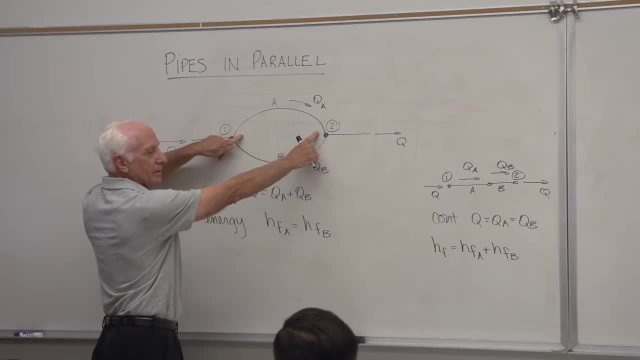 If I've got this pipe and the pressure drop in this pipe is 10 psi, the pressure drop in pipe B has to be 10 psi, has to be 10 psi. So that's HFA, equal HFB. That's where it comes from. 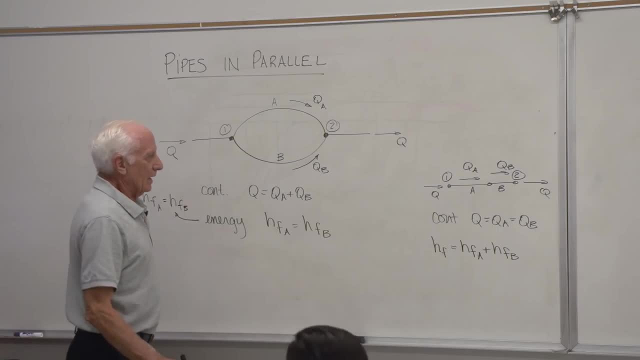 the energy equation If they're in series, if the pressure drop in pipe A is 10 psi and the pressure drop in pipe B is 10 psi, guess what? the pressure drop from one to two is 10 plus 10 is 20.. 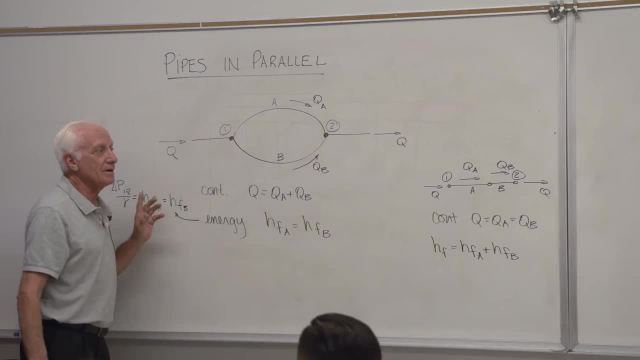 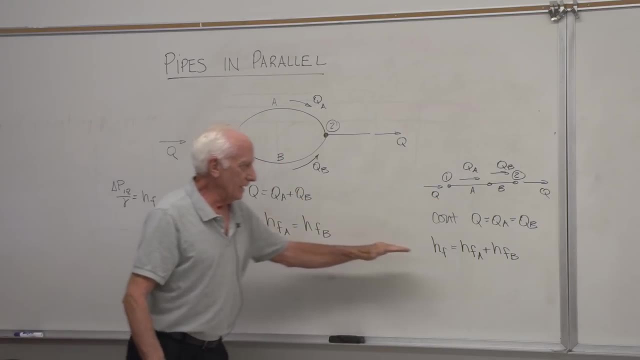 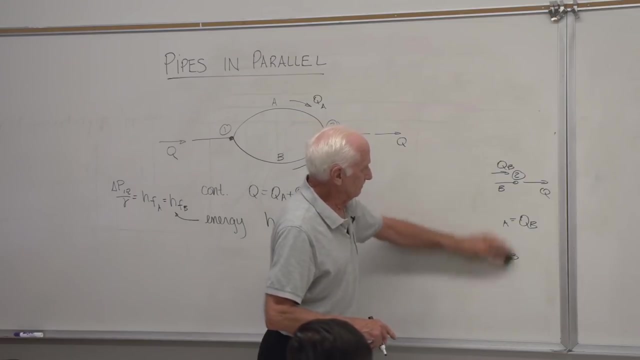 Right, So they're different. Qs add Qs are equal. HFs are equal. HFs add Series parallel. that's the difference. I'm going to erase him now because we did this last time. Now, last time with the series. 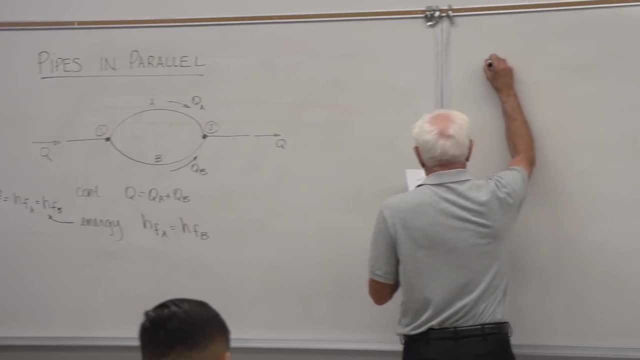 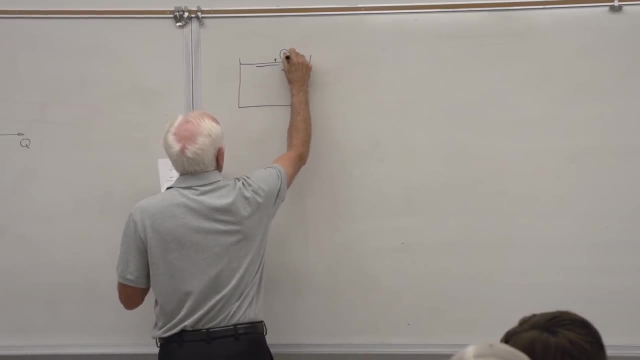 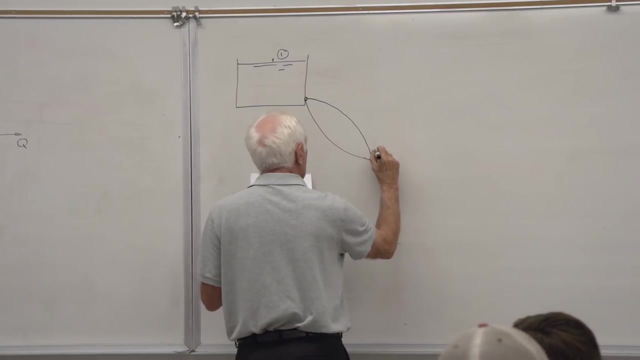 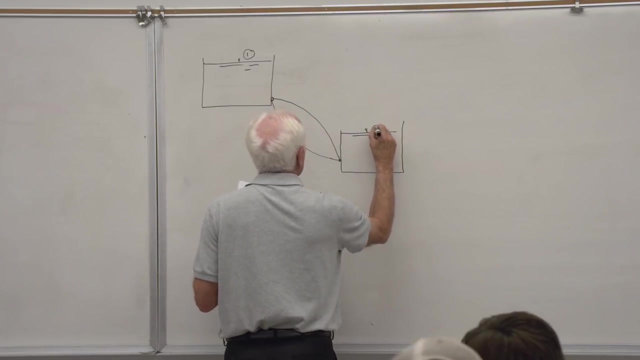 we also looked at this problem where we've got a reservoir here- and this is going to be 0.1, and we've got a pipe A and a pipe B going down here to a reservoir down here, which is our 0.2.. 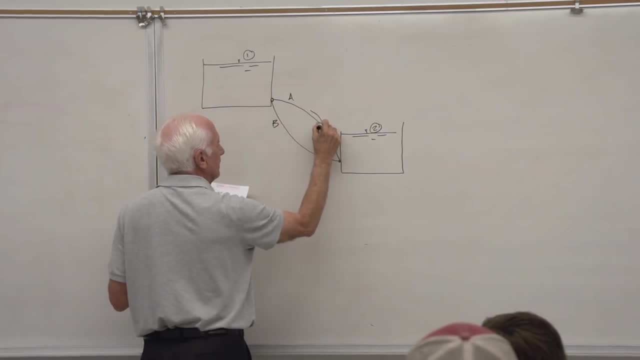 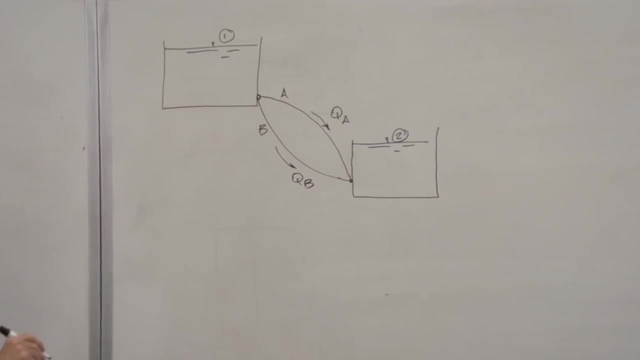 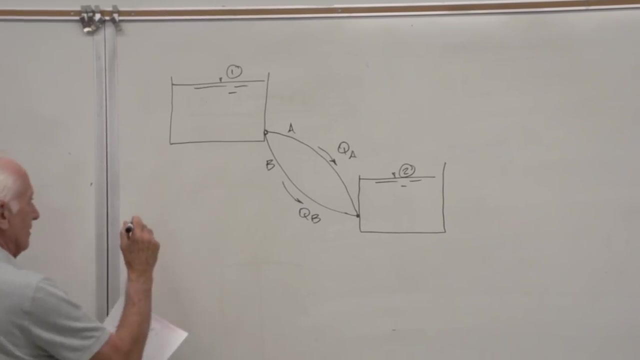 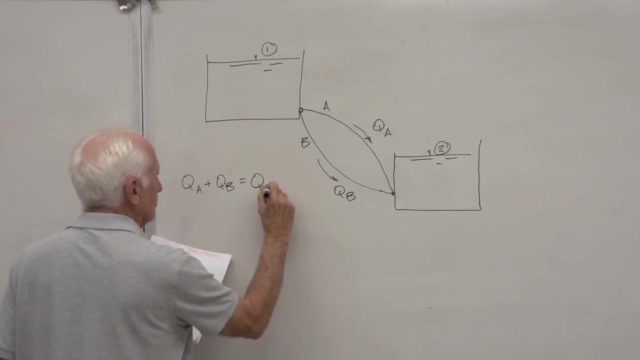 This is pipe A. this is pipe B. QA, QB- The same equations hold out. write them down: QA plus QB: equal the total flow rate from the two reservoirs. Q- Okay, Energy. Now energy Delta. Z is equal to HF A or HF B. 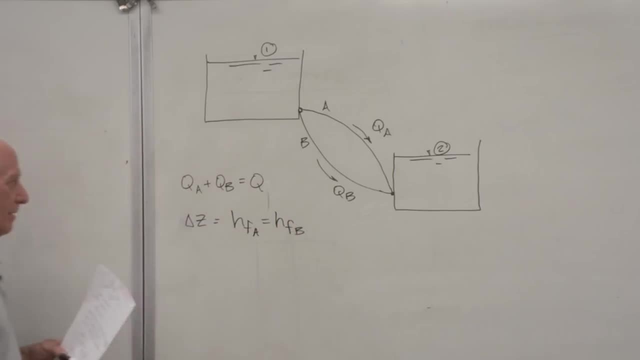 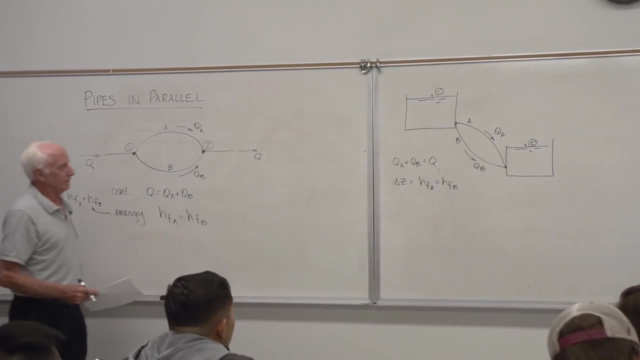 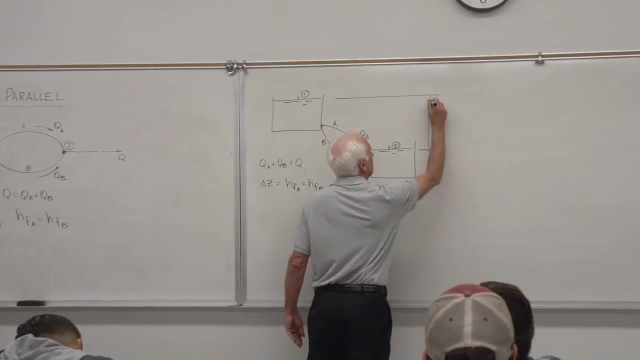 Take your choice, it's the same. Okay, Here here. here you see how similar they are. So over here somebody could ask you, as maybe the homework we just did, There's Delta Z If Delta Z is 50 meters. 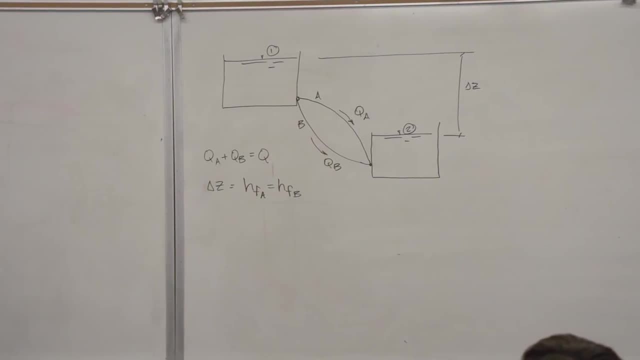 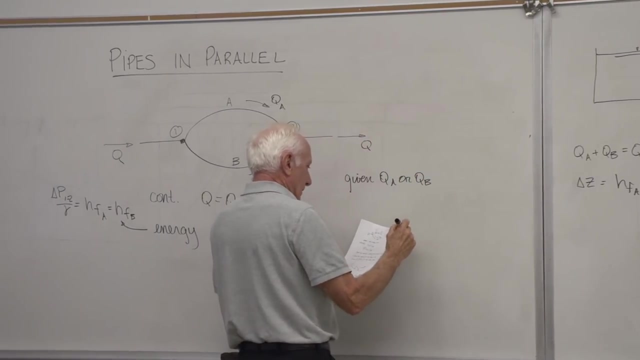 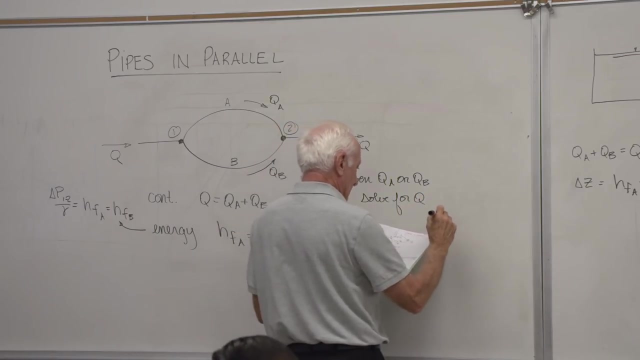 what's the flow in pipe A? what's the flow in pipe B? Matter of fact, I'll write down what kind of things you could be given and asked for A problem like this. you could be given QA or QB, Solve for Q, solve for either one, you don't know. 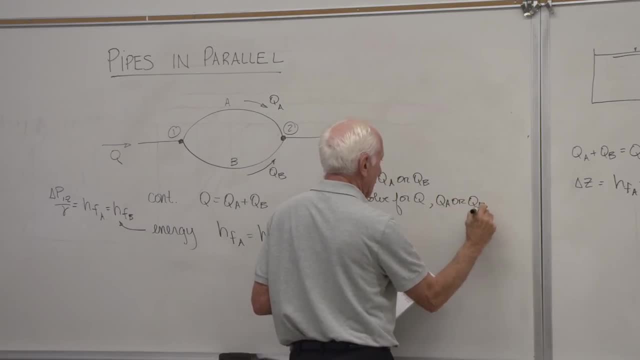 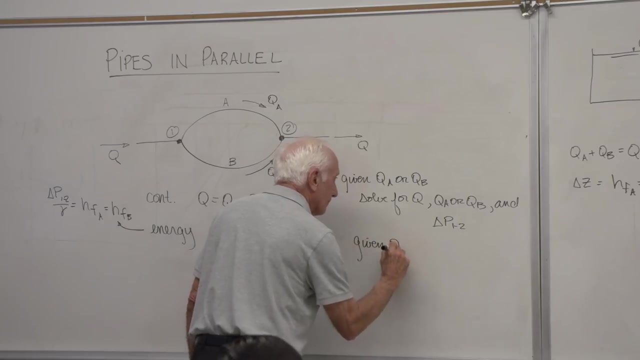 QA or QB and solve for, let's just say, the pressure drop one to two Or you could be given the total flow rate Q, Solve for again QA, QB, Delta, P one to two, Or you could be given. 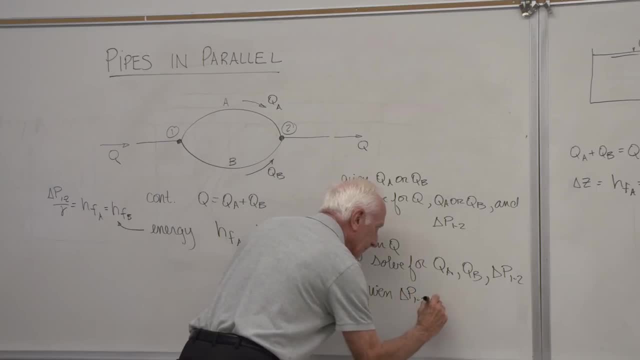 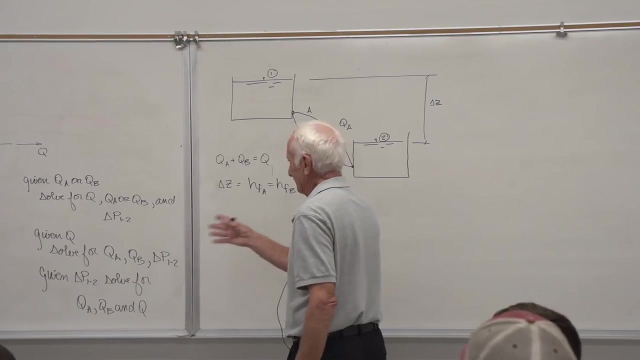 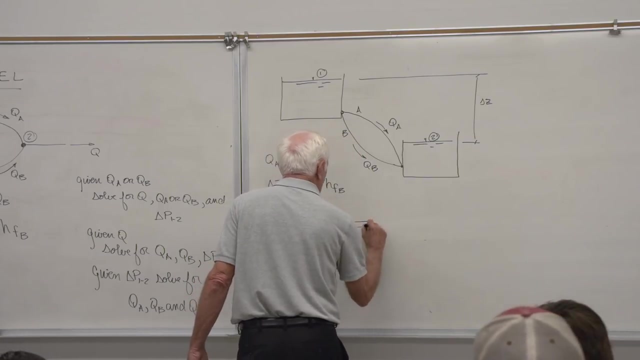 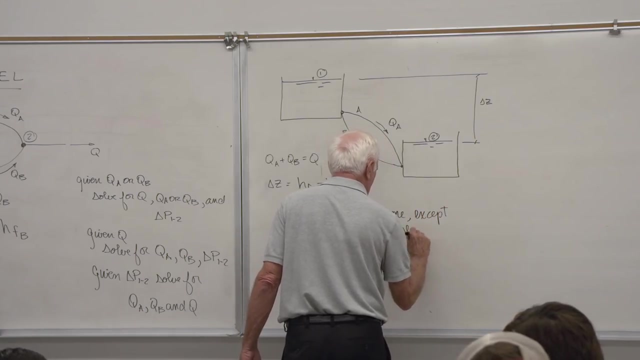 Delta P one to two to P 1 to 2.. Solve for QA, QB and Q. Okay, let's go over here This guy. actually, it's the same thing, just replace delta P with delta Z. Same except replace delta P. 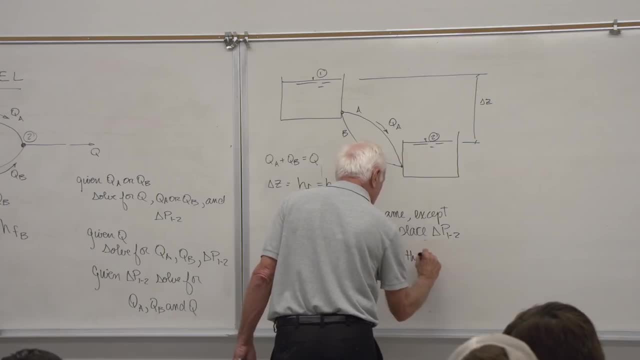 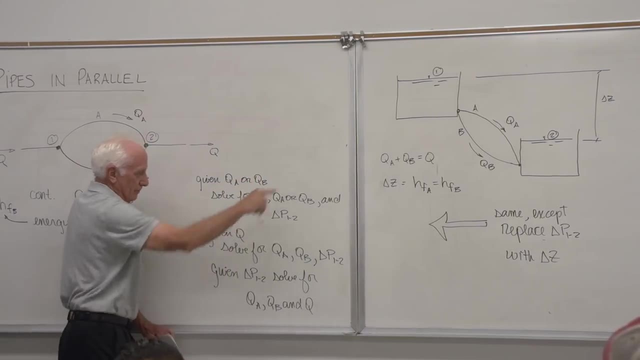 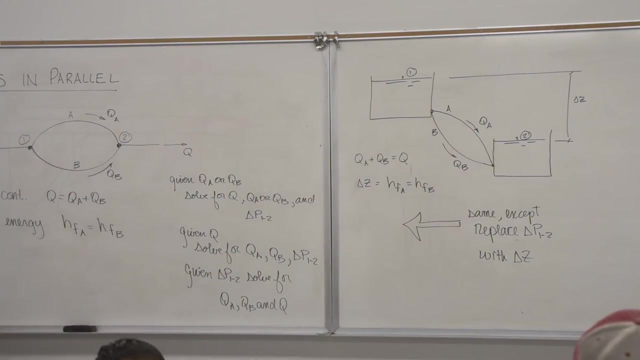 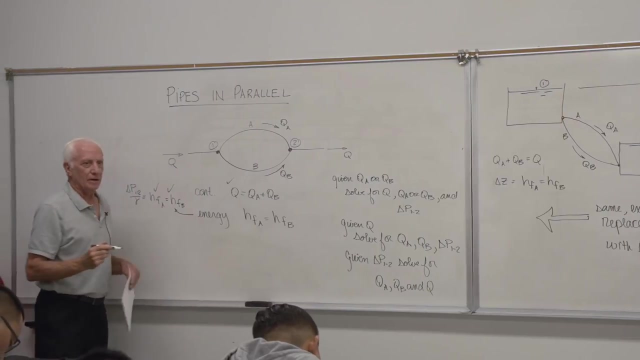 1-2 with delta Z, For instance, given the total flow rate Q in that problem, solve for QA, QB and delta Z. Okay, that's what it means. Three unknowns how many equations: One, two, three. There they are: Two energies, one continuity. 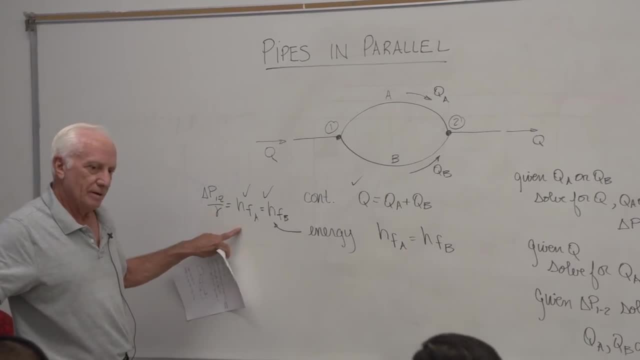 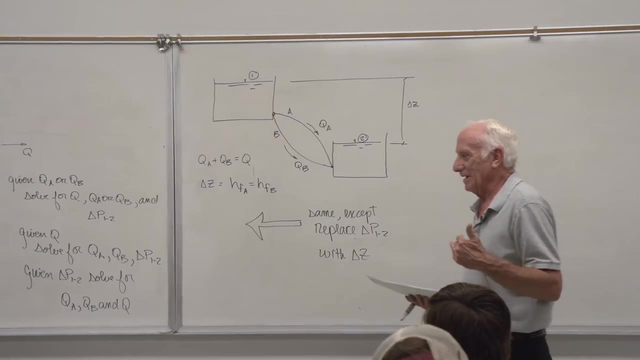 conservation of mass. That's two equations right here. equal sign, two equations, Okay. so first thing you want to identify is: what kind of problem do you have? For instance, what's that problem over there? I don't know, it's some big. 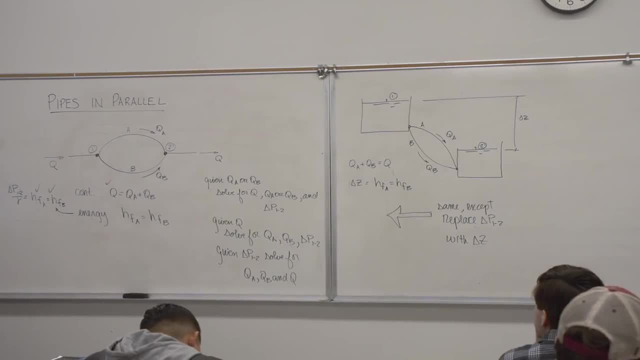 complex network. There are series pipes, there's parallel pipes. You're looking at one parallel pipe combination there. This one's two reservoirs, water flowing from one to the other, But this is very typical of those kind of problems. Okay, 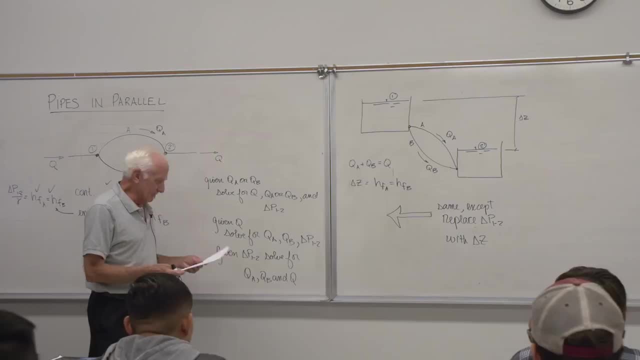 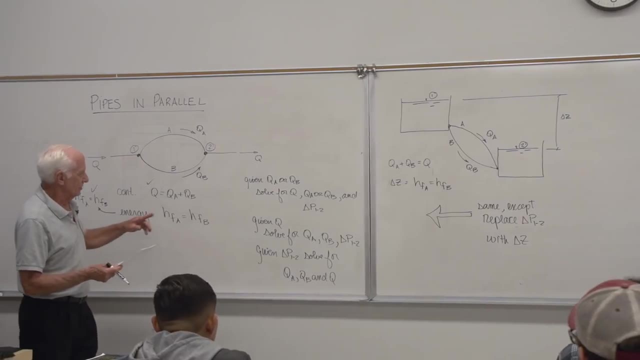 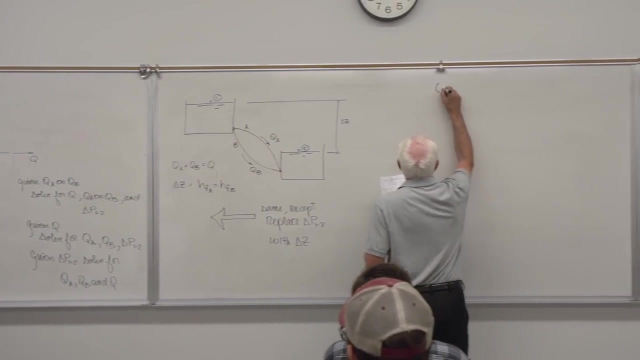 so we're going to take. let's see, I'm going to solve for delta P, so I'll do one of these guys. Delta P, Okay, Okay, Okay, Okay. I know QA. All right, I got this guy. So here's my problem: QA is given 0.100. 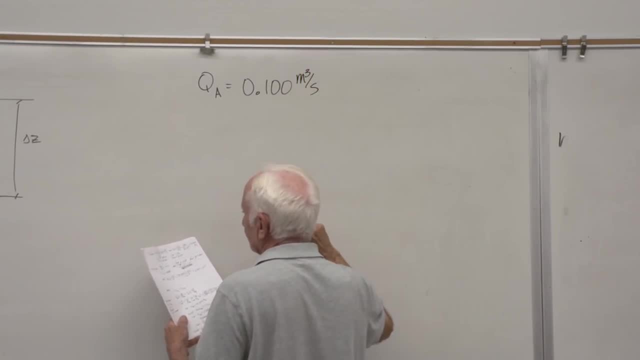 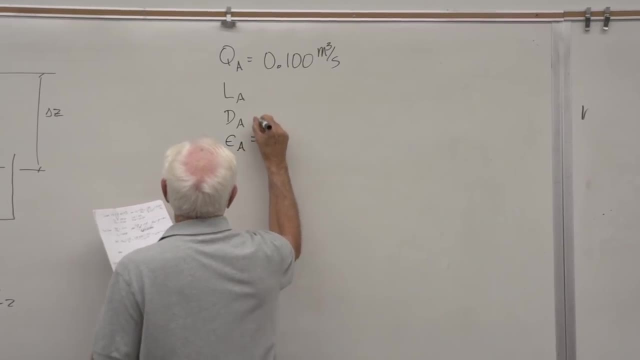 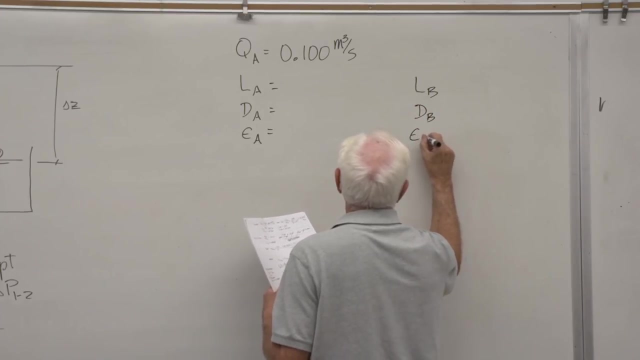 cubic meters per second. LA diameter of pipe A. roughness of pipe A Pipe B: 0.100.. All right, so 20 meters, 20 centimeters, Epsilon 1,100.. No, let's see. 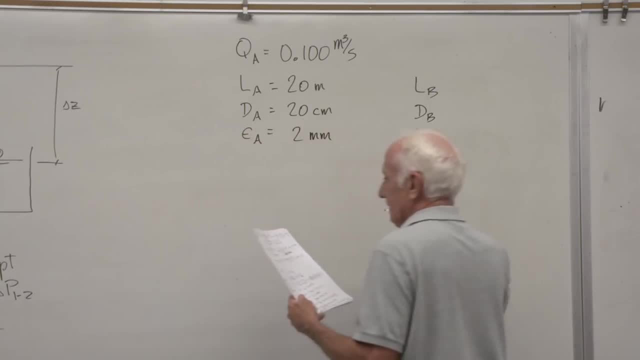 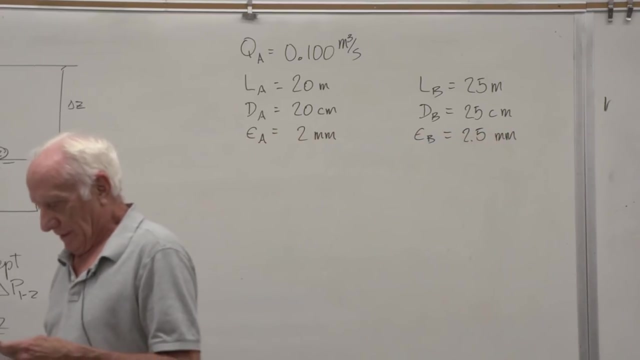 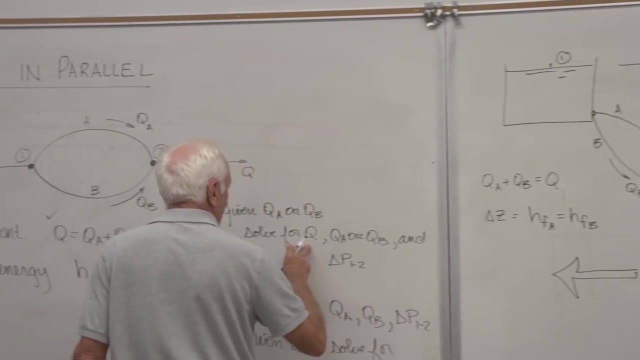 epsilon 2 millimeters. pardon me, All right, LB: 25 meters. Diameter of B: 25 centimeters. Epsilon sub B: 2.5 millimeters. Okay, Find Q. well, here it is. Find Q I know. 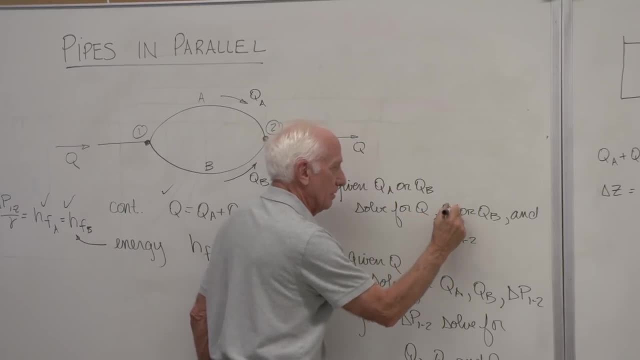 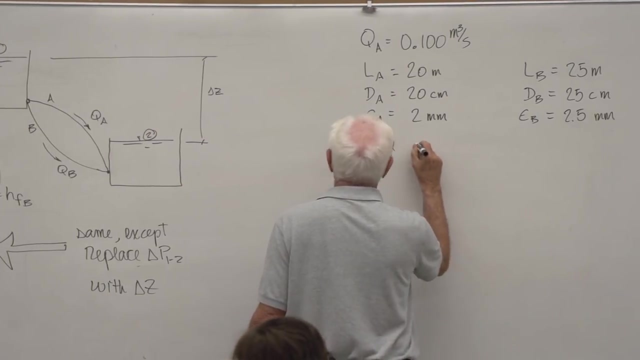 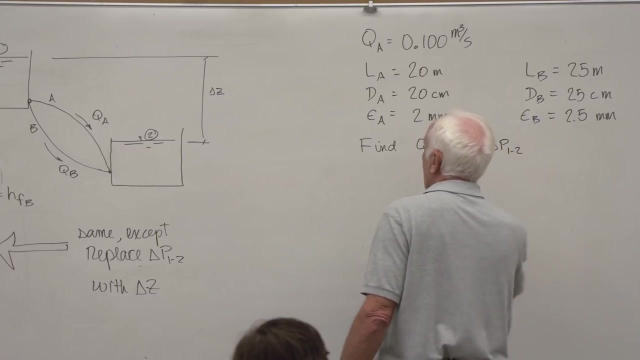 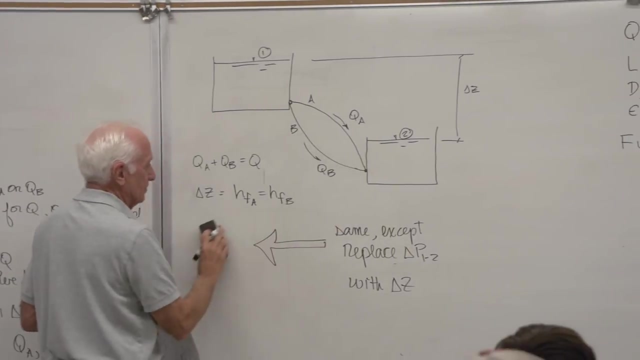 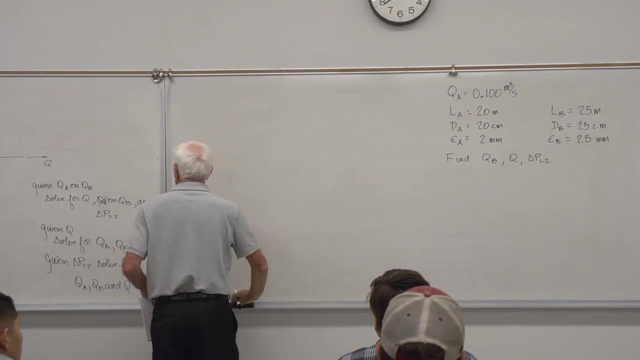 QA. yeah, Find Q QB delta P 1, 2.. Okay, And the problem, I'm going to erase this middle one now, so I make room here, So we're not doing this one. Okay, here they are. Here they are, I know QA. 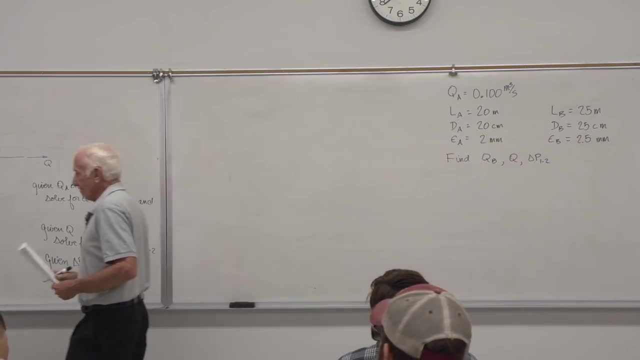 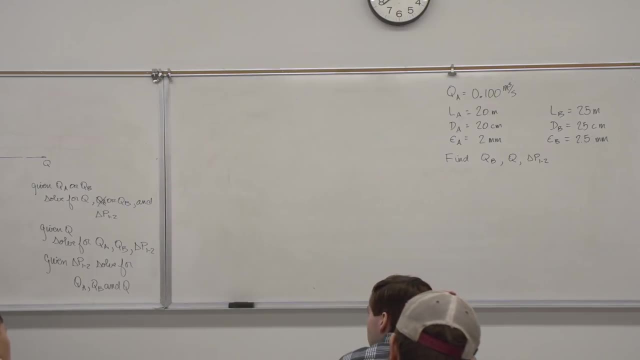 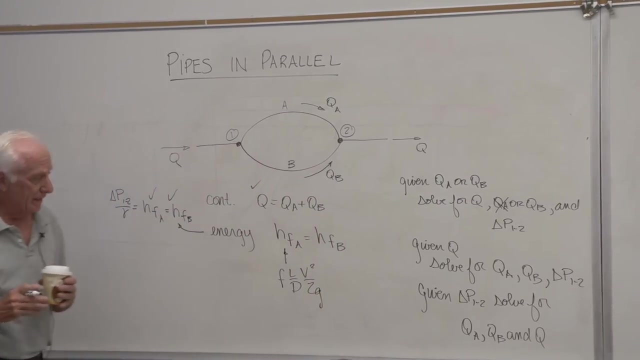 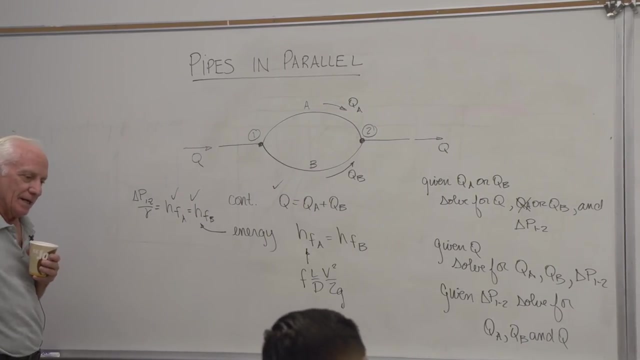 I don't know QB. Okay, When I use the energy equation HF, I need F. We know that. We talked about that last time. I need F. Sometimes I've got to guess F if I don't know the flow rate. but if I know the flow rate I can solve for F. I know the flow rate in. 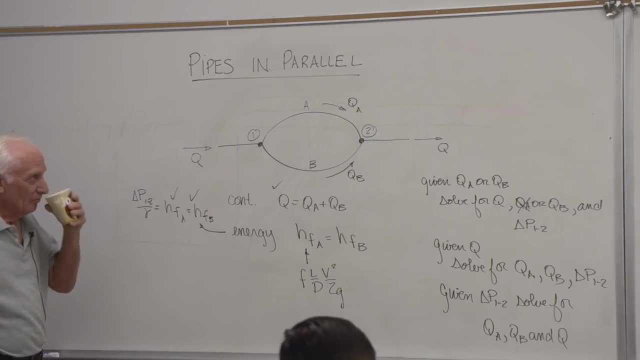 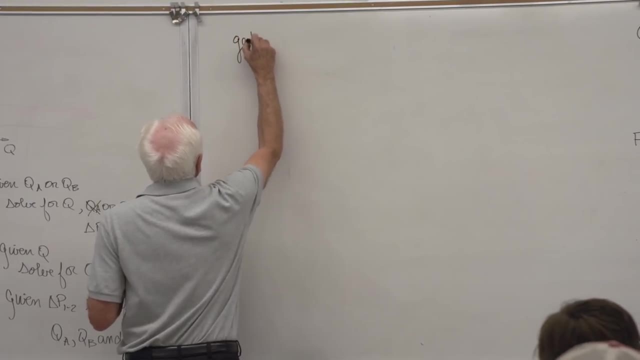 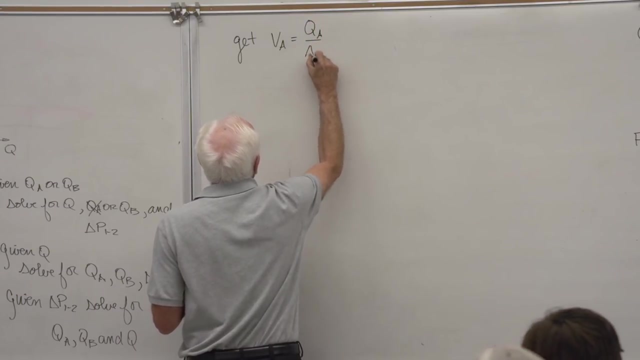 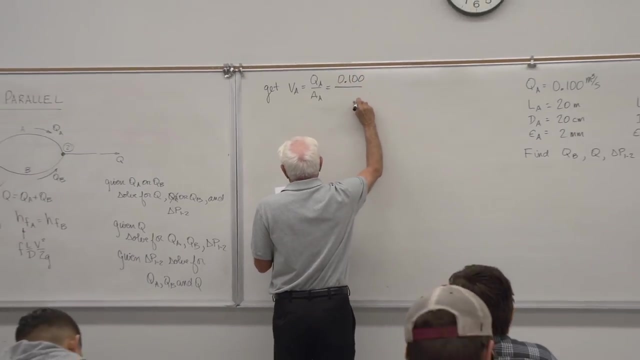 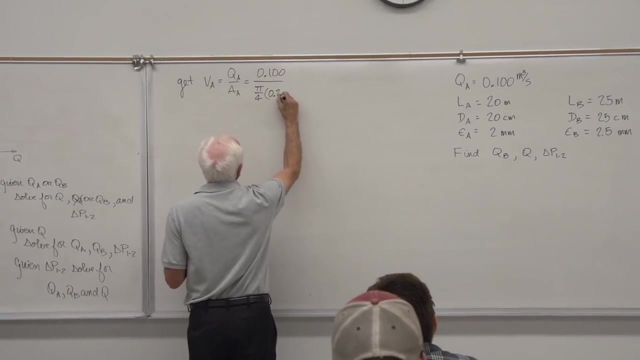 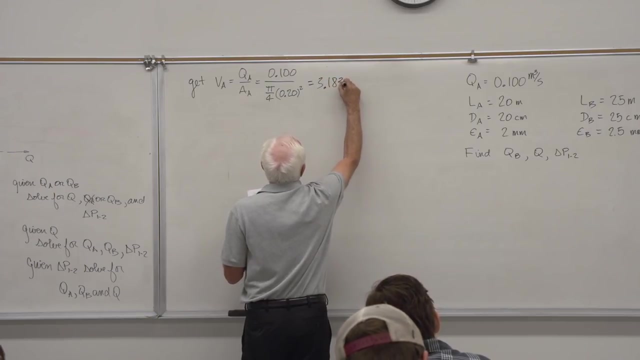 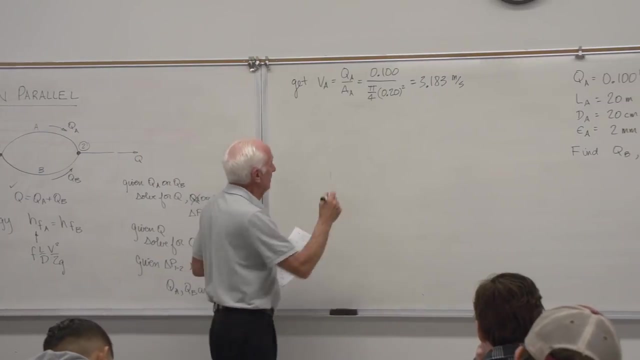 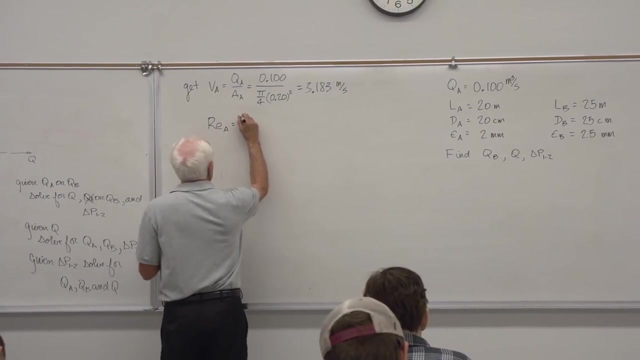 pipe A. I'm not going to guess. All right, step one: get the velocity in pipe A. All right. QA over area of pipe A. QA given Divided by pi over 4.. Diameter is 20 centimeters Squared: 3.183.. Got it. Reynolds number. pipe A. I used VD. 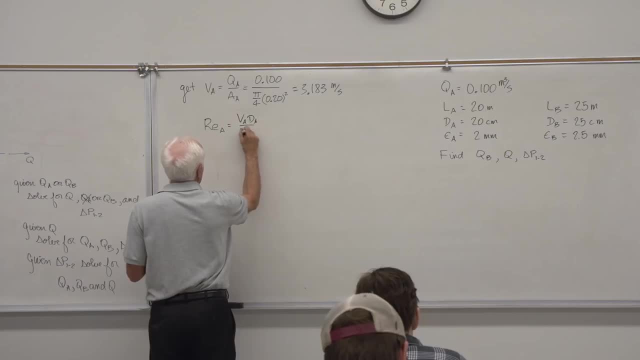 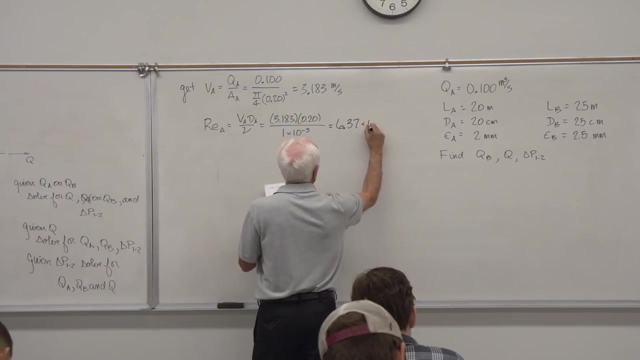 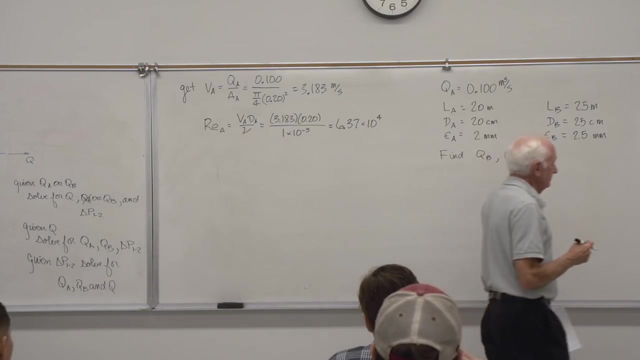 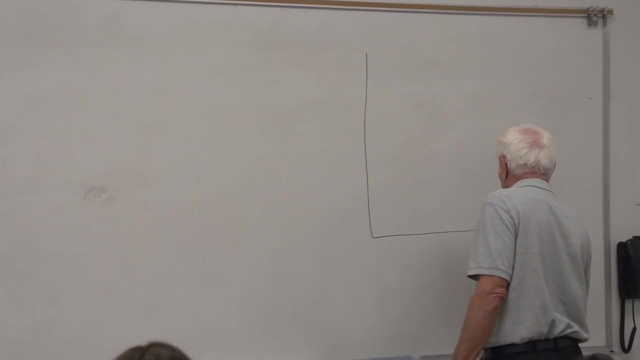 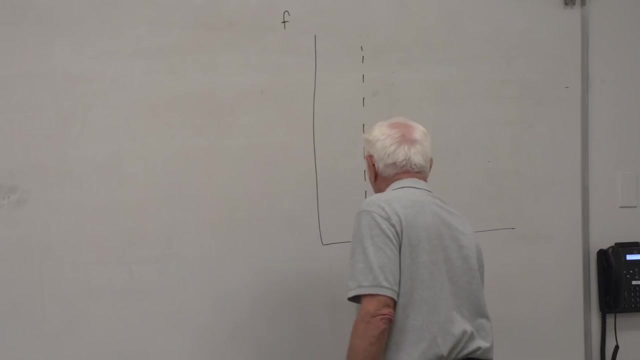 over nu Velocity Divided by pi over 4.. Diameter: Kinematic viscosity: Reynolds number: 6.37 times 10 to the fourth. Okay, got it. I go to the Moody chart. I've got different curves. We looked at these last. 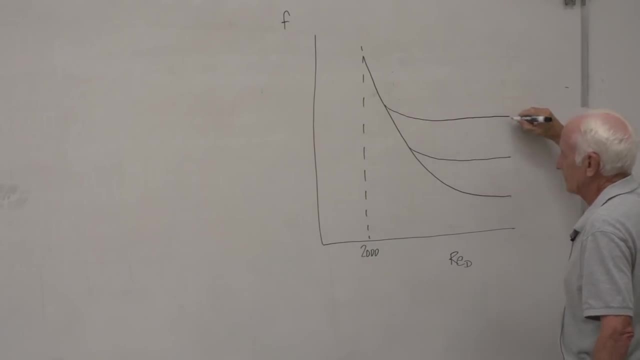 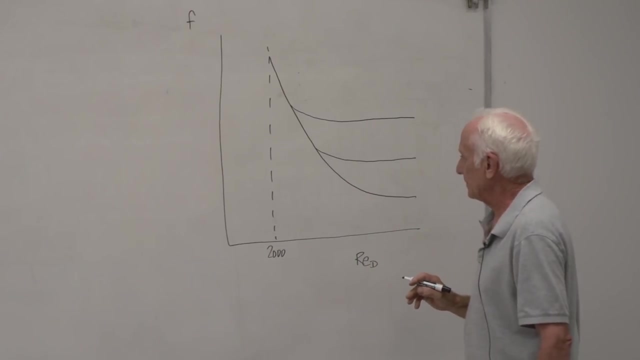 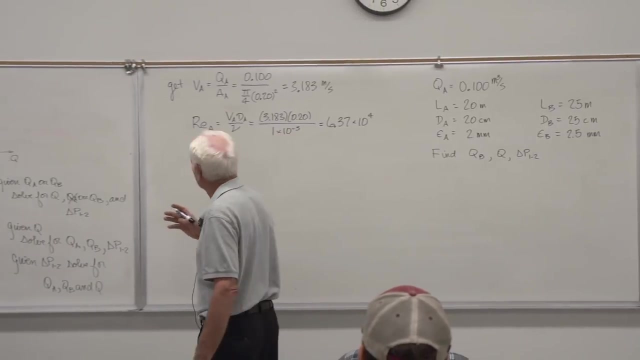 time I gave you a copy of a Moody chart to look at, rather than the textbook, so if you want to, if you missed it last time, I've got a copy of the Moody chart for you. I want to find F for pipe A. okay, Review of the first fluids, fluids one class I. 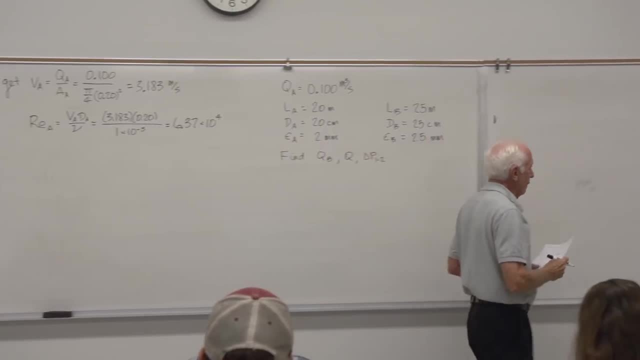 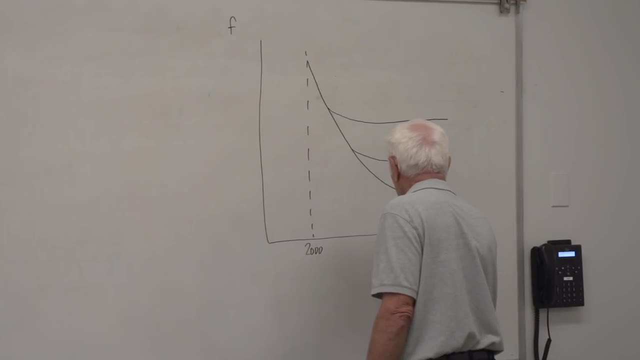 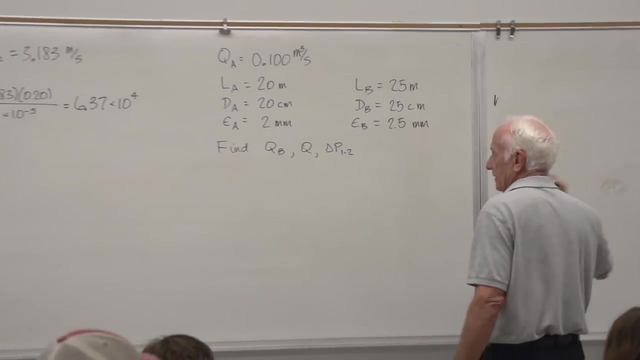 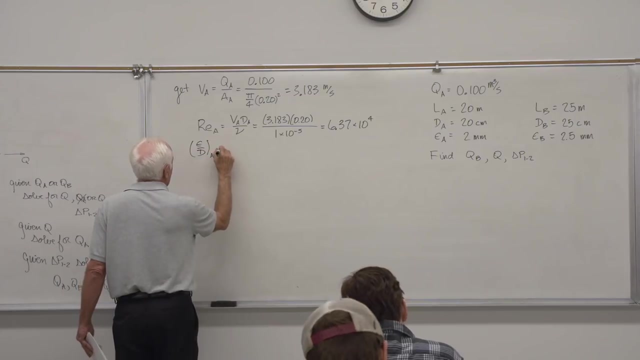 go to the Reynolds number 6.4 times 10 to the fourth. I have to go up to the relative roughness curve E over D, So E over D of pipe A. I'm going to go to the relative roughness curve E over D of pipe A. 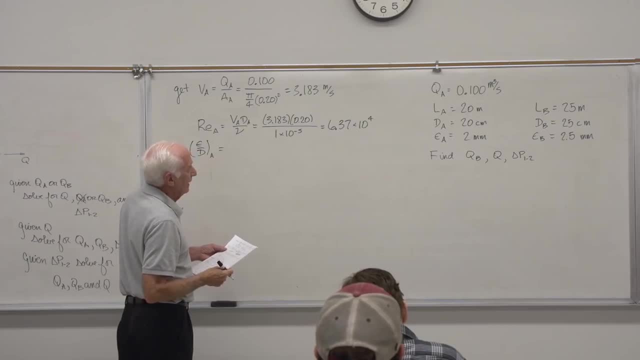 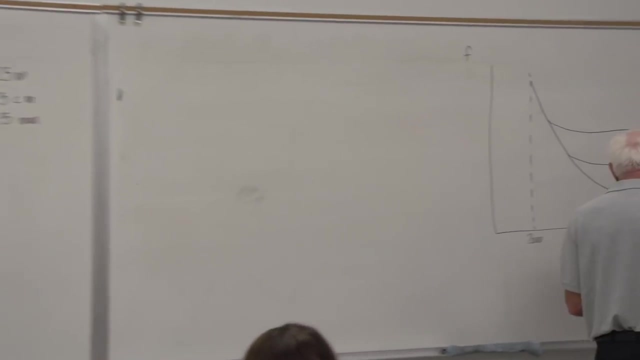 Okay, epsilon 2 millimeters. yeah, Diameter 200 millimeters: 2 divided by 200, 0.010.. I go here to that line, 0.010.. It's labeled like that on the Moody chart. you've got a. 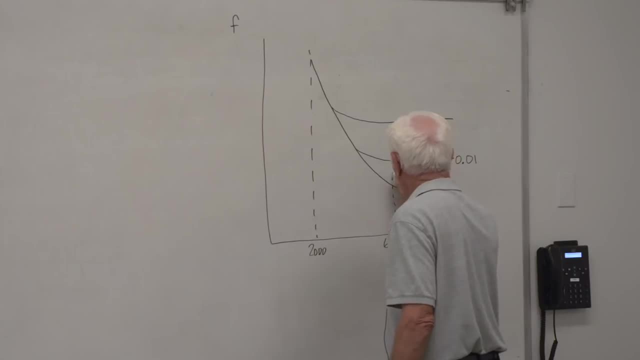 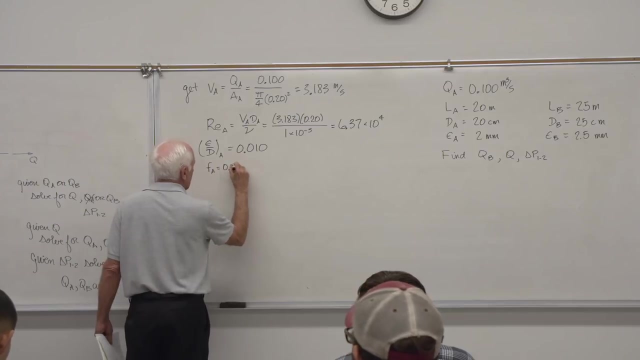 copy of. I go up here. I read across horizontally until I get the value of F of A: 0.038.. I didn't guess it, I got it exactly. Okay. F of A. Okay, Now as far as the. 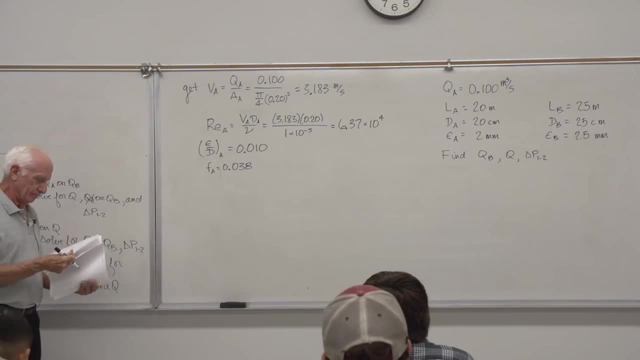 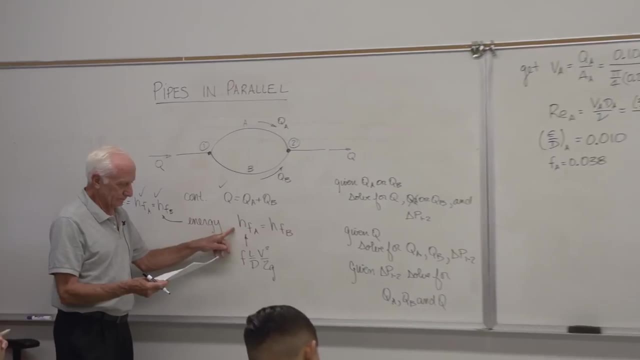 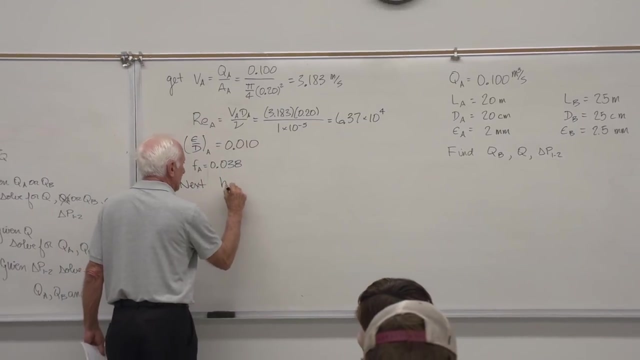 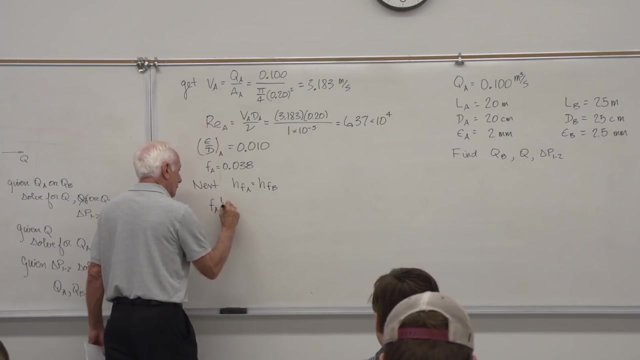 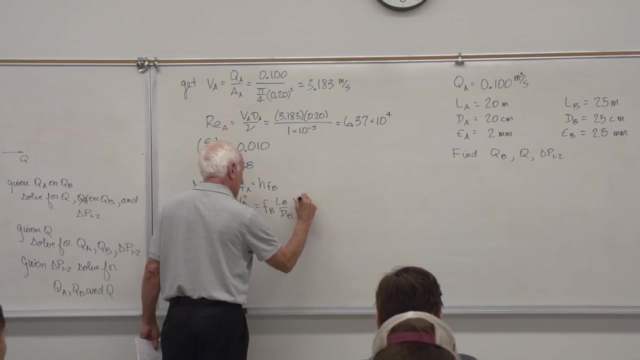 After that, let's see my next step. Let's look over. here. I'm going to use him next. HFA has to be equal to HFB because they're in parallel. There it is written up, the Darcy-Weissbach equation. 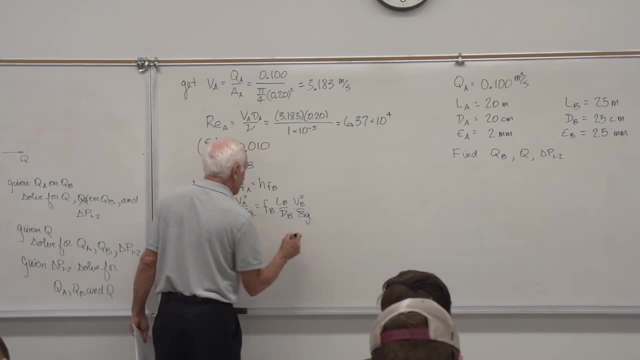 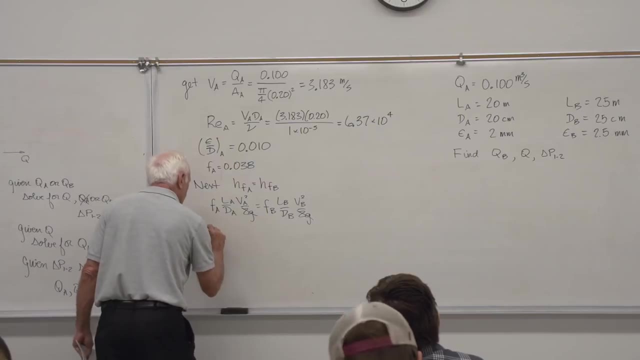 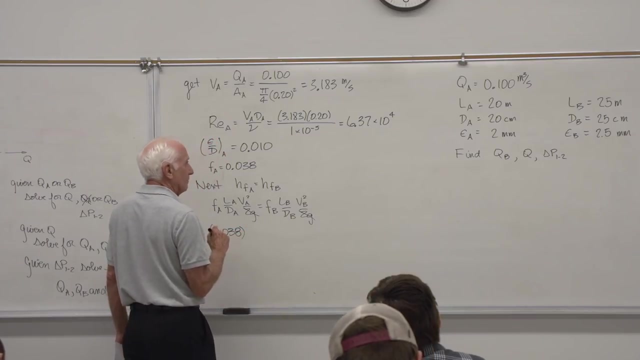 I'm going to cancel out the 2G. I'm going to cancel out the 2G. So I know FA 0.038.. LA 20 over DA 0.2.. VA squared. I know VA- VA 3.183.. 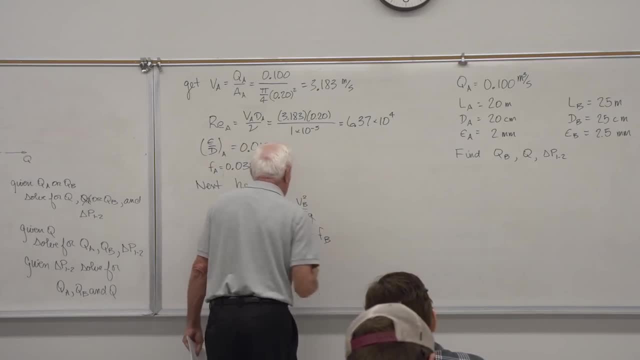 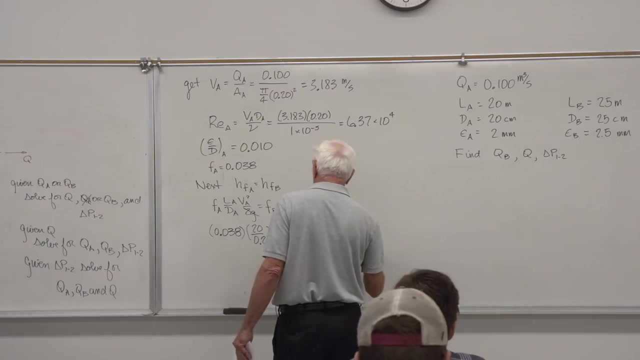 Equal FB. I don't know FB. LB 25 divided by 0.25.. Okay, Times my velocity in pipe. This is pipe B squared. Yeah. Okay, That's for pipe B. One equation, two unknowns. 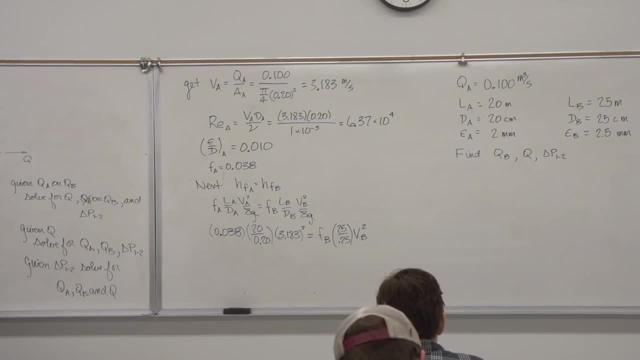 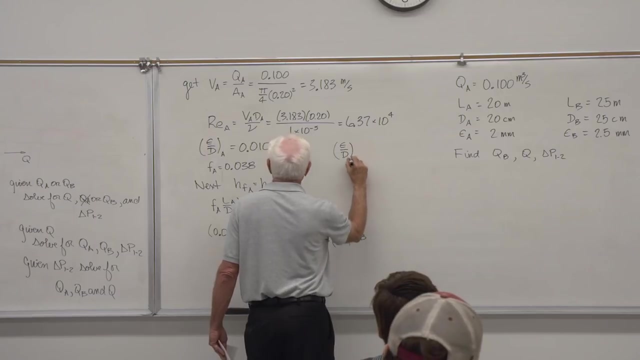 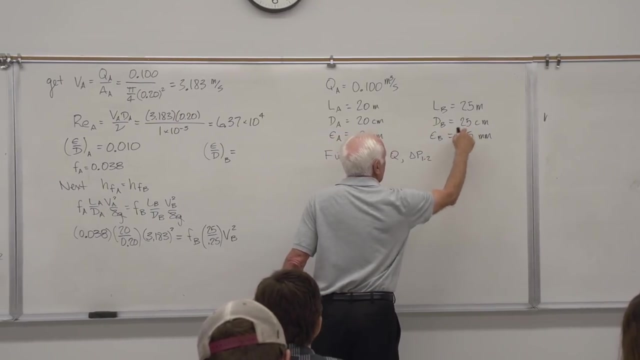 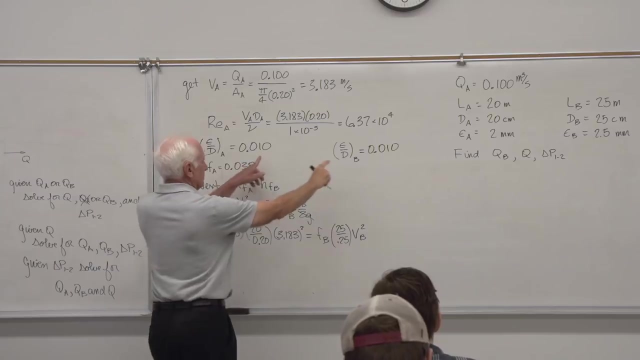 Okay, start the guessing game. Okay, I don't. I've got to find a guess for FB. there's a moody chart. First I'm going to get the relative roughness of pipe B, epsilon over D of pipe B, 2.5 millimeters divided by 250 millimeters: 0.010.. Notice: 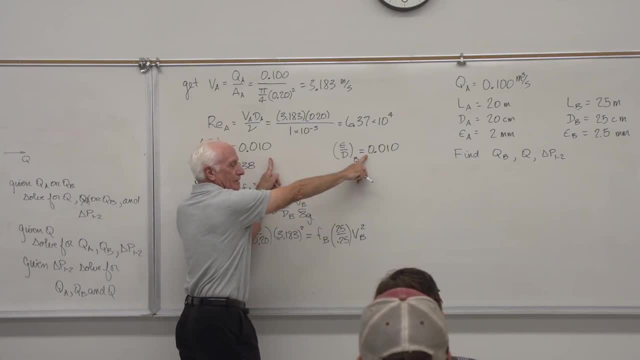 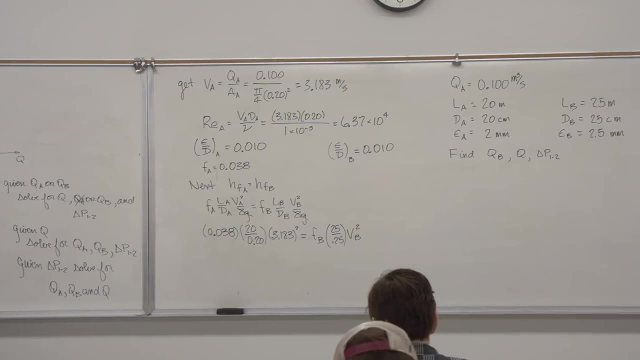 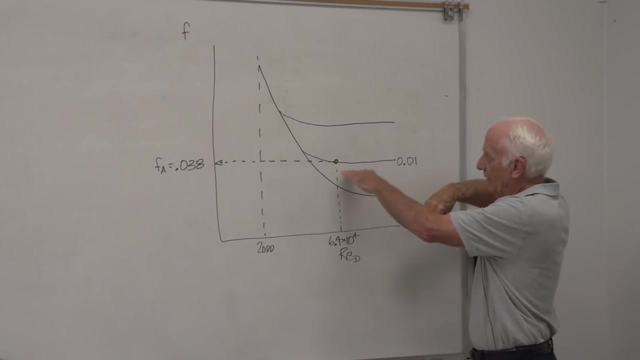 they're the same. epsilon over D, epsilon over D is the same. I don't know. I don't know the Reynolds number, obviously. So what I normally would do would be go over to the moody chart, take a ruler, lay the ruler down where the flat part. 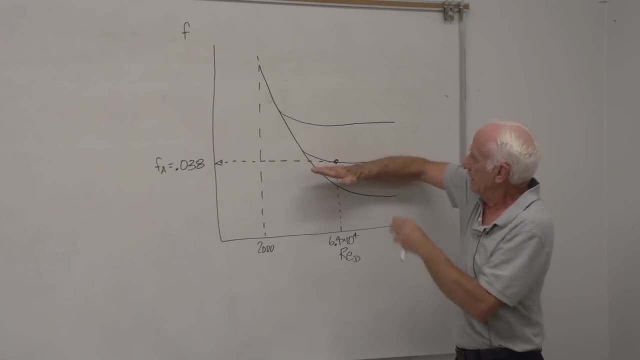 of the curve is horizontal part. Extend that ruler to the F axis and take that as my first F guess. Well, it turns out it's pretty close to this. If you put a ruler on this line right here, you can do it yourself with what I gave you. 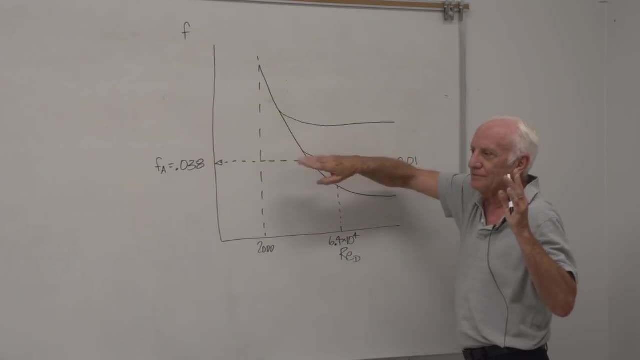 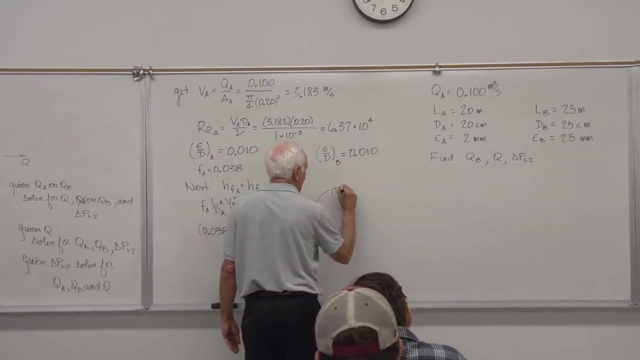 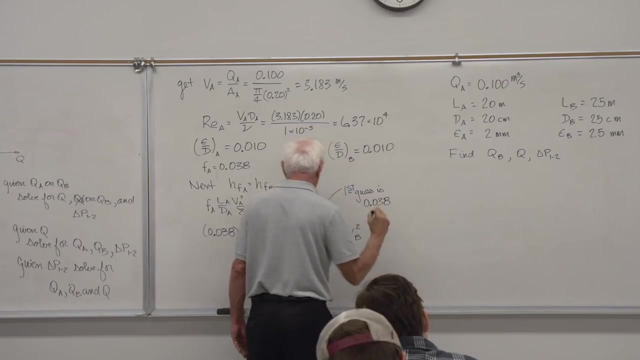 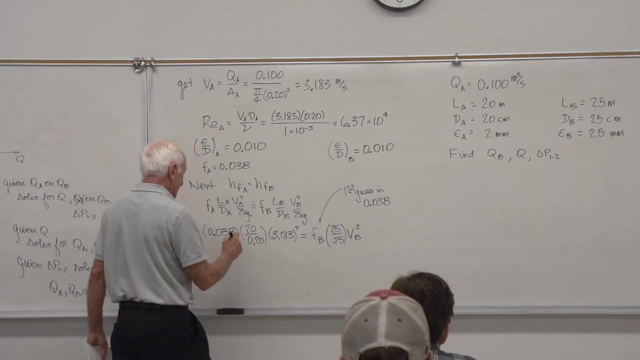 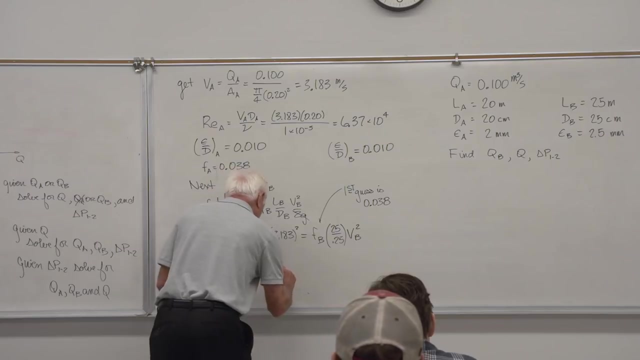 It's really close to that. So I'm going to say my first guess for FA is 0.038, FB, pardon me, First guess is 0.038.. Got it Okay. Solve for VB. I get VB equal 3.183.. That's interesting. the same as VA. same. 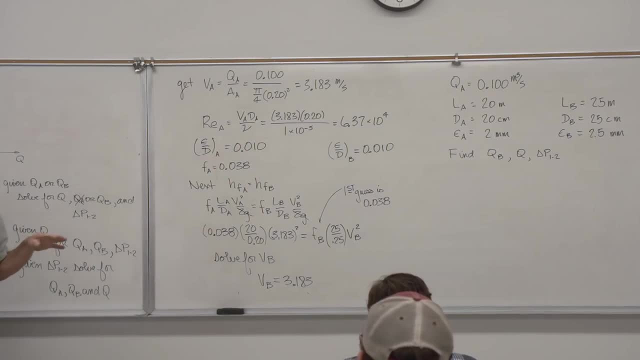 velocity in both pipes. You wouldn't know that It's not normally true, But I made this problem up so the numbers were really simple. I didn't want to hide things by, so I made these timers up so everything kind of came out the way it. 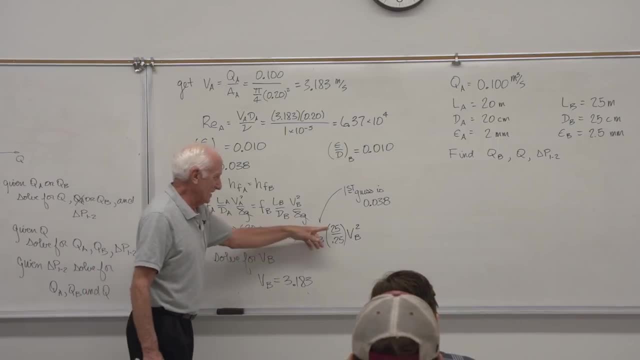 cancels out. 20 divided by this is equal to 25 divided by that. This was equal to that. Okay, I did it on purpose to make life easy, Okay, But okay, So that's okay, It can happen. There it is. Is that what I want? QB? No, no, It's not QB yet. 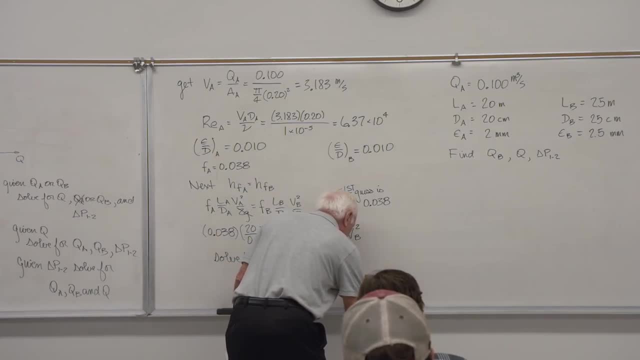 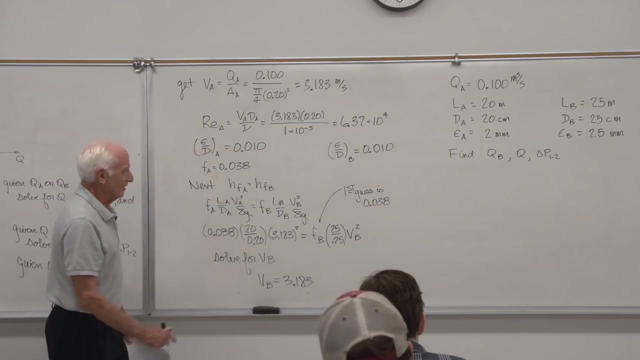 Don't forget QB. QB equal VB times area in B. Well, okay, We'll do it the right way. We'll do it the right way. I don't know if that's right or not. Why? Because I guessed it. I've got to check my guess. 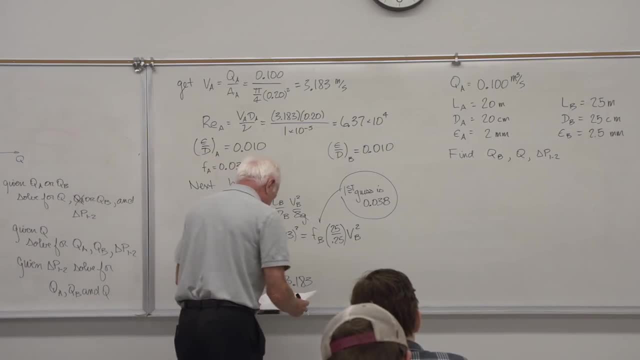 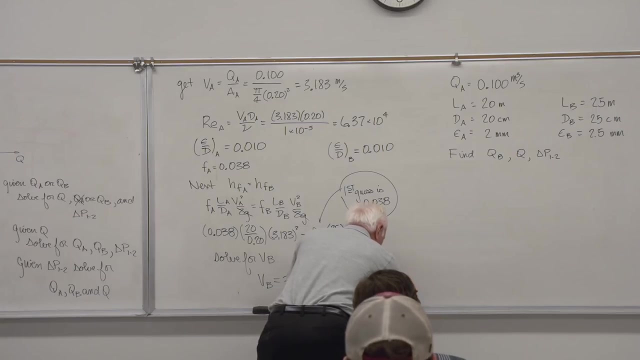 now. So there's VB. So now from that get the Reynolds number, pipe B, and you get Reynolds number for pipe B. Then take that velocity times the diameter divided by the kinematic viscosity- 7.96 times 10- to the fourth. So that's the. 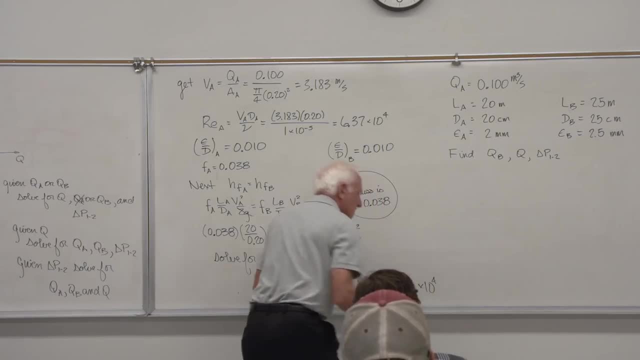 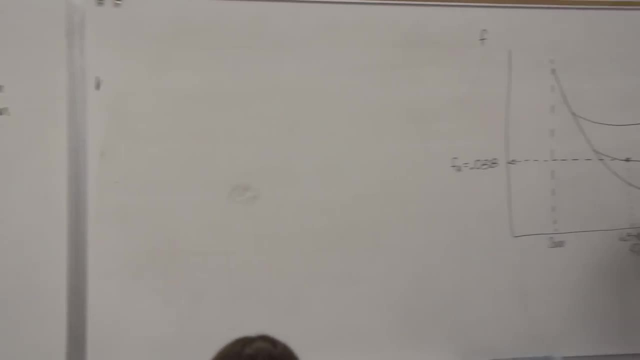 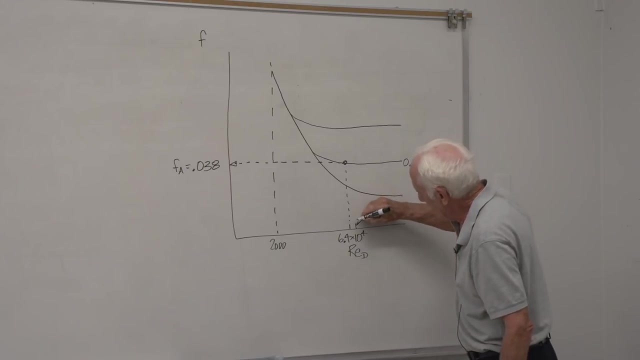 fourth: 7.96 times 10 to the fourth. Go back over to the Moody chart. Here it is 7.6 times 10 to the fourth. Go vertically up until you hit the relative roughness line labeled .01.. There it is. Go horizontally across. 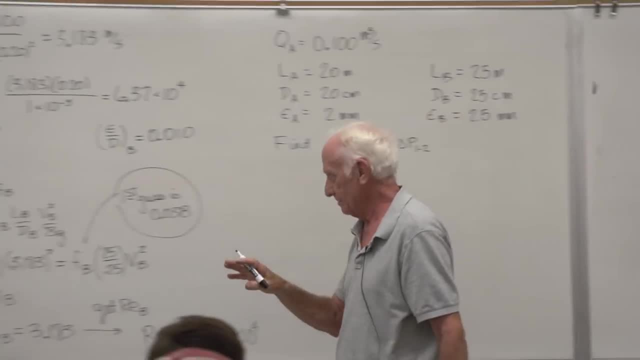 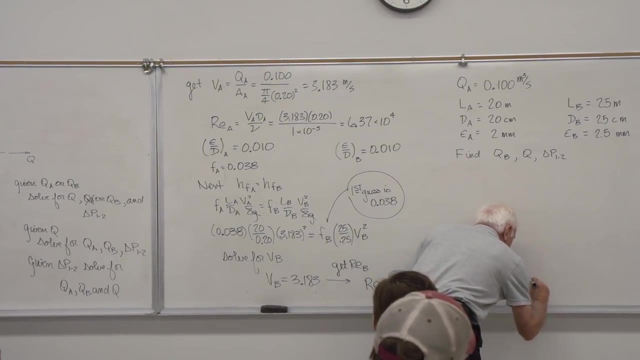 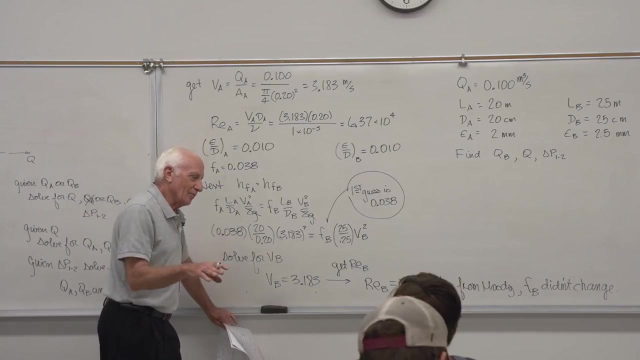 Thank you very much. It didn't change. It didn't change From Moody FB didn't change. So no more iteration. If it would have changed, and in this exam situation you just tell me, I would repeat the above calculations based on this. 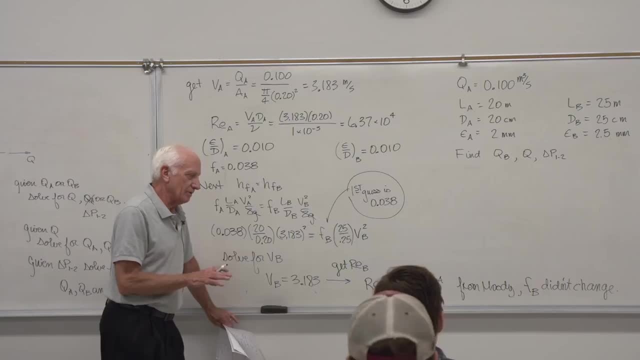 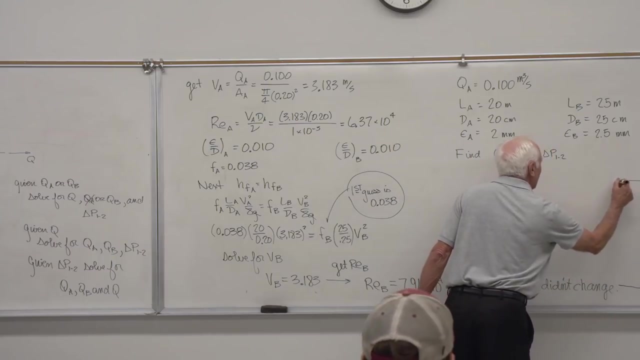 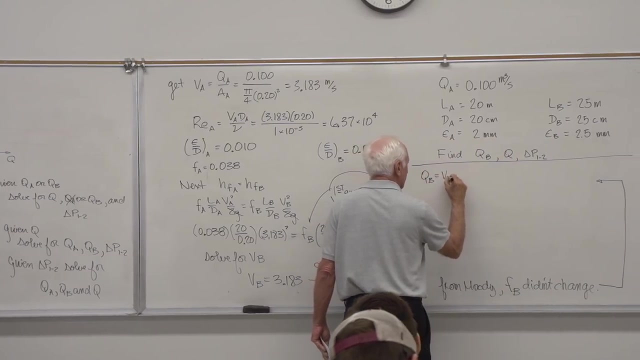 new FB until the FB value converged. That's all you say. so I know what you would do as a next step. In this case it converged immediately, Okay. So once I get this, okay, now I'm going to go, maybe up here Now. I'm going to get QB Now. I. 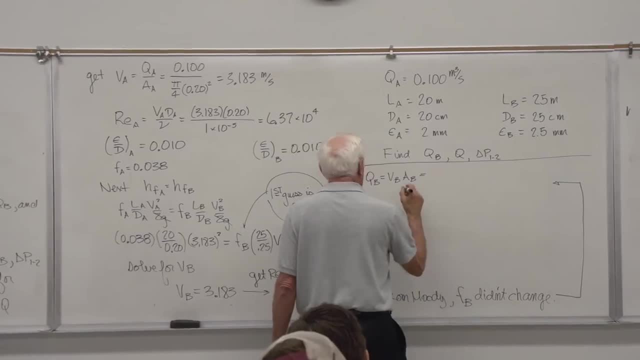 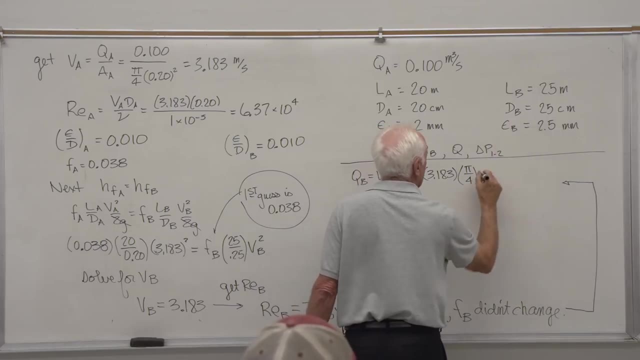 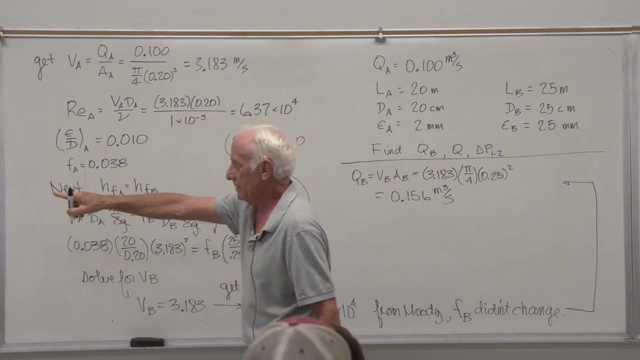 know that's the correct velocity: 3.183 times the area pi over 4, D squared .156.. So my QB: 0.156.. Okay, Now I want Q. There's the equation over there for Q. 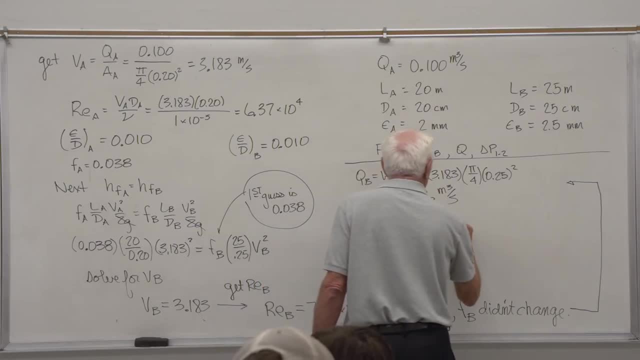 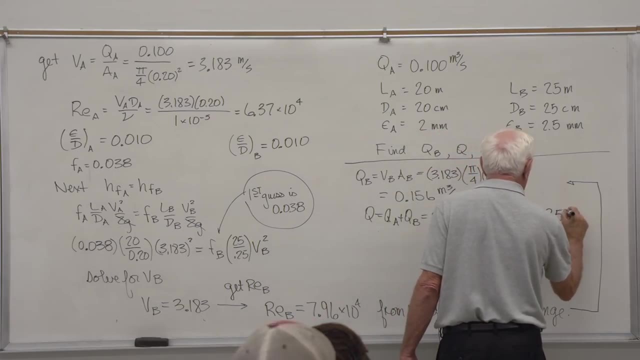 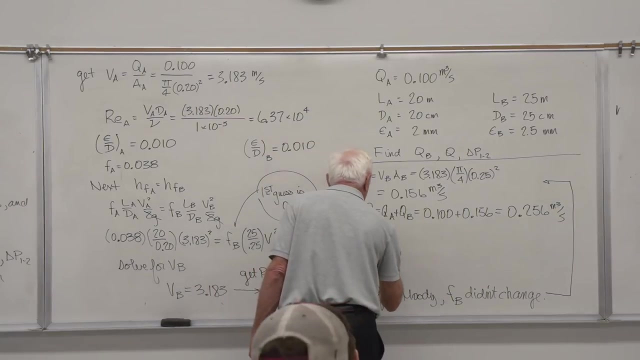 .156.. .156.. .156.. .156.. .156.. .156.. 1, 0, 0, 1, 5, 6.. Got it? The third question: what is delta P? There's the equation over. 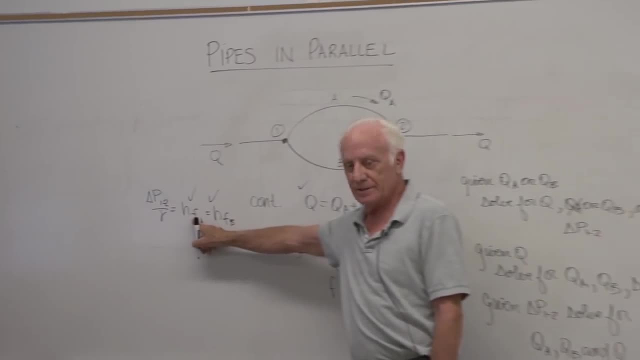 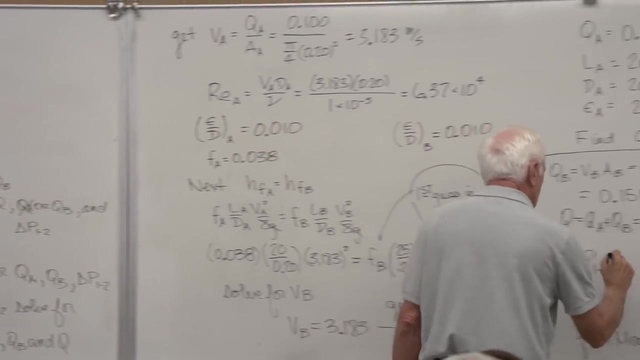 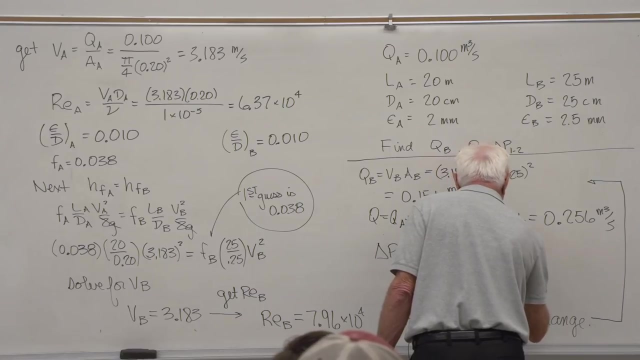 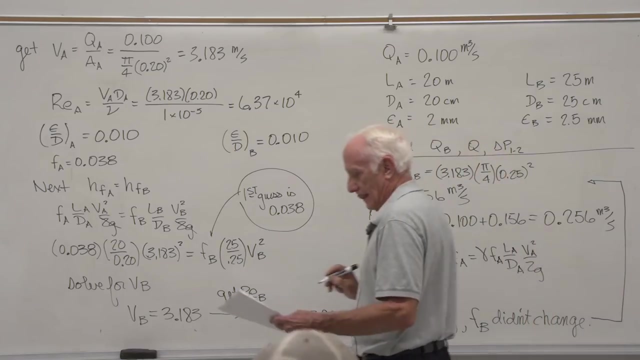 there, I wrote it down for you. Take your choice. take your choice: either HF1 or HF2. those are in parallel, So delta P is equal to gamma times HFA, gamma FL over D V squared over 2G Gamma 9810, so delta P comes out to be 19.25 kPa. 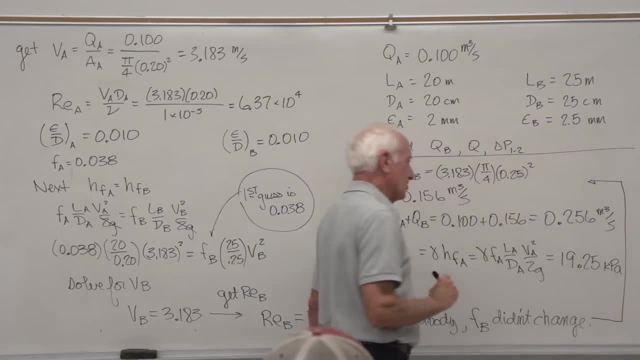 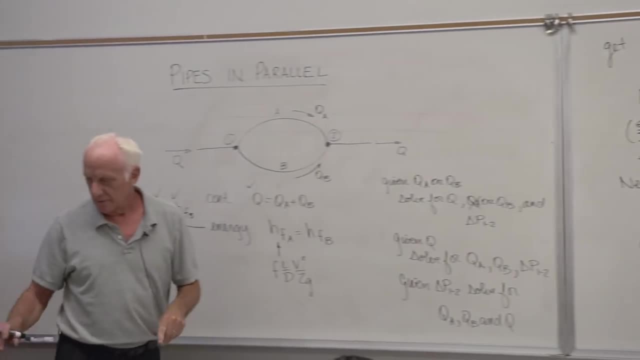 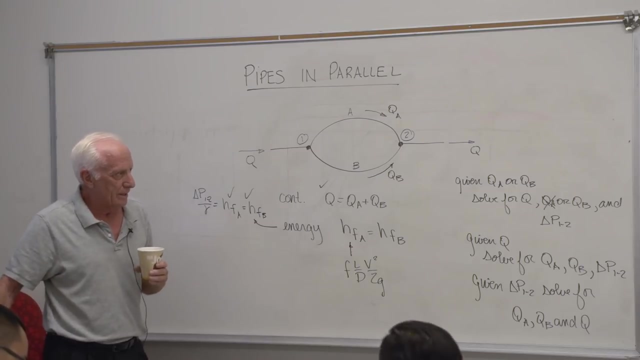 Pressure drop from point 1 to point 2 in this picture right here with those two pipes. So you do it the same way, no matter whether it's this problem or the problem with two reservoirs separated by a distance, delta Z. that's the way you. 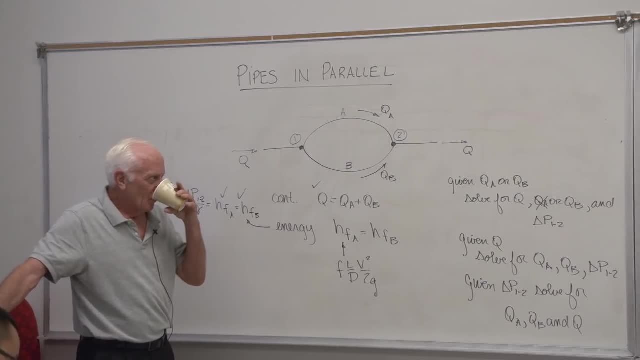 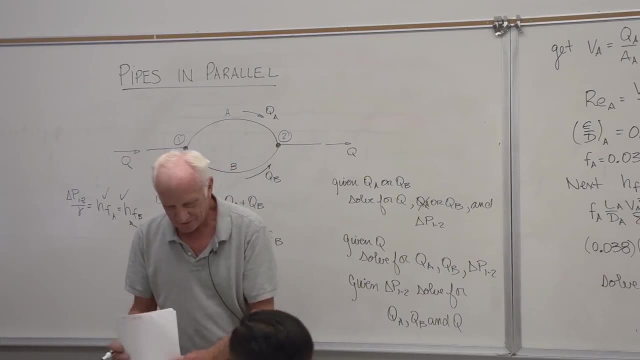 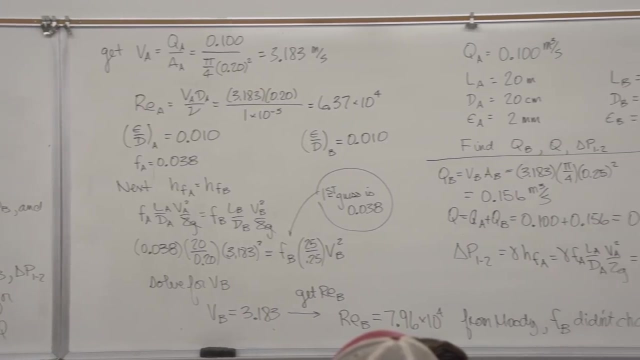 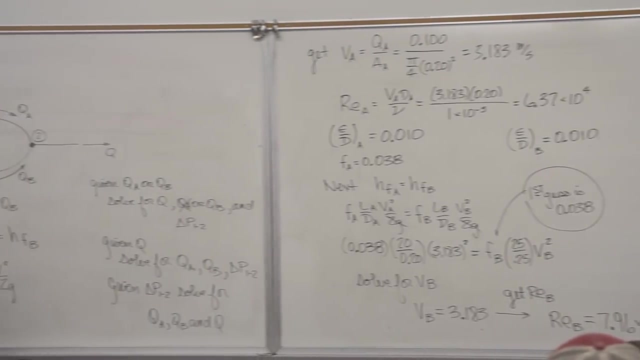 approach all these guys. Okay, now, any questions on that? then? Okay, Second step: this is the last part of the chapter six material. last part of chapter six material. Let's start over here. Pipes in series. pipes in parallel. 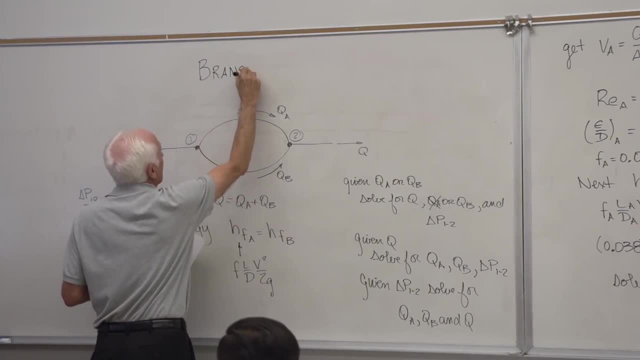 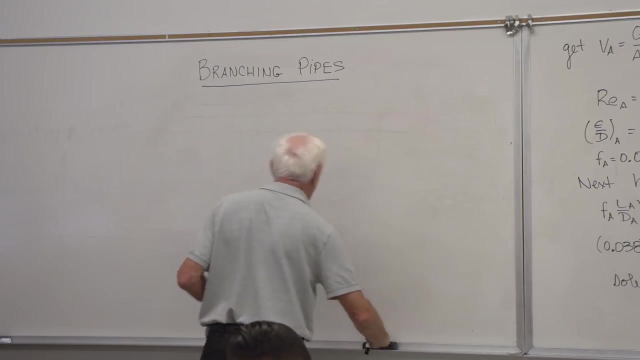 and now branching pipes. Okay, Here's what I'm going to do. I'm going to do a branching problem. Okay, Here's what a branching problem looks like. Let's take three reservoirs. This one will be reservoir C: This one will be. 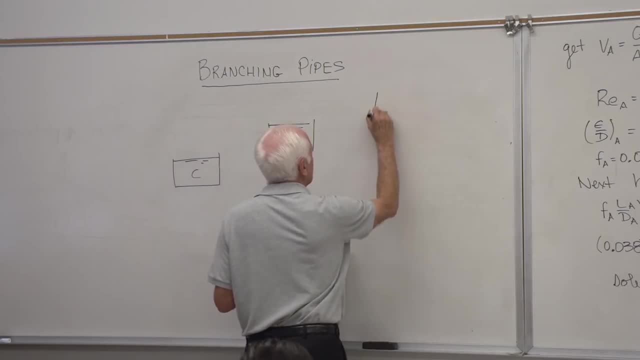 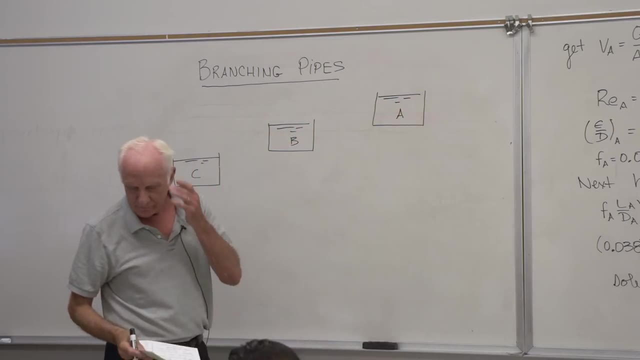 reservoir B And this one will be reservoir A. Okay, And they're connected by pipes. So this guy down to here, this guy down to here, this guy down to here. We call this point. J stands for junction. That's the junction point. 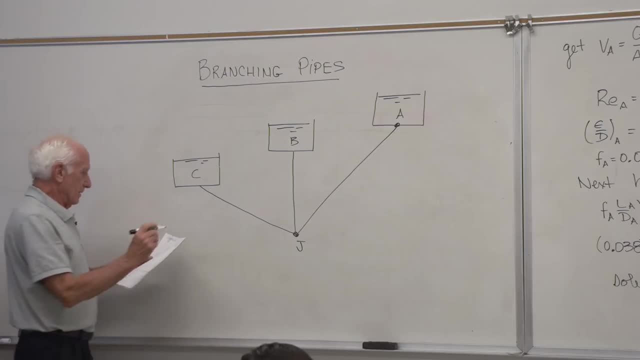 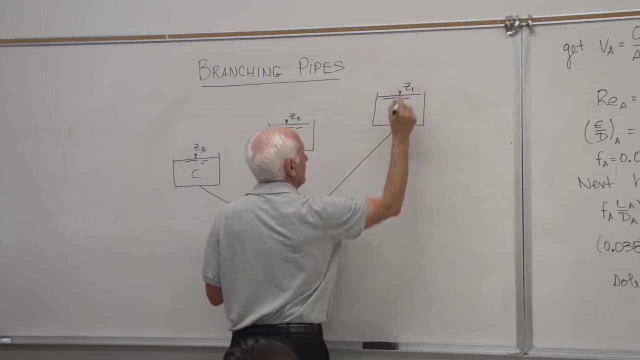 This elevation we're going to call Z3.. This elevation, Z2.. This elevation we'll call Z1.. Typically we know the elevation Z1, Z2, and Z3. And the question that is asked is: what are the flow rates in those three pipes? Okay, This is pipe A, This is. 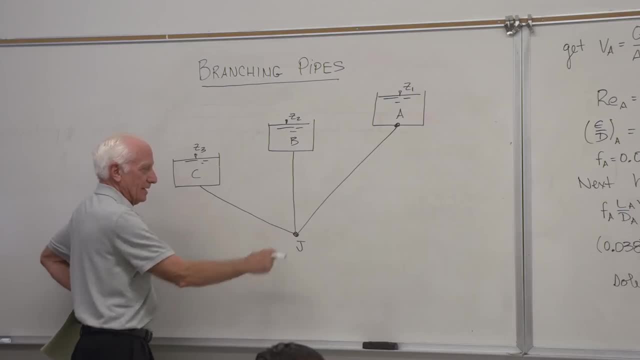 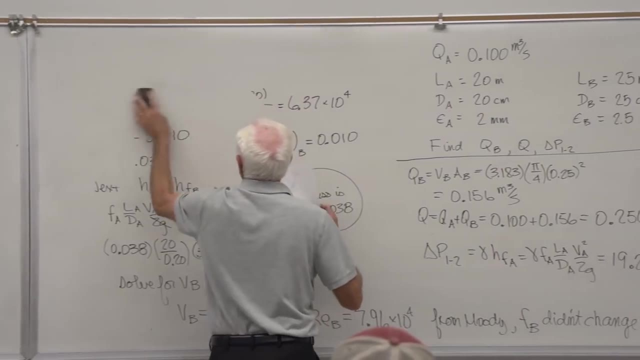 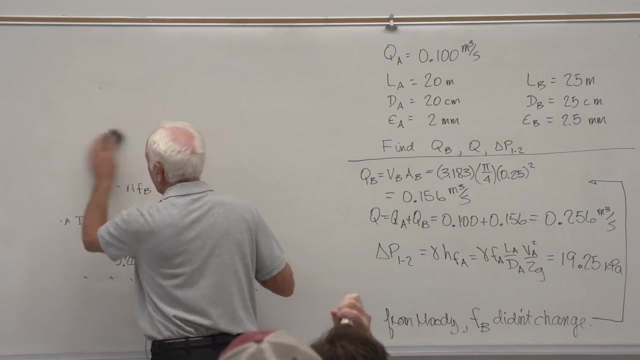 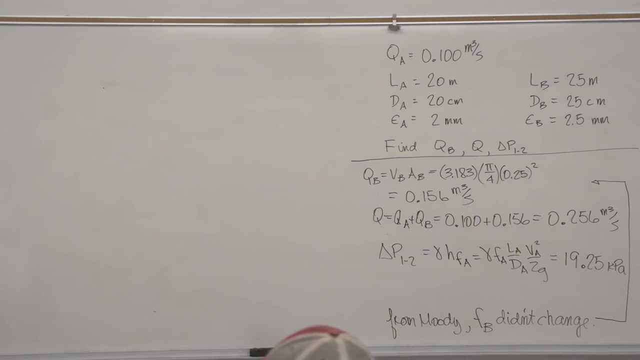 pipe B. This is pipe C. They come together at J. Okay, So we write our equations And we start off. we'll start off with Z1, Z2, and Z3.. Okay, So we start off with pipe. Let's do pipe, I guess this one first. A to J, So energy. 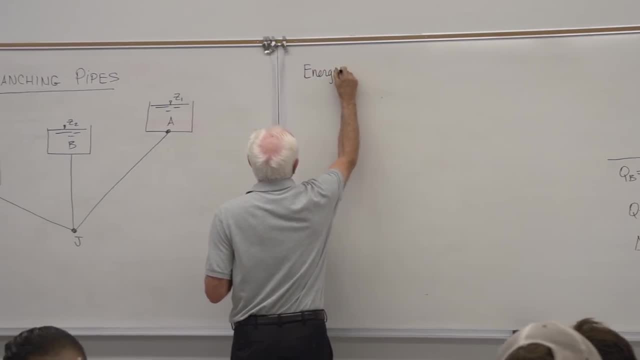 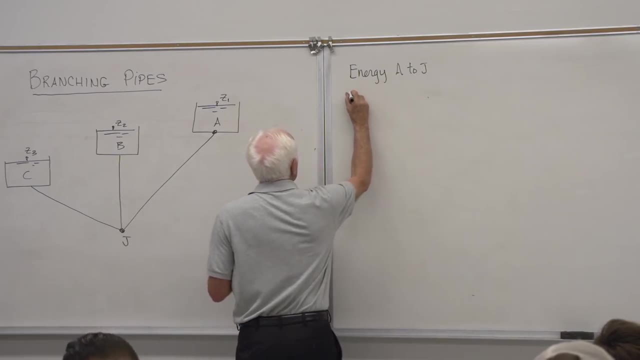 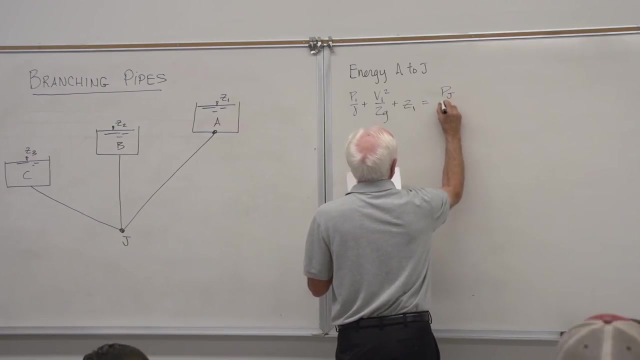 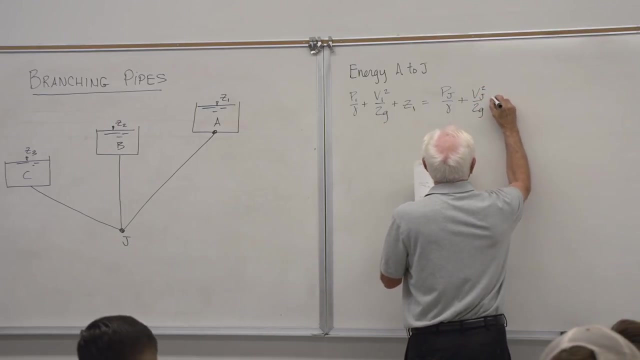 A to J. Okay. Energy equation: P1 over gamma V1 squared over 2G, Z1 squared over 2G. Okay, Z1 equal P at J, V at J squared over 2G ZJ, plus the friction loss H in that. 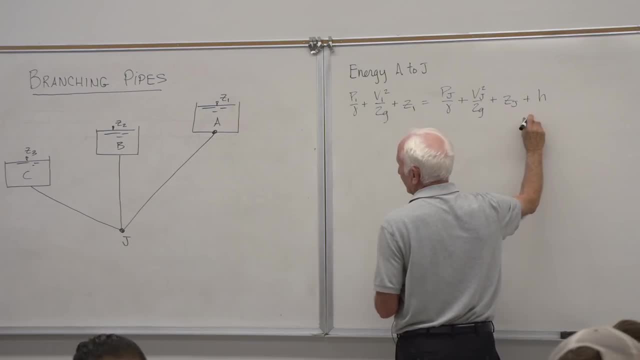 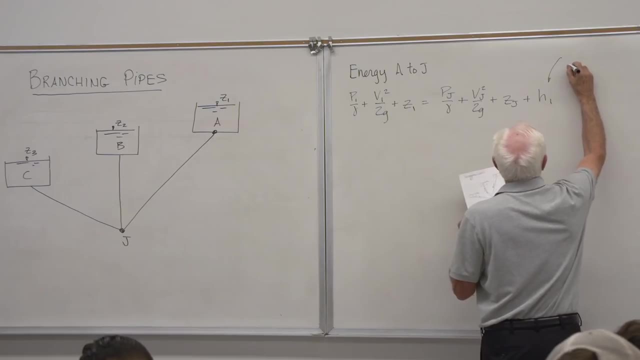 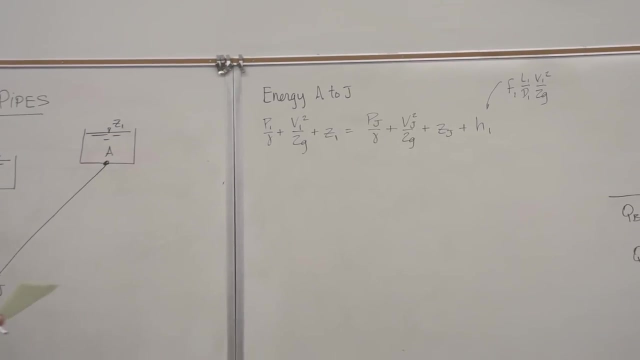 particular pipe, I think I guess I call that. I don't know why I did that, but okay, I call that H1.. Okay, That's in pipe A. That's the friction loss in that pipe right there, Okay, Free. 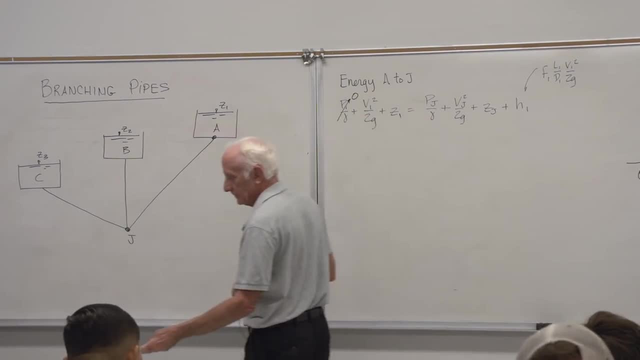 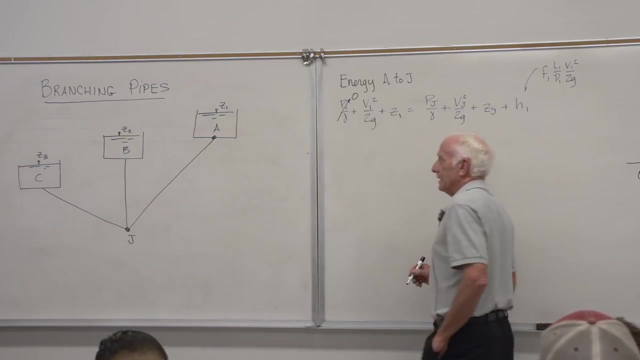 surface: P1, zero gauge, Pressure: zero. We talked about this before- from pipes in series in parallel. Normally the textbook, if you read it, says we're going to neglect the difference in kinetic energy. We know V1 is zero. Get rid of that. 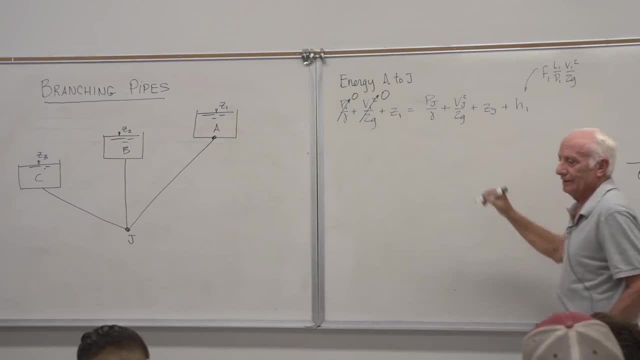 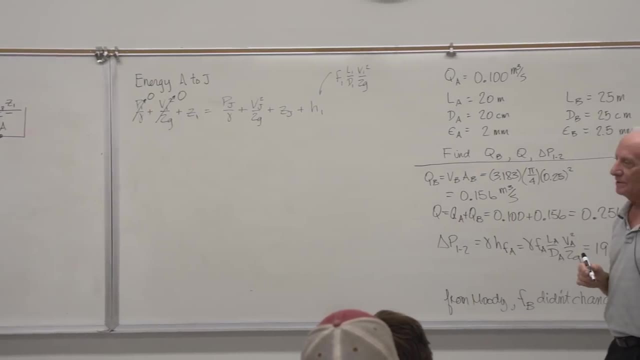 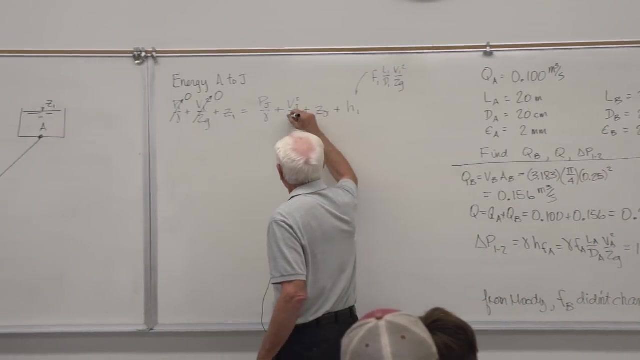 guy. We're going to neglect that guy right there because he's typically a lot smaller than any other term in the equation. Okay, So I'll believe him. textbook says We typically neglect that term because this value is a lot smaller than the other terms in the equation. Okay, We neglect him. 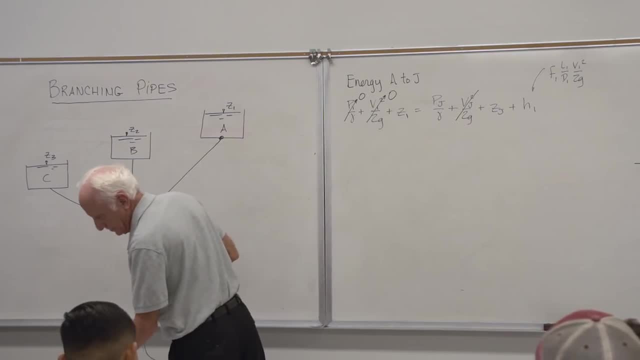 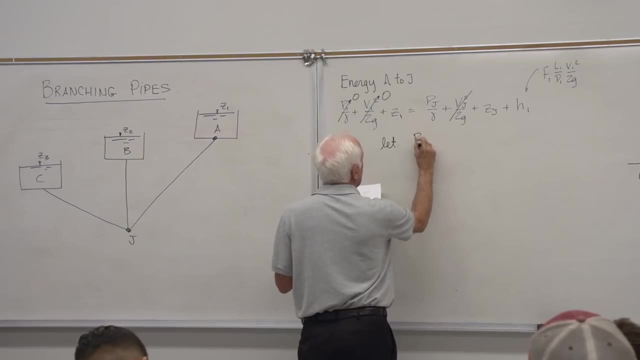 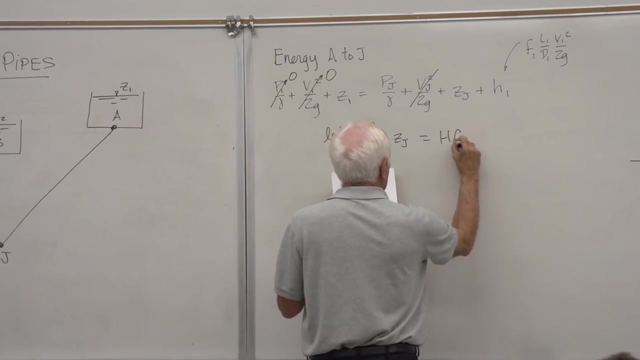 Okay, So we're left with our first energy equation. So we have- and we're going to let change this to be let PJ over gamma plus ZJ equal hydraulic grade line at J. Okay, Okay, Okay, Okay. 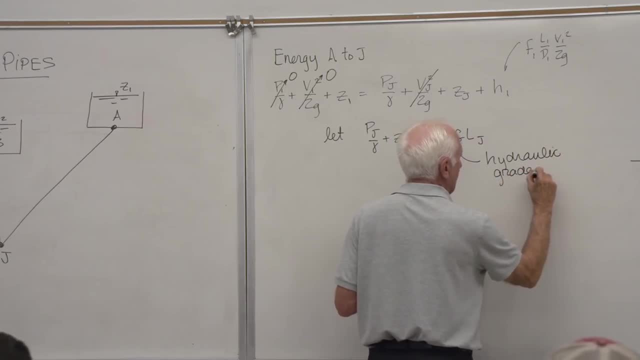 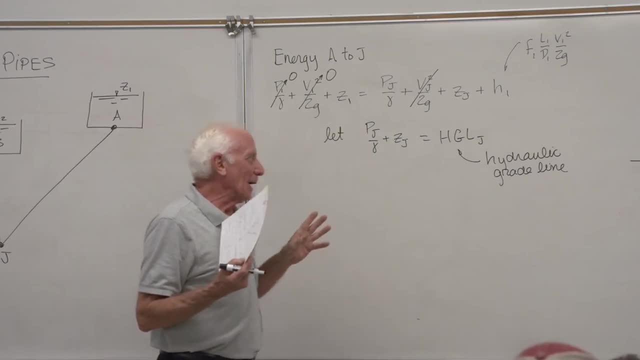 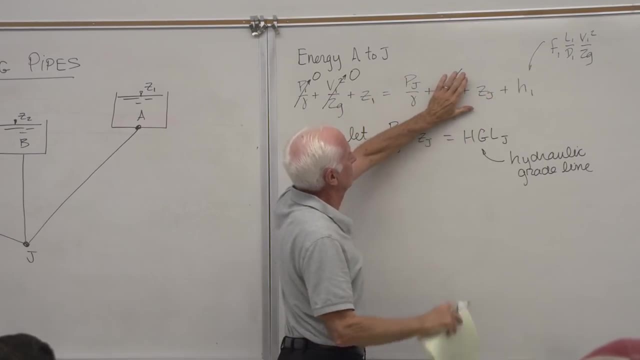 Yeah, It depends who you have and how much time they have. That's okay. That's okay. Just so you know these three terms together. that's called the eventually grade line. If you knock them out, those two terms are called the hydraulic grade line. 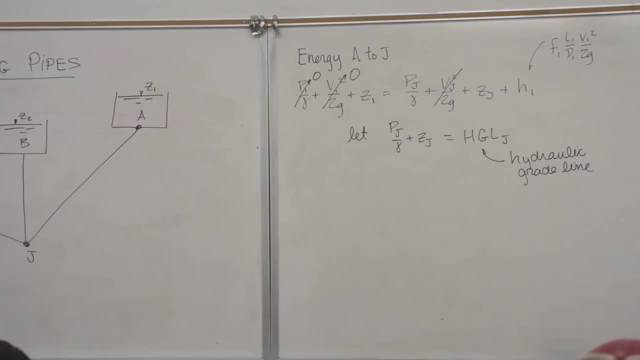 Exactly used a lot in civil engineering. They really beat it into you there. Maybe not so much in mechanical. It has some interesting uses, graphically especially. But that's okay, Don't worry about if you haven't been exposed to it. All you know is that when you add these: 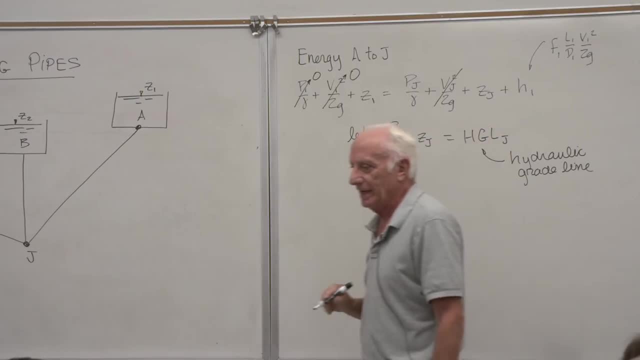 two terms together. they're titled hydraulic grade line HGL. Okay, That's energy A to J. We do the same thing, Energy B to J- And we get this equation. Oh, by the way, I didn't complete this. Let me complete this first Replace. 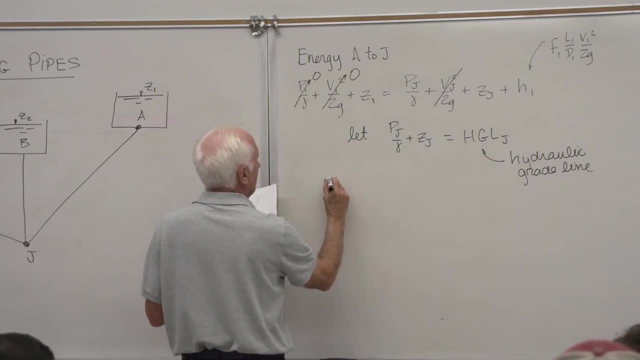 these two guys with that. So we get Z1- equal hydraulic grade line at J plus H1.. Now we go Energy B to J. Okay, I'm not going to go through all the gory details again. We get this one Z2- equal hydraulic grade line at J plus H2.. And then we go. 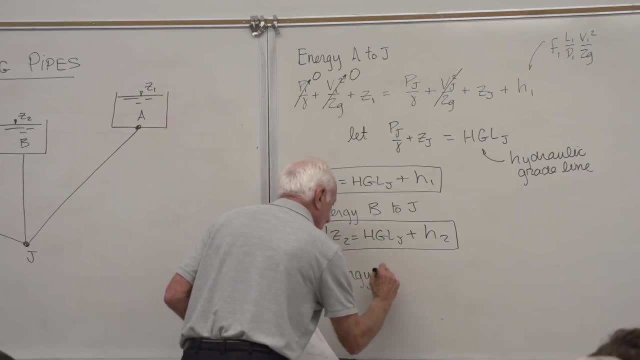 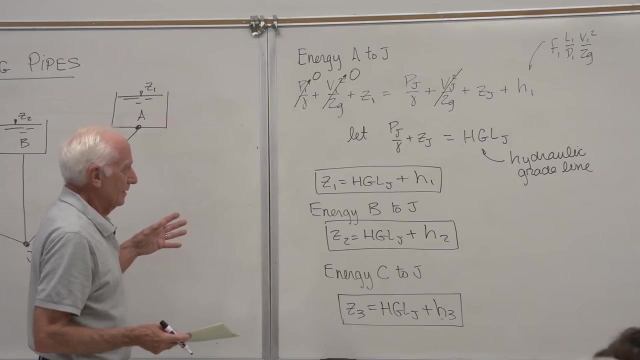 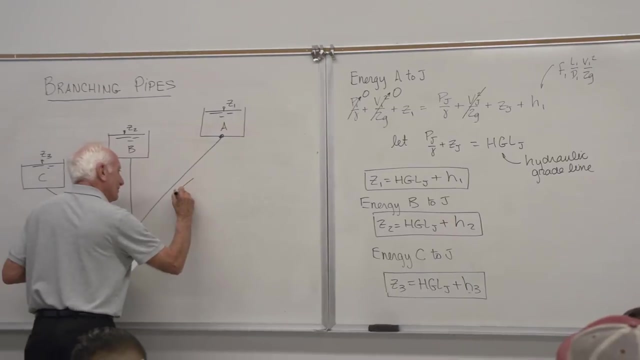 Energy C to J, Z3.. Okay, When we write that energy equation, those three energy equations, this is not right. We know we're wrong, But this is. this is the way We're assuming the flow rate is going down here, going down here and going down here. 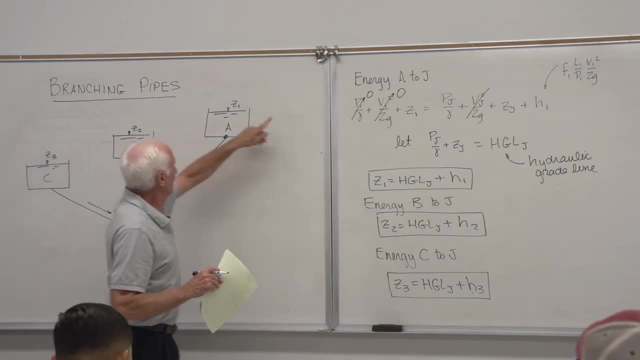 Every one of these start out up here, down to J, Up at 2, down to J, up at 3, down to J. That's a three boxed equations. We know they're wrong, We'll correct them later, But for right now we don't know which way all these flow rates go. 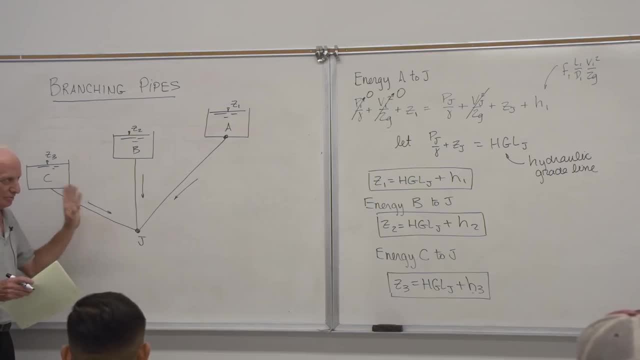 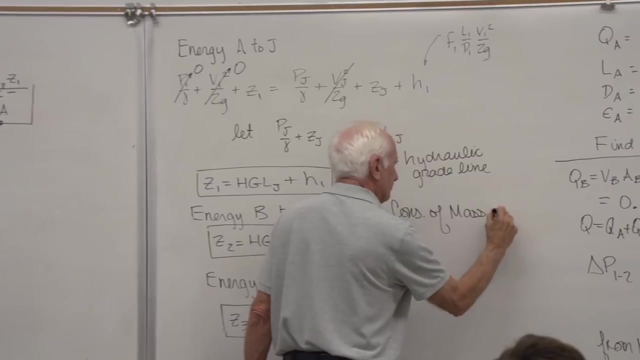 I do know some, but I don't know some other ones. when I worked a problem, an example I'll show you, but that's assuming all these flow rates go down, which we know can't happen. Okay, the last equation: conservation of mass. at J, The flow rates that come in. 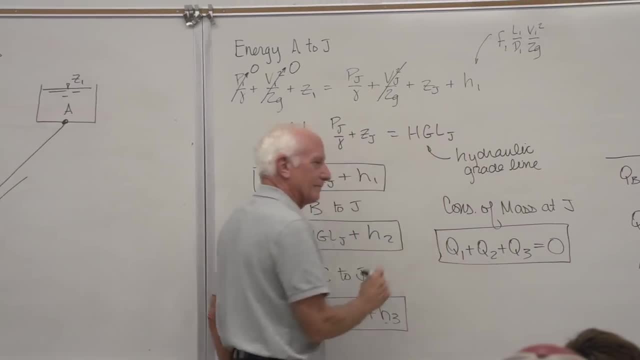 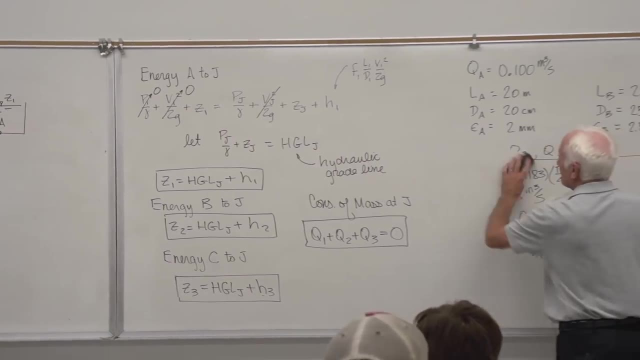 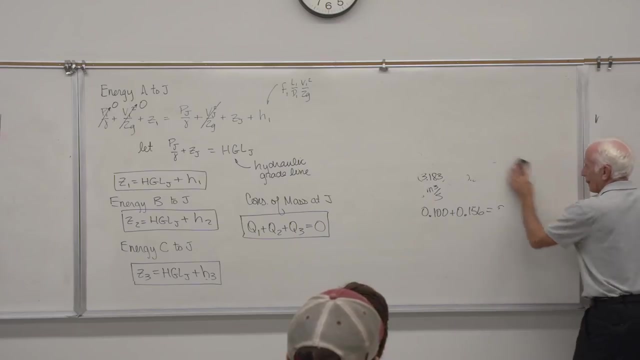 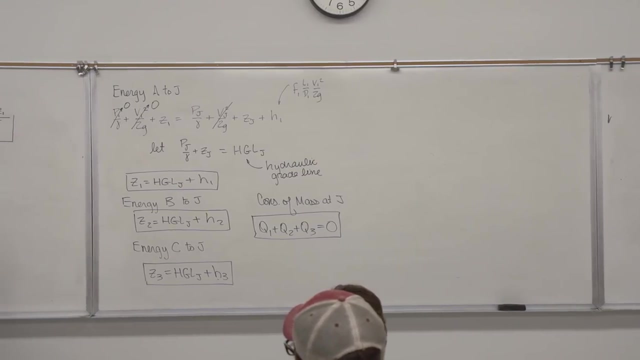 Equals zero got it. three energies, one conservation of mass. Okay, We can have four unknowns. okay, three equations. I'm a four equations. we got four unknowns. You probably know what they are. Here's q1, q2, q3. There's three of them. 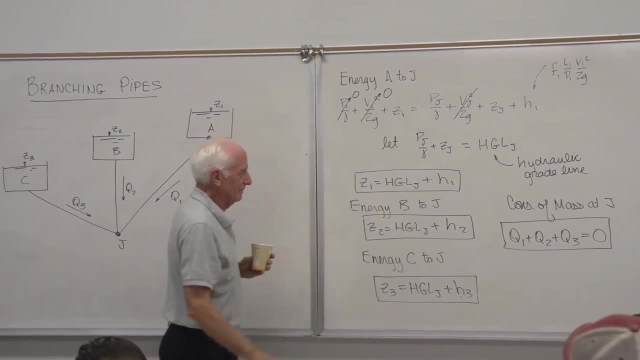 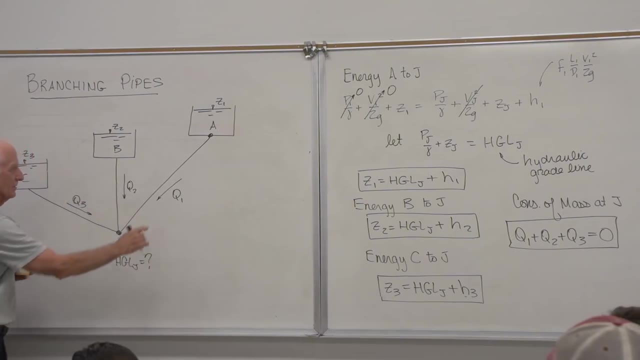 The other guy. I don't know the pressure: J. hydraulic rate line J, Four unknowns: q1, q2, q3. hydraulic rate line J, four equations: Theoretically I can solve those algebraic equations Okay, so that that's the approach you use. Now we'll work a. 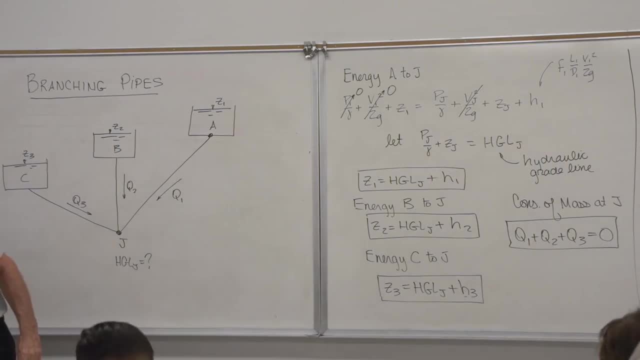 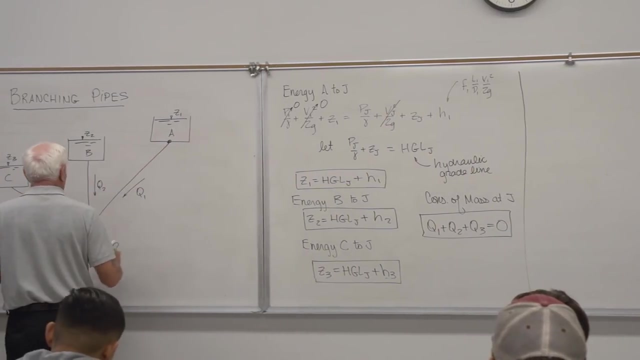 Problem with numbers, to see how that cranks out. Okay, so let's start off, and I'm gonna maybe leave this same picture up here. Yeah, I'm just gonna change some things here. Okay, I'm gonna get rid of this. Okay, I'm gonna get rid of this. I'm gonna start with just how the problems pose to you. 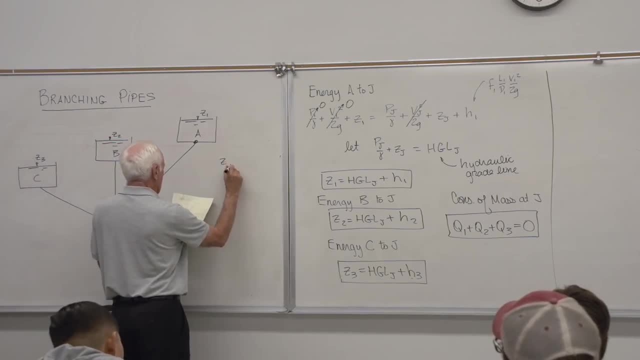 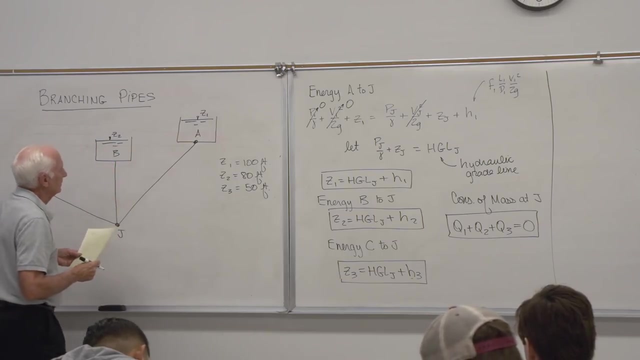 Here it is: Z 1 equal to- I'll do an English problem- hundred feet. Z 2 equal 80 feet. Z 3 equal 50 feet. Okay, let's see pipe. Okay, This was call this pipe one. I hate to call it pipe AJ, it makes it too complex. 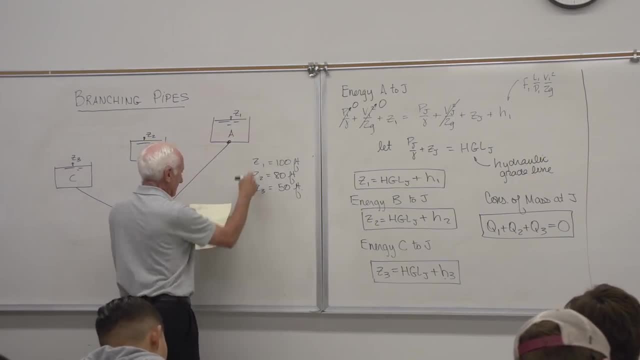 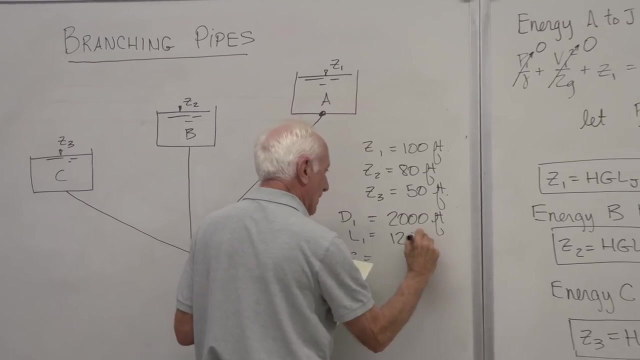 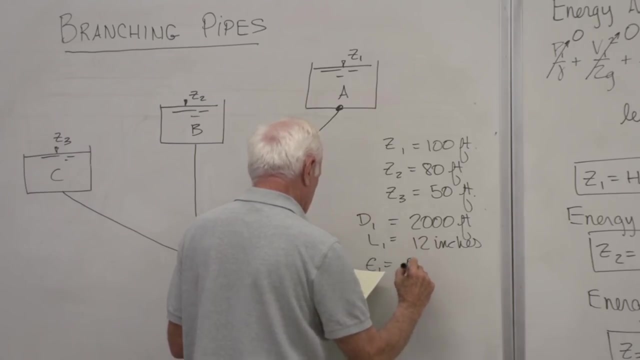 I'm gonna call that pipe one. Oh yeah, that's okay. That's fine, pipe one. D 1, L 1, Epsilon 1. Hmm, I'm copying the wrong line. that is a 8 inch pipe and Epsilon 1. Okay, D 2, L 2, Epsilon 2. 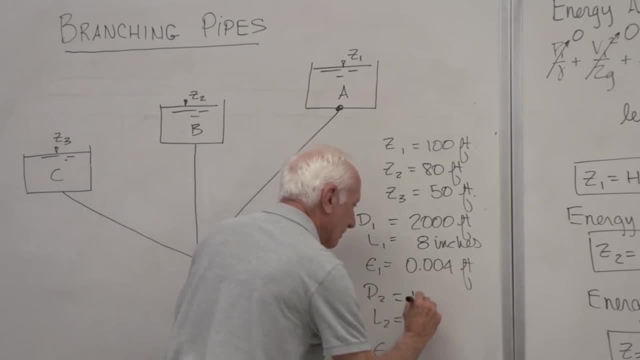 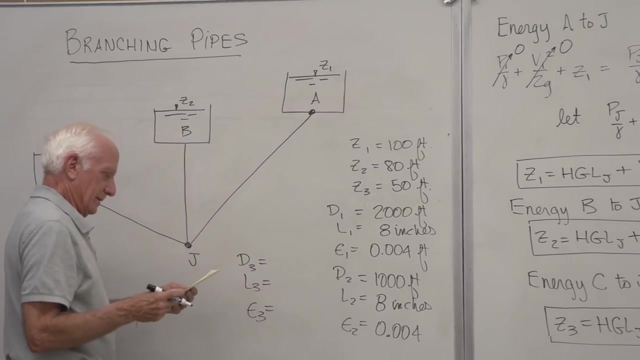 Okay, D 2: a thousand foot long pipe. It's 8 inches in diameter. I The roughness of that pipe. It's the same, 0.004 feet. Okay, D 3, L 3, Epsilon 3: Pipe 3 is 2,000 feet long. 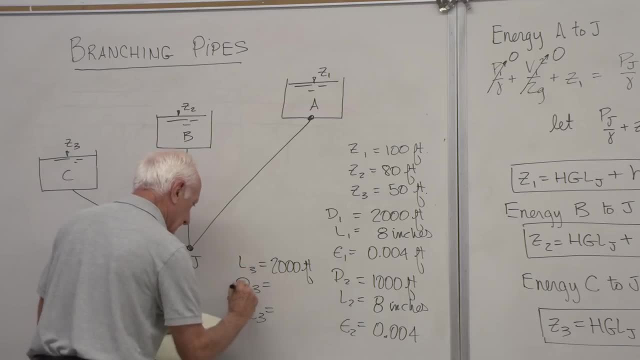 Its diameter is 12 inches, 1 foot. It's roughness, it's, it's rougher pipe: 0.04. Okay, yeah, Oh Yeah, they should be. thank you so much. Yeah, as I said, beef, That's a, that's a big pipe. 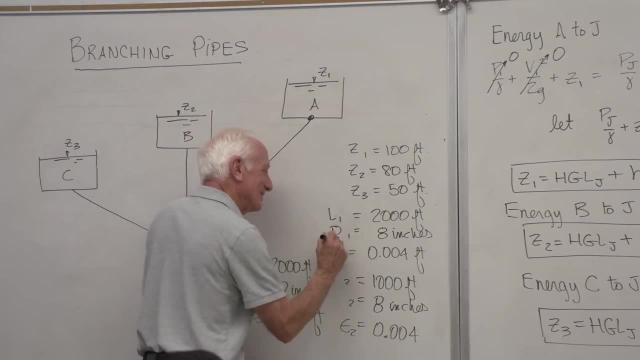 As I said before, if you see something on this board where it doesn't make any sense to you, I don't want you to tell me now. So everybody's notes are the same when they leave class in there. Your notes are correct. good, Thank you so much. 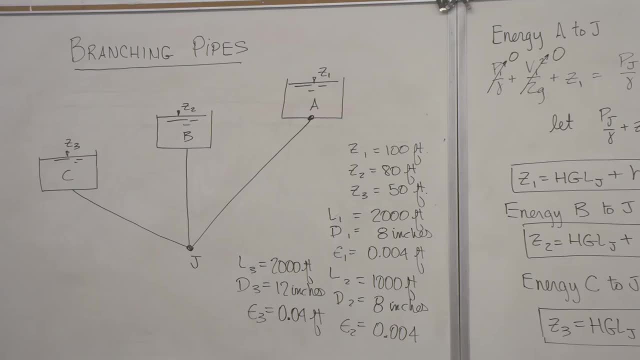 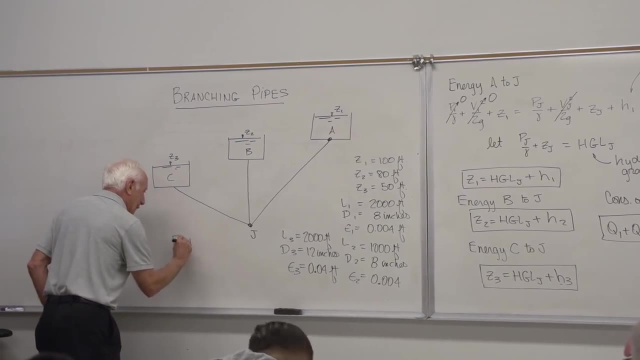 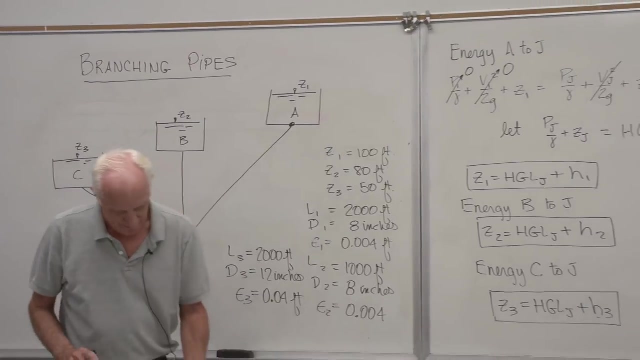 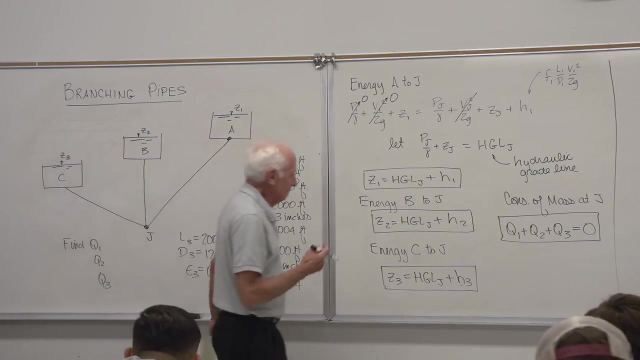 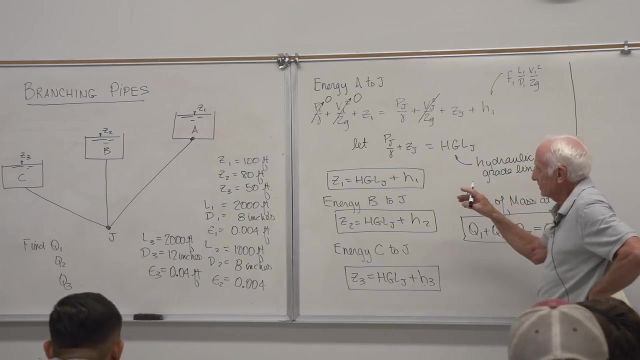 Okay About you know or ask for, or ask for Q 1, Q 2 and Q 3, so find Q 1, Q 2, Q 3. Okay, so that's our starting point. Um, Just so you know, I'll put one of these guys here. 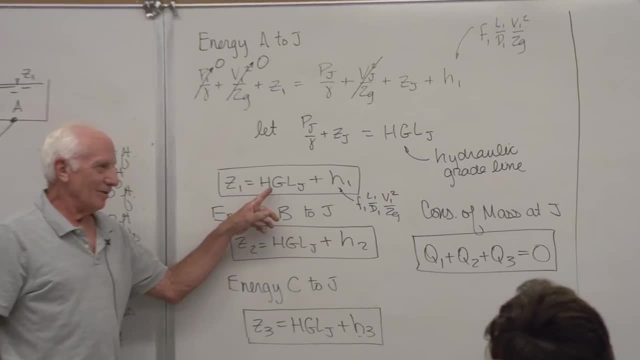 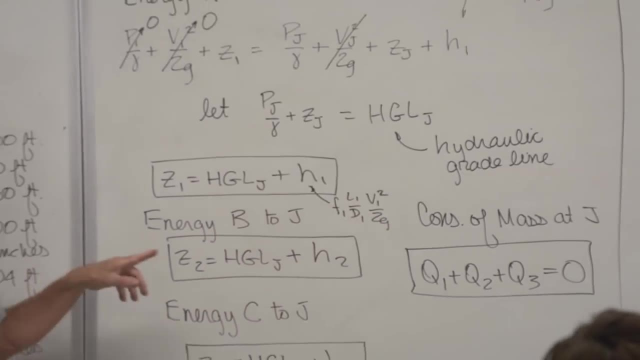 I Don't know how I draw a great line of J. I Don't know f1.. I don't know v1, three unknowns. I Don't know how I draw a great line of J. Don't know f2.. I don't know v2.. I 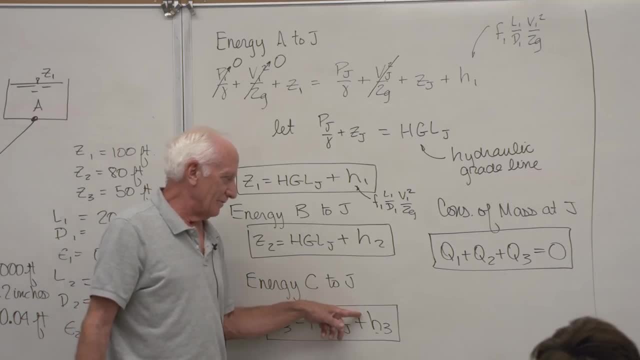 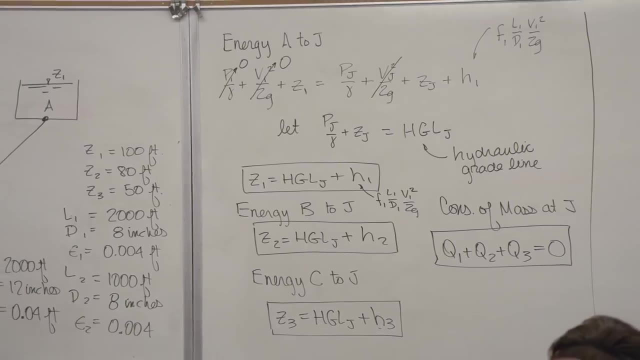 Don't know hydraulic grade line of J. I don't know f3.. I don't know v3. Boy, that's a tough start. Obviously, This is one of the tougher, one of the three series: parallel and branching. Oh yeah, Oh yeah. 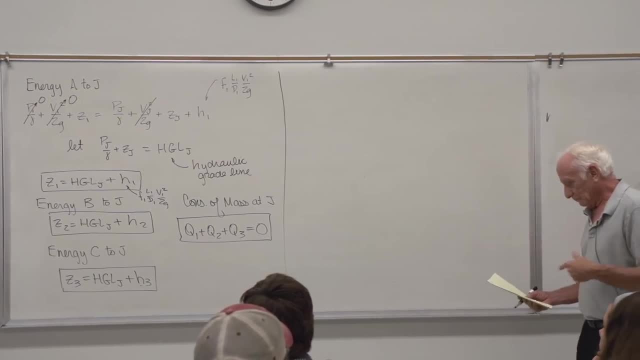 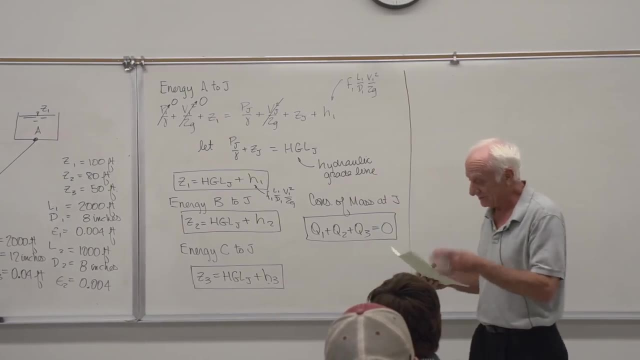 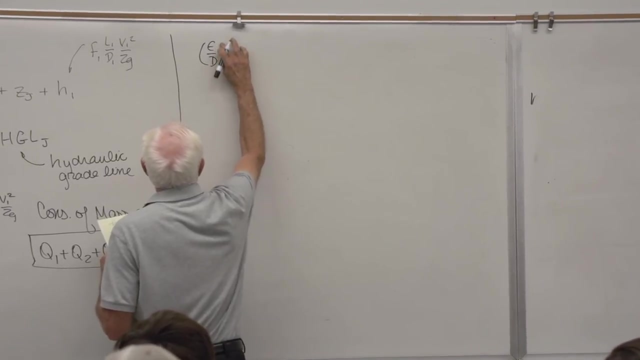 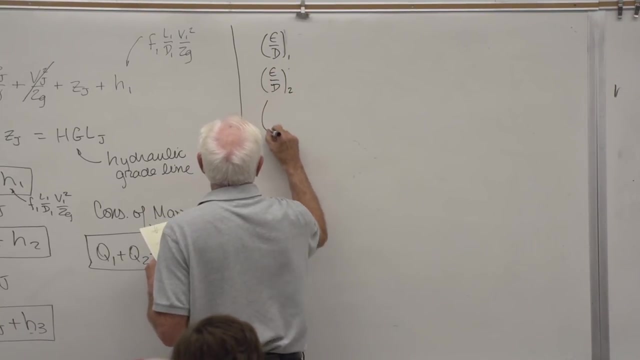 They're not easy. Okay, Got to start somewhere. I'm gonna guess the F. if you don't know the F, two guys to guess the F. okay, so epsilon over D of pipe 1, epsilon over D of pipe 2, epsilon over D of pipe 3, I'm not gonna this. point 0 0 6 and point 0. yeah, point 0 0, 6. 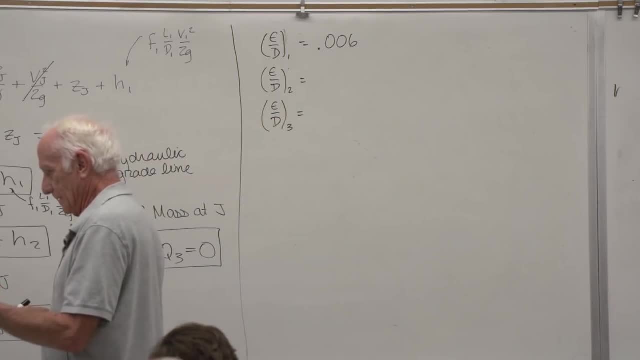 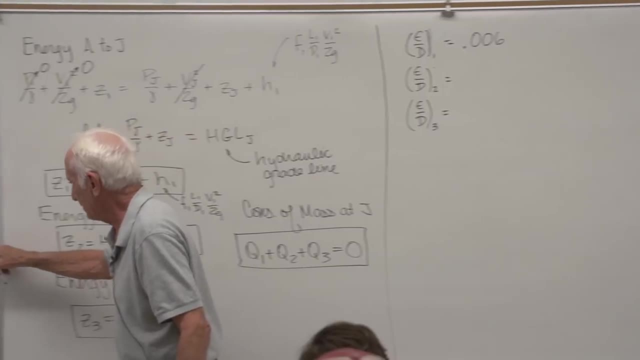 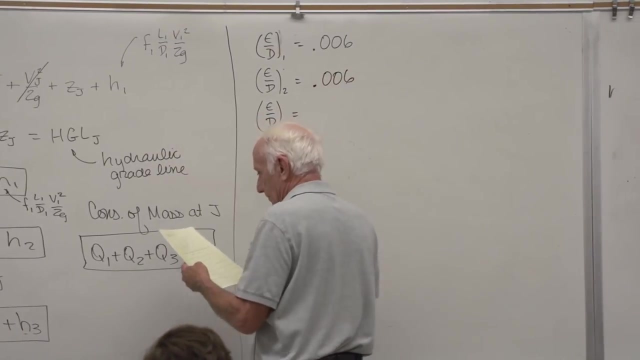 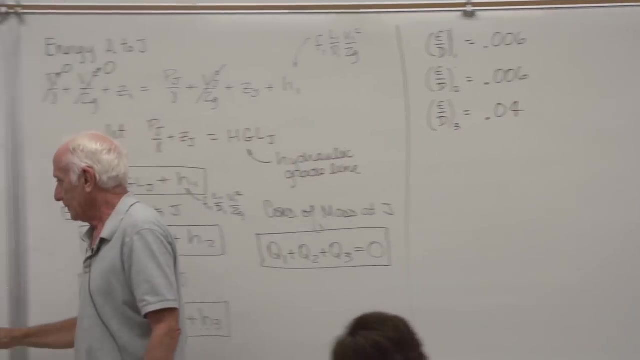 okay, pipe 2. I don't think I got pipe 2 down there. yes, I okay. yeah, okay, it's the same in pipe B, this pipe B and pipe, they're both the same. 0, 0, 4, 8 inches, 8 inches. yeah, okay, 0 0, 6. and now the third one is point 0, 4, whether you want to use an. 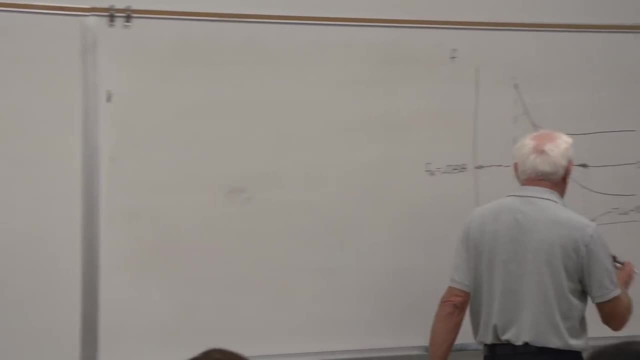 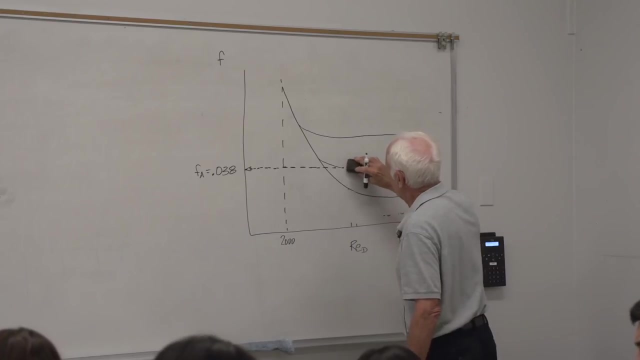 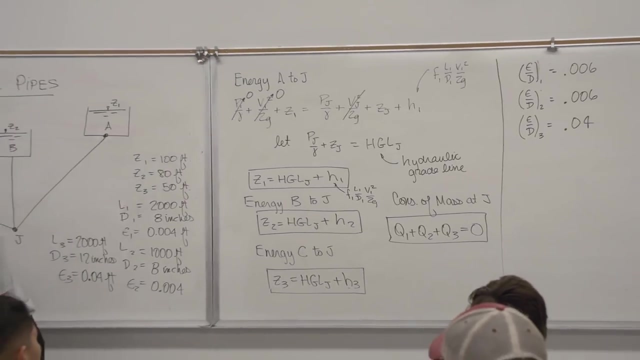 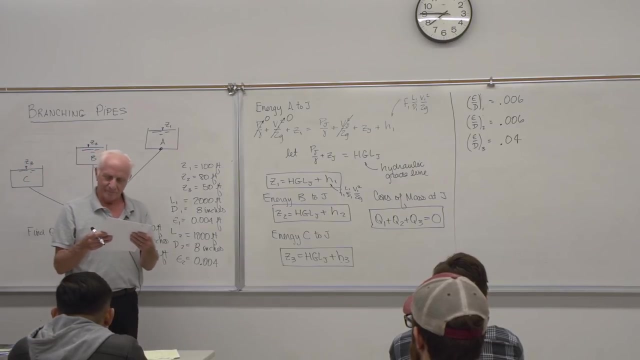 equation, or whether you want to use a moody chart. that's your, your decision to make. I'm going to use the moody chart, though, so I go over here. the rectal curve 1 is a- I don't know the Reynolds number. here's the rule, if you don't know it, first of 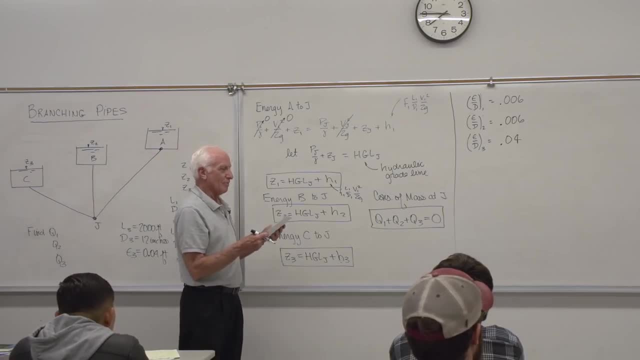 all find the relative roughness curve. let me see if I can find one that maybe is: yep, here we go, mm-hmm, immigration speed objects random 교체 rough. yeah, I can find him zero zero six. yeah, I can find zero zero six. okay. 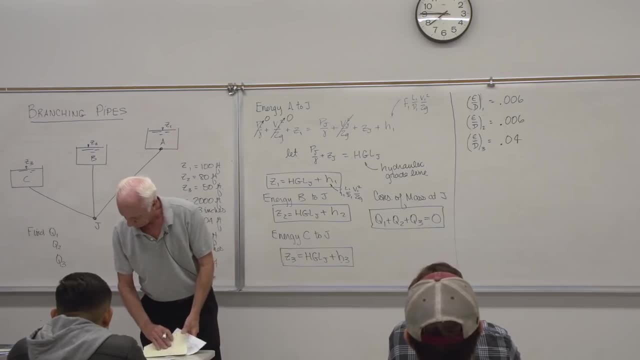 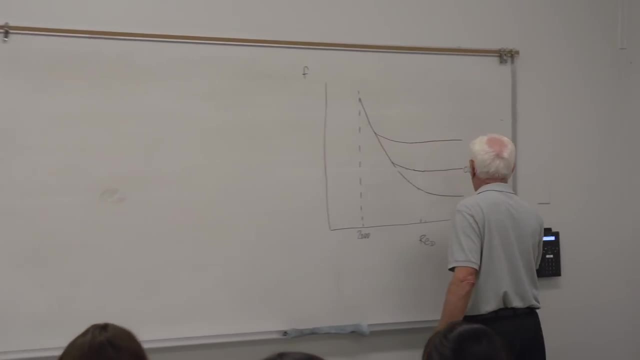 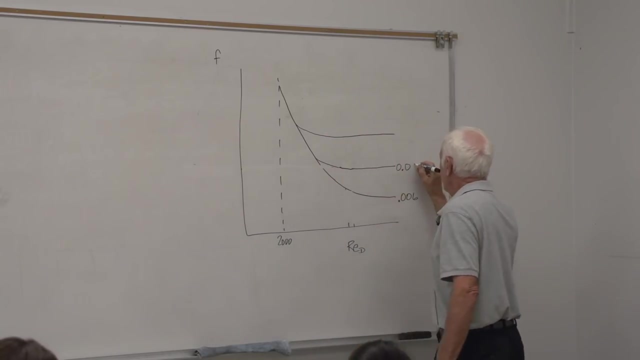 they're both. they're both on that over there. so there's one line label point zero, zero six, and one line on we chart is labeled zero four. I don't need to interpolate between those lines, luckily. I take my ruler. I start out here. where it's flat, it's flat right there. yep, it is. I put my ruler on here. I get my. 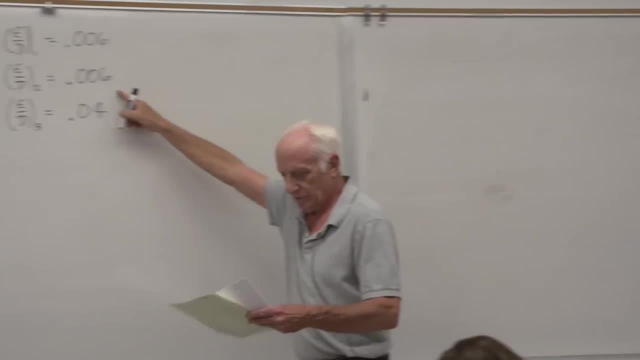 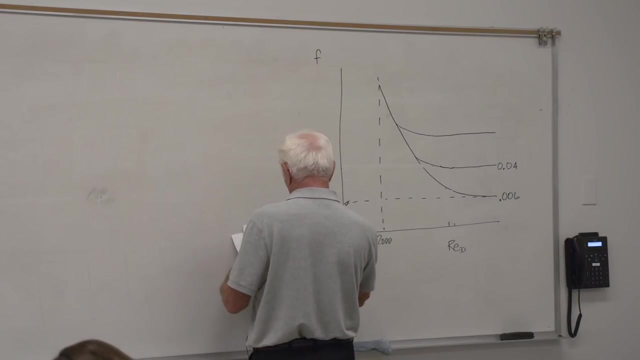 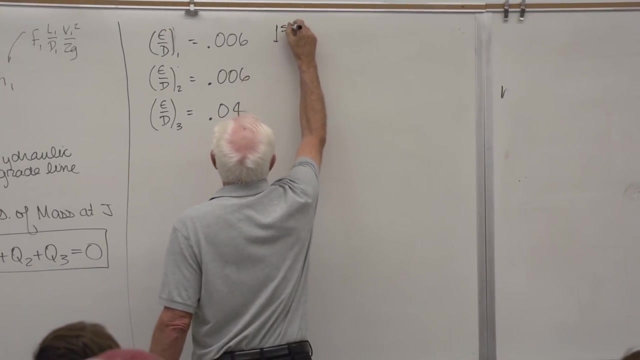 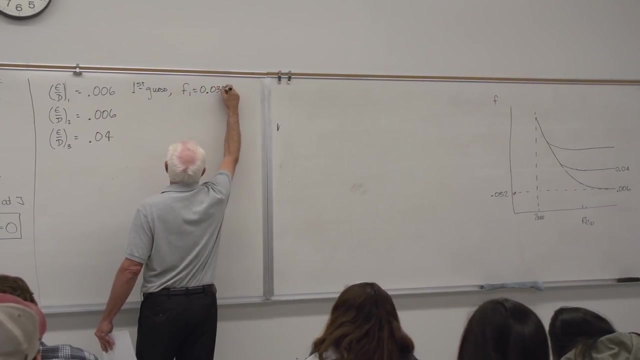 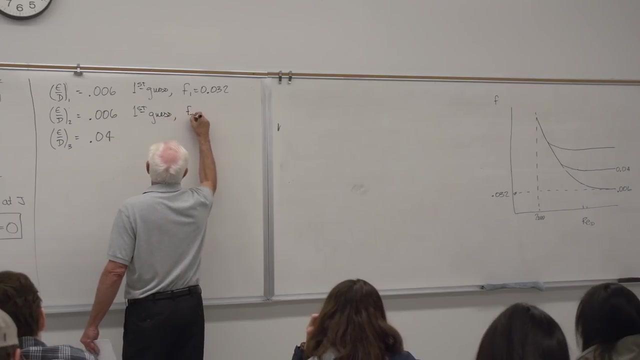 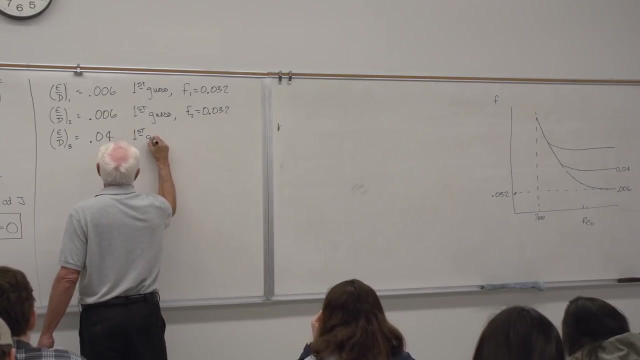 first guess for the F zero, zero, six value and I get point oh, three, two. okay, so first guess F, pipe one: zero. point zero, three, two. first guess pipe two. F equals zero. point zero, three, two. first guess over here. find the epsilon over D, relative roughness: point zero four. put a ruler on the flat part of the curve. put a ruler. 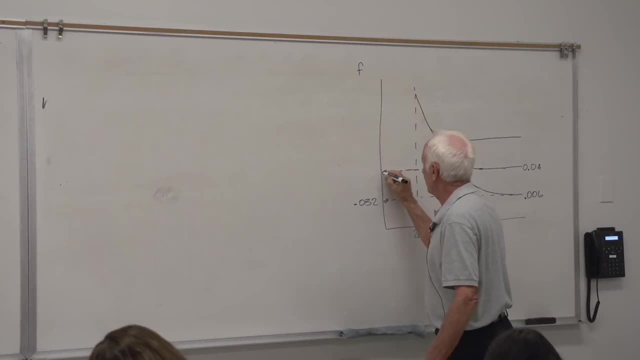 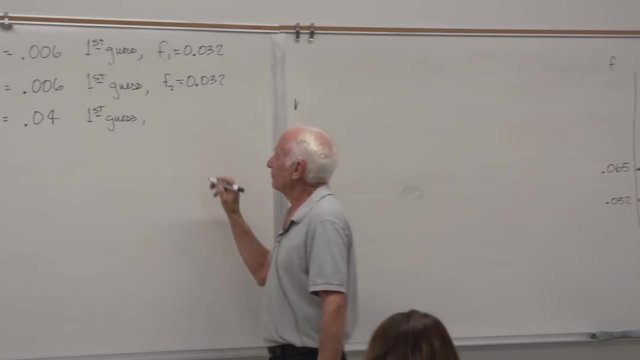 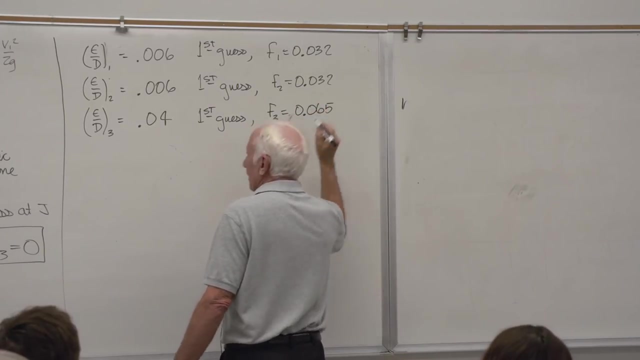 on it. extend the curve and put a ruler on the flat part of the curve. extend the that horizontal line over to here. and my first guess for F for that pipe point: oh, six, five, got it all right. so now I've got those F's as a guess. okay, now I'm going to try and 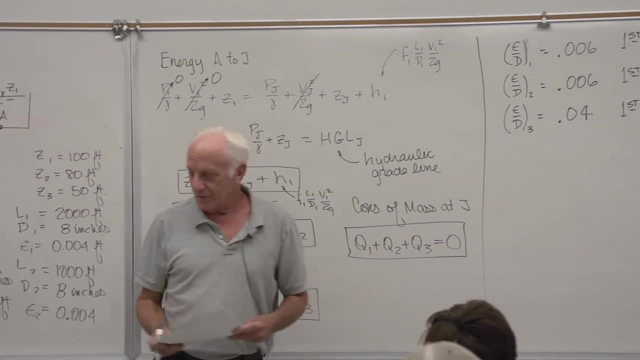 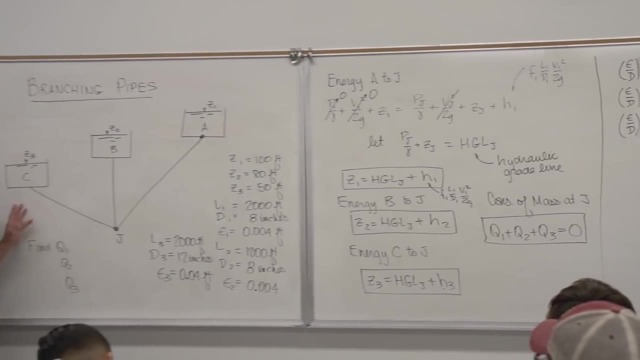 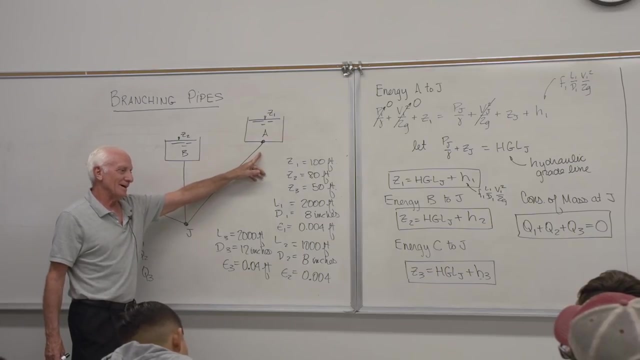 solve these guys. so here's what I've got to realize. I guarantee you I know which way the flow goes in that pipe. I know that that's not a guess. it's going to go down because that reservoir is the highest reservoir of the three. so I know Q goes down that way. this is the lowest of the. 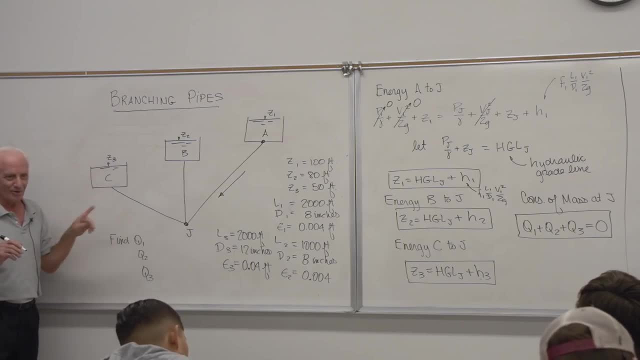 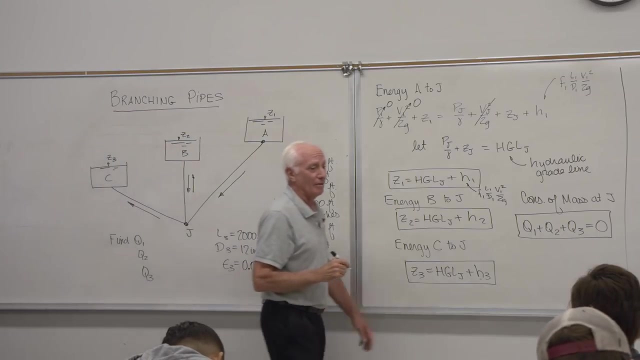 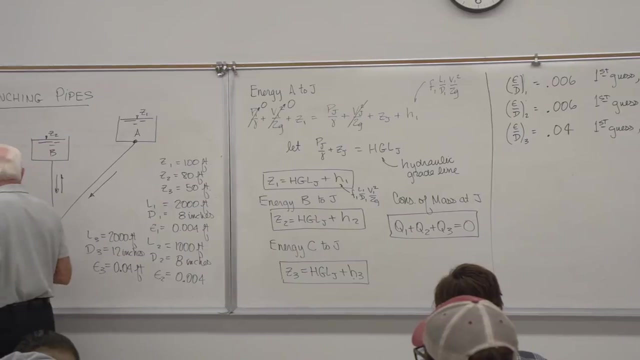 three reservoirs. it's not a guess. I know the flow always goes down to the lowest reservoir. yeah, there it is, those two guys. I know this is a guy I'm worried about. I'm not sure which way he goes right now. I'm gonna find out, but I don't know when I start. okay, so how many unknowns are? 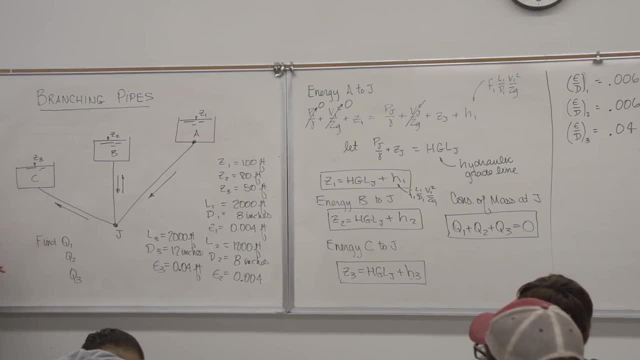 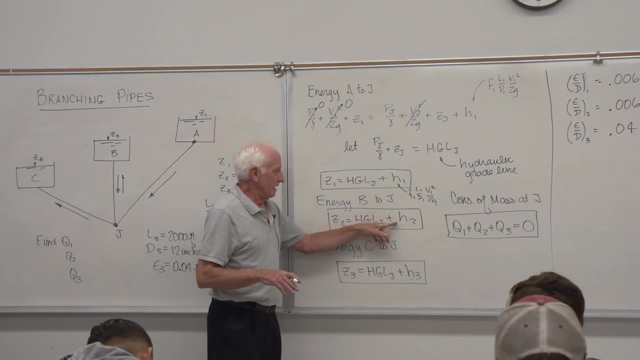 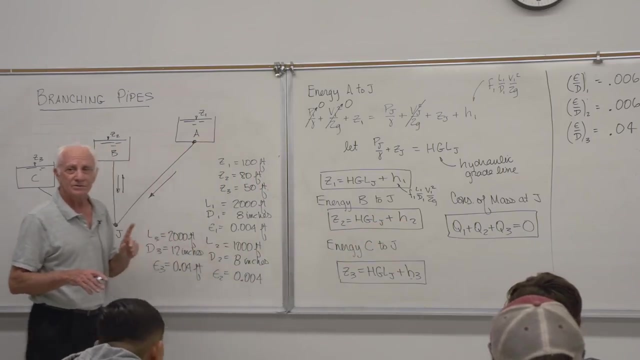 there one, two, three. oh, when I started, how many unknowns were there: F 1, V, 1, 3 here, F 2, V, 2, 3, 4, 5, F 3, V, 3, 4, 5, 6, 7, seven unknowns, seven unknowns. how many equations. here they are. 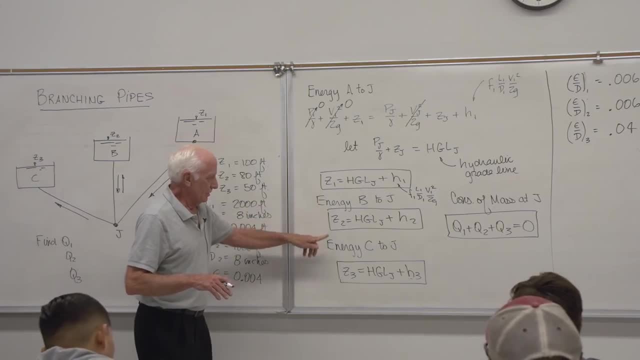 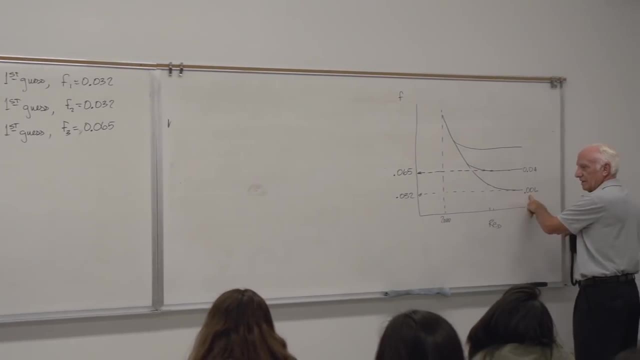 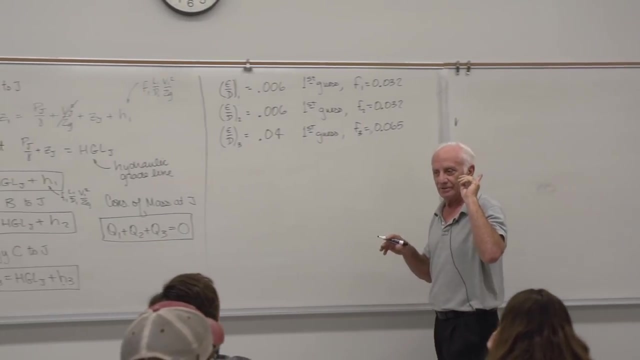 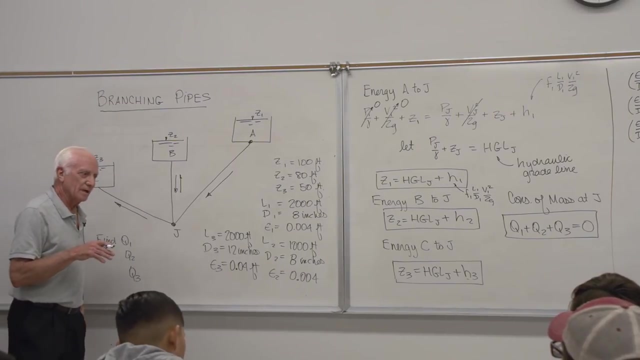 now one, two, three, four. here they come. pipe one, five, pipe two, six equations, pipe three, seven equations. moody chart: three equations, seven equations, seven unknowns, simple problem. oh my gosh, you know it's not a simple problem, it's a very complicated problem. so what I do? first, I guess, three F. 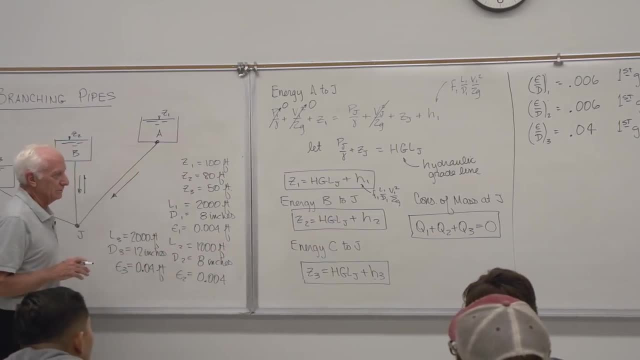 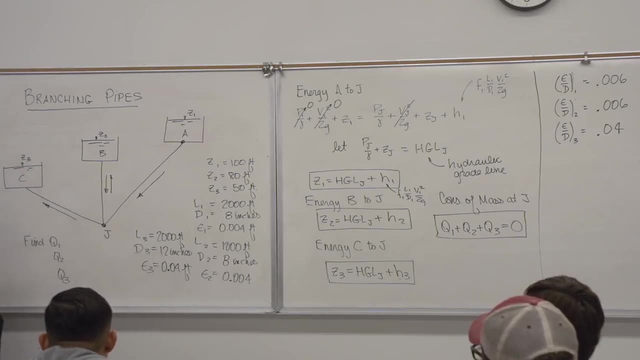 values. what's left? four, unknowns how many equations, four. good, I'm on my way now. I got to do some more guessing. oh, oh, you'll love these problems. I'm sorry, I'm not. you'll like them. maybe you're gonna guess velocities. no, I mean what am I a? 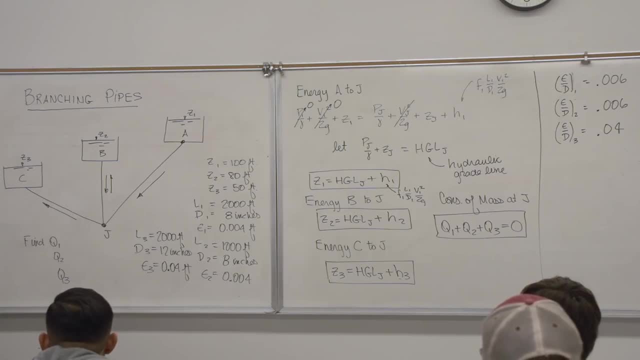 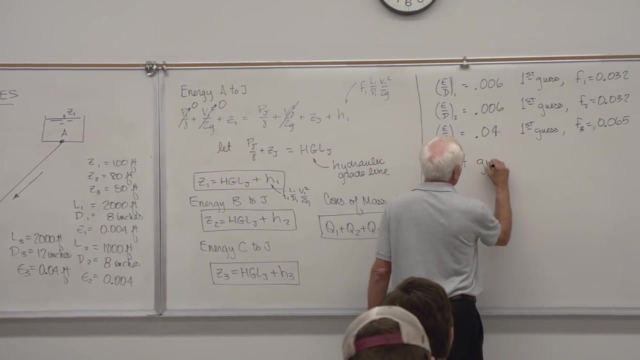 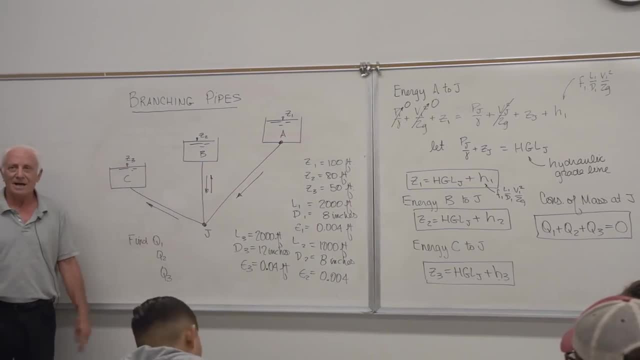 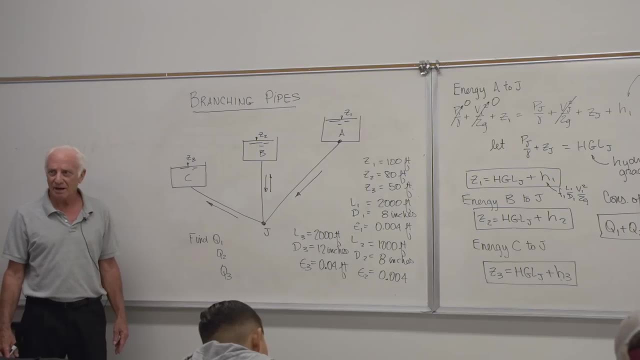 q1. okay, I'll ask anybody in class. the guy says: how do I know? 10 cubic meters per second, a hundred cubic meters per second, a thousand cubic meters per second, how do I know? dr Biddle, I'll say: you know what. you're right. you have no idea, do you? I said no, I don't. 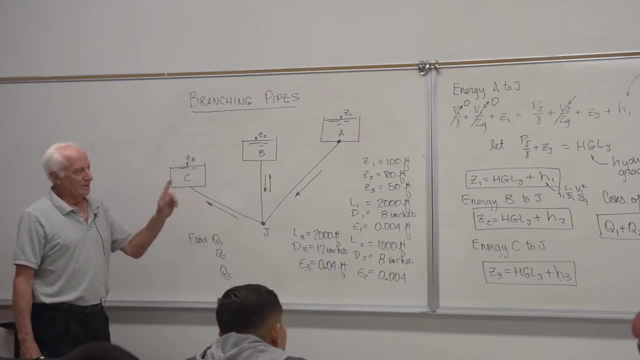 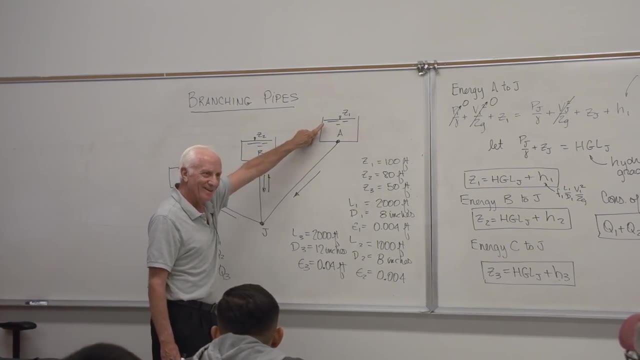 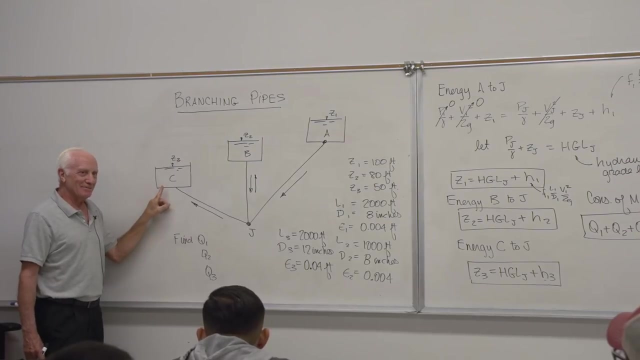 know, I'm gonna ask you guess hydraulic grade line and I'll tell you what it better be. this is what it better be. it better be no higher than z1- okay. and it better be no lower than z3- okay. if it's lower than z3, the flows, all the flows. 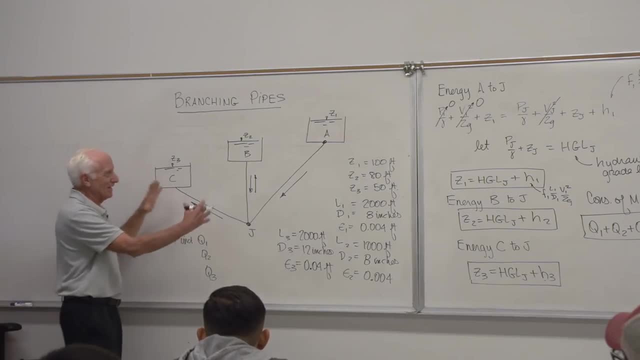 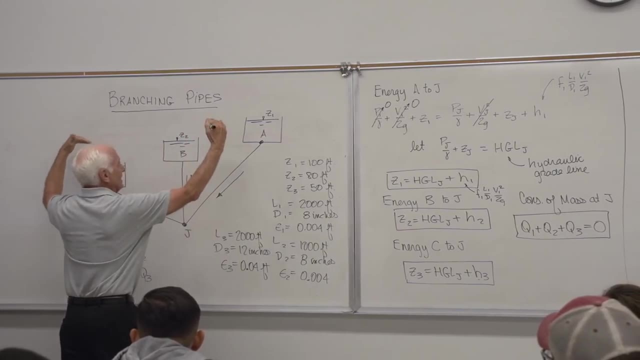 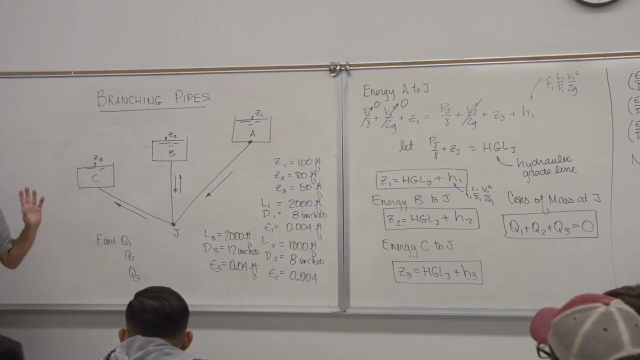 end up coming down. I mean, you know that's the way it is, so don't you gonna make your first guess for that it's, it's. it's a real problem. it's a real problem, it's a bounded guess between these two guys. okay, Z 1 100, z 350. some books say: 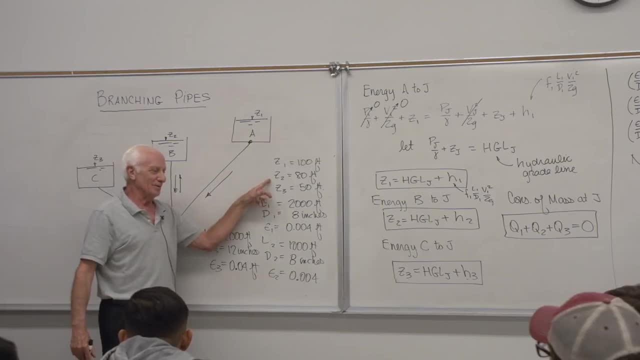 you might as well play the easy game: guess the middle 180. if this is 80 feet and this is 80 feet, the flow rates zero there to start with. okay, I understand that. that's fine, you can do that if you want. which might want to, is we don't? 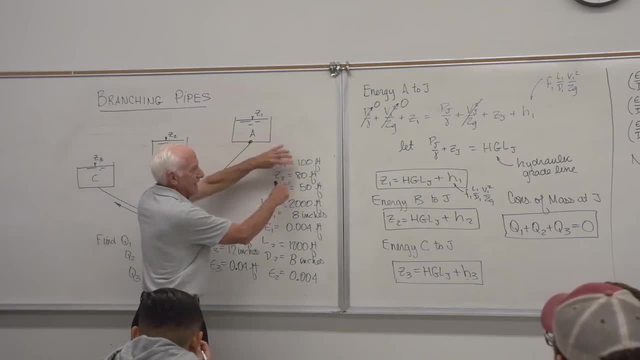 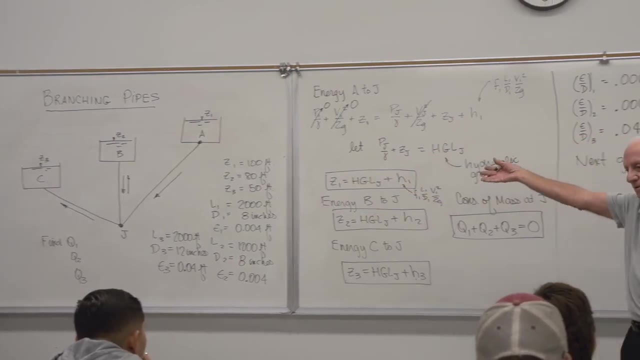 know these guys make your first guess: hydraulic grade line as the middle 180. I said you know what I'm just gonna guess 75. it's halfway between 100 and 50, I guess halfway between. so hydraulic grade line of J equals 75. okay, now here it. 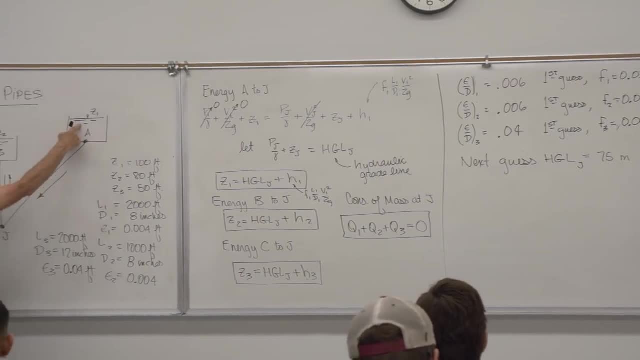 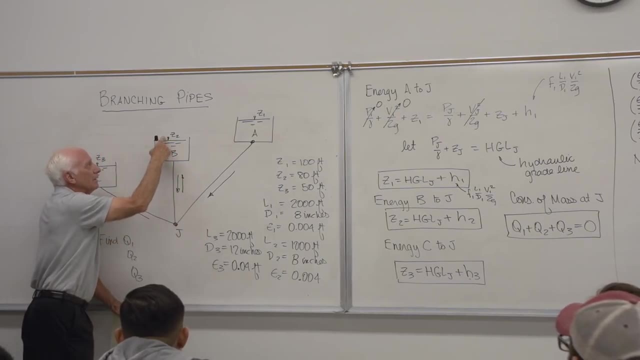 goes. he's a hundred, he's 75. water goes down. by the way, this is all water. so you know, this is 75, this is 80, this is 75, this is bigger, 80. flow goes up. this is 75, this is 50. flow goes up, so I guess 75. okay, oh wait, that was Z. 2 is 80, I'm so. I. 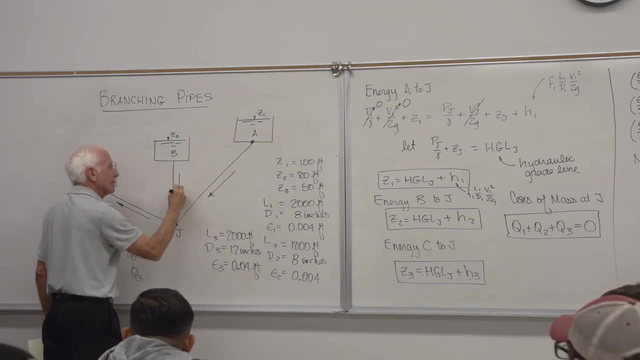 got a flip-flop, that was 80. that's 75, pardon me, so I'll put up here so I get them right. 100 feet, 80 feet, 50 feet. okay, my first guess: hydraulic grade line J equals 75, a hundreds greater than 75. flow is down. 80 is greater than 75, flow is down 75 is. 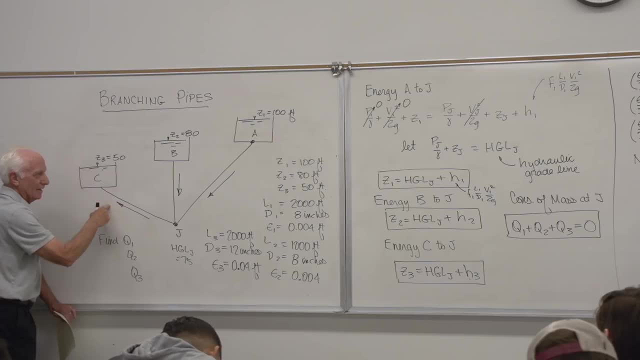 greater than 50, flow is up. okay, do I need to change my equations now? well, okay, do I need to change my equations now? well, okay, do I need to change my equations now? well, of course I do. I'm gonna write the. of course I do. I'm gonna write the. 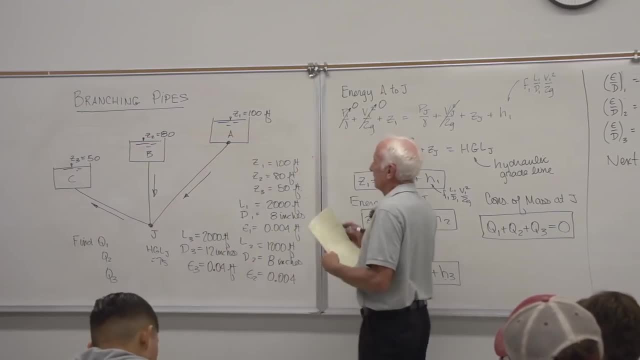 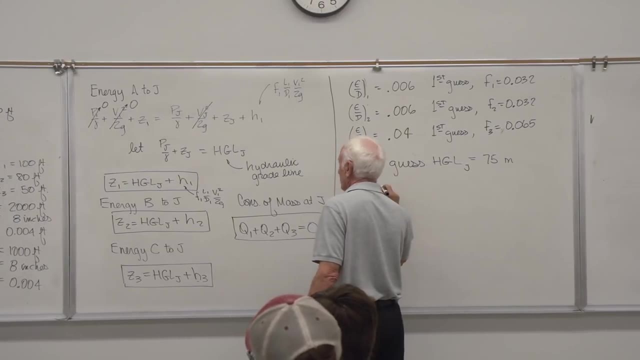 of course I do. I'm gonna write the the equation from here down to there. okay, the equation from here down to there. okay, the equation from here down to there. okay, from Z 1 down to J: there it is Z 1. from Z 1 down to J: there it is Z 1. 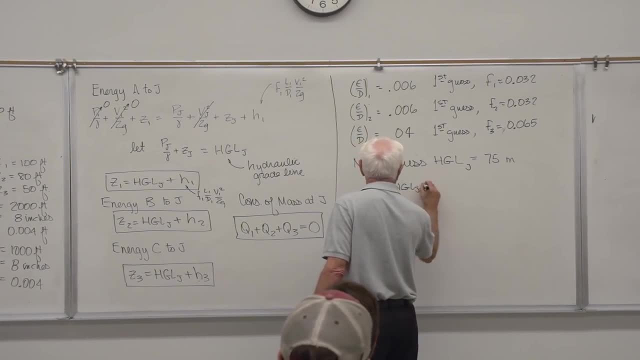 from Z 1 down to J. there it is Z 1. equal hydraulic grade line at J plus F. equal hydraulic grade line at J plus F. equal hydraulic grade line at J plus F. 1, L, 1, D, 1, V, 1 squared over 2 G. okay, Z 1. 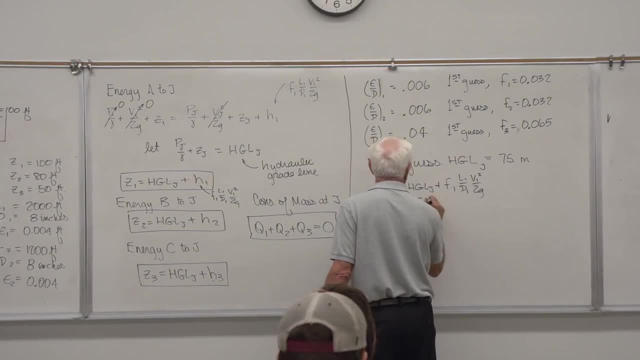 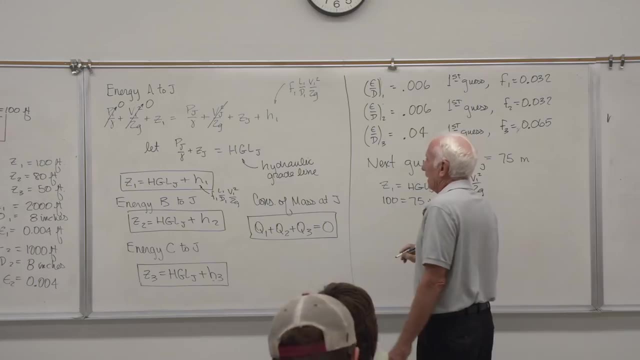 1 L, 1, D 1, V 1 squared over 2 G. okay, Z 1 a hundred. my guess a hundred. my guess 75,. F1, my guess 0.032.. L1, 2,000.. Diameter: 8 inches: two-thirds Times the velocity. 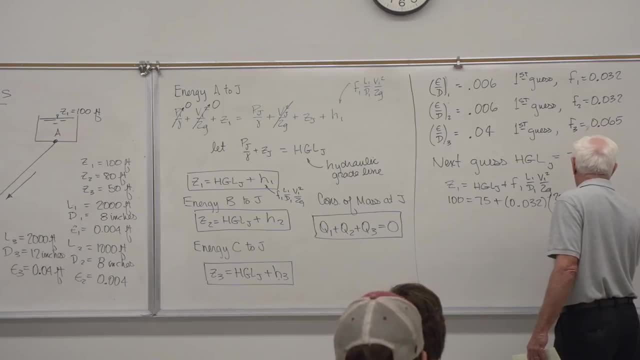 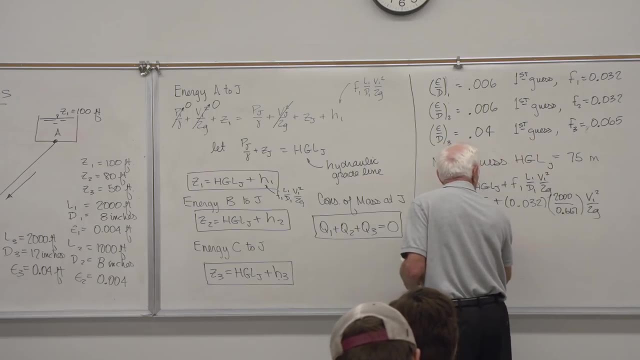 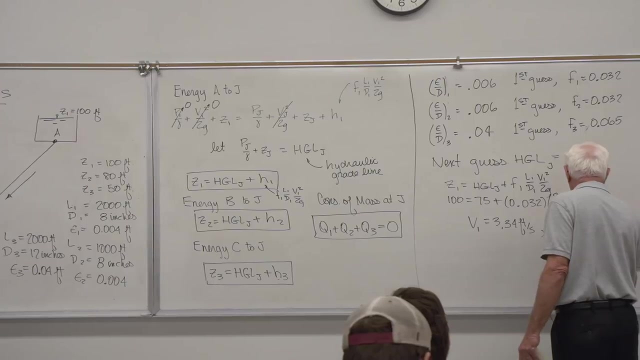 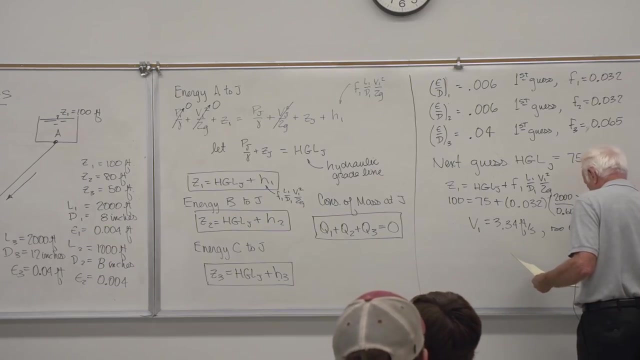 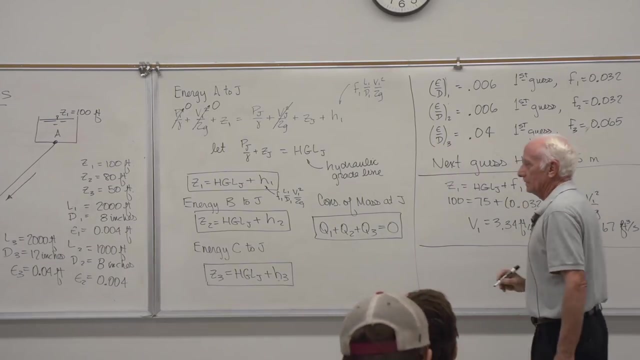 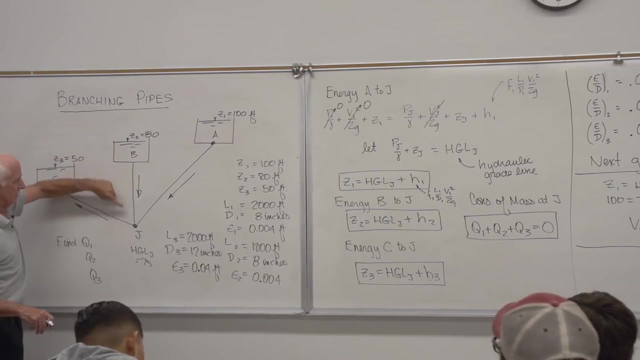 squared, V1 squared Divided by 2G got it 32.2.. V1 equal 3.34 feet per second. So Q1, V1 times A1, 1.167 cubic feet Per second. OK, that's pipe. one, Pipe, two flows going from the reservoir down. 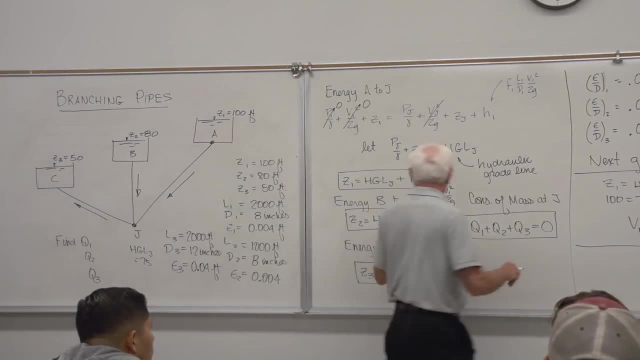 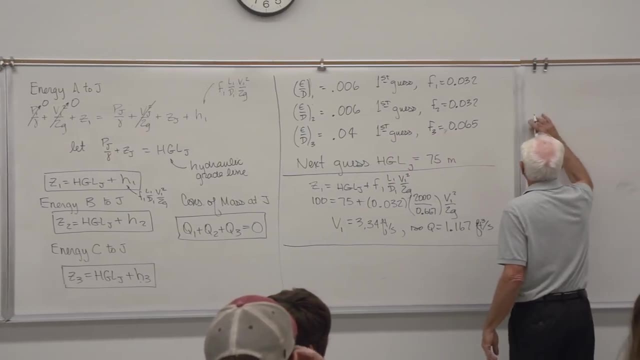 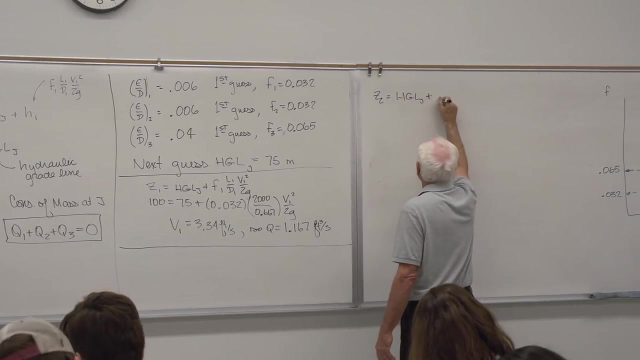 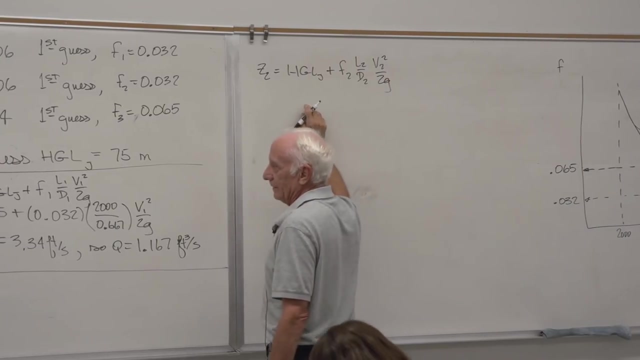 to J: OK 80.. Same thing, except be careful now. OK 80,. same thing, equal this. So now we have- I'll write it down- Z2, equal hydraulic Hydraulic line at J plus F2, L2 over D2, V2 squared over 2G. Here we go. Z2 is: 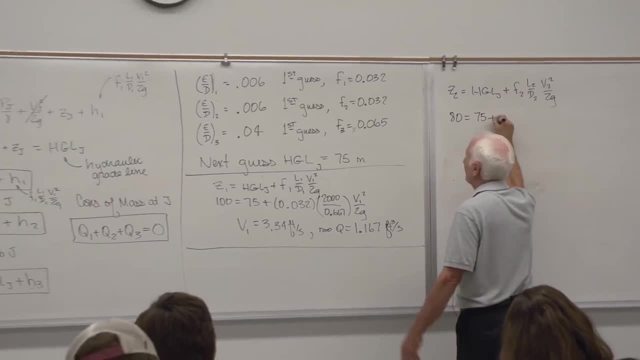 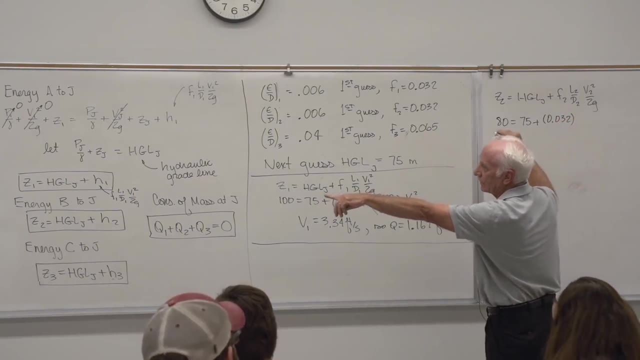 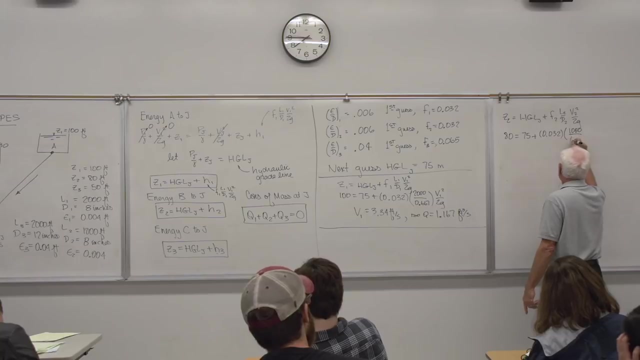 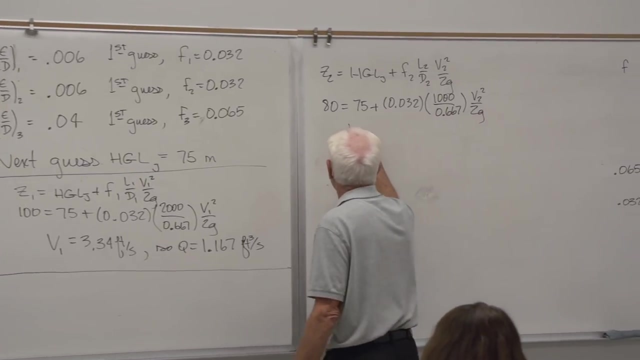 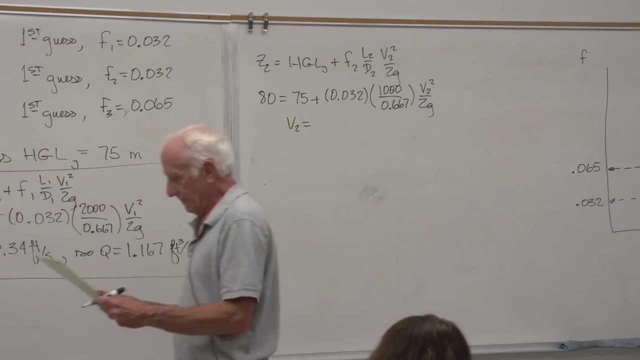 80.. My guess hydraulic grade line was 75.. My guess for F2, 0.032.. L2 over D2, 1,000 and three two-thirds 1,000 and two-thirds And two-thirds Times V2 squared over 2G, Solve for V2.. V2 comes out to be 2.59. 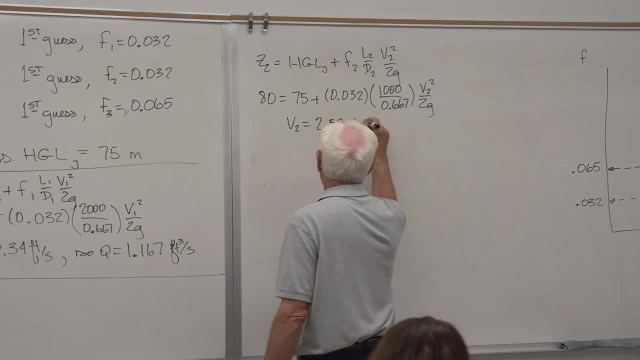 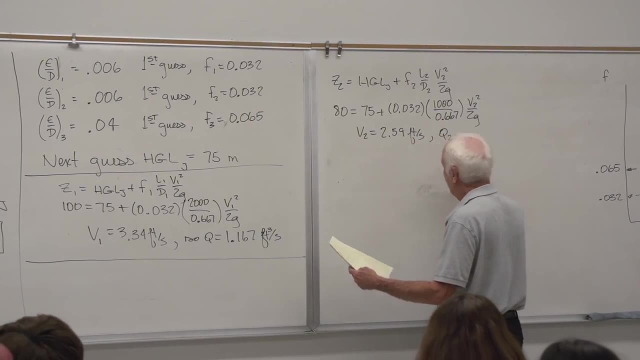 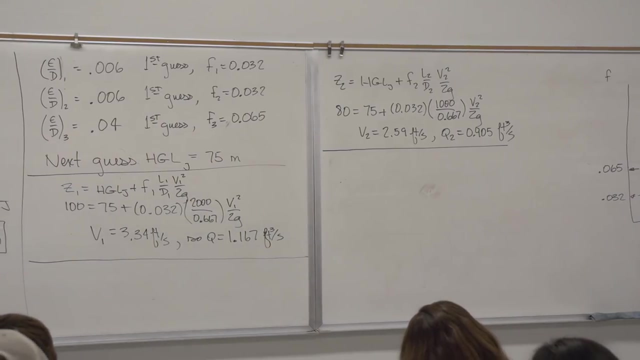 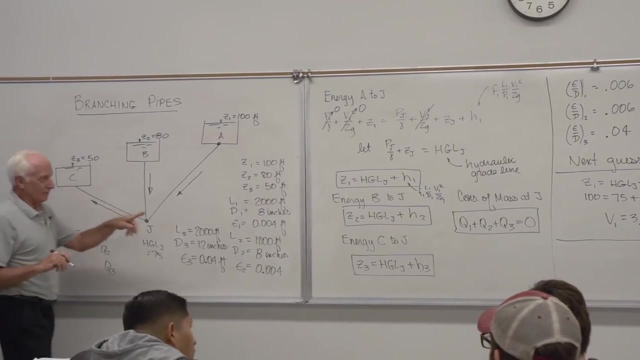 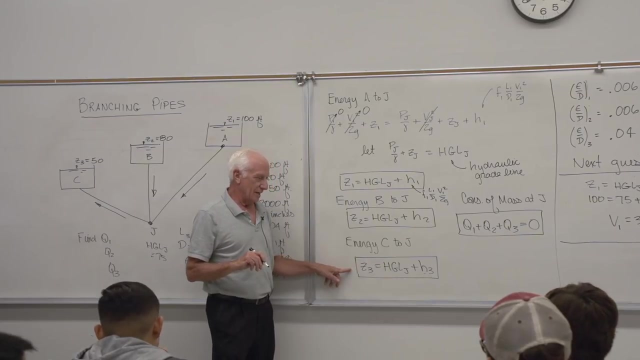 feet per second. So Q2 equal V2, A2, 0.905.. Cubic feet per second: Got it. Now comes the third one: The flow goes from J to here. Don't write it like this, because this one assumed the flow went from Z3 down to J. No, it went, it's the. 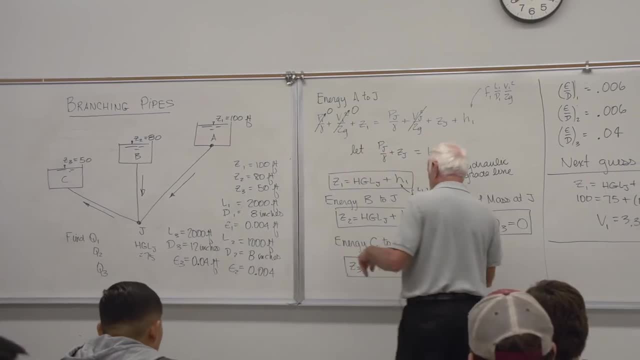 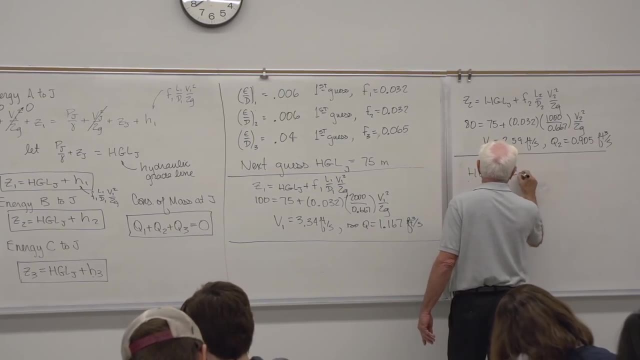 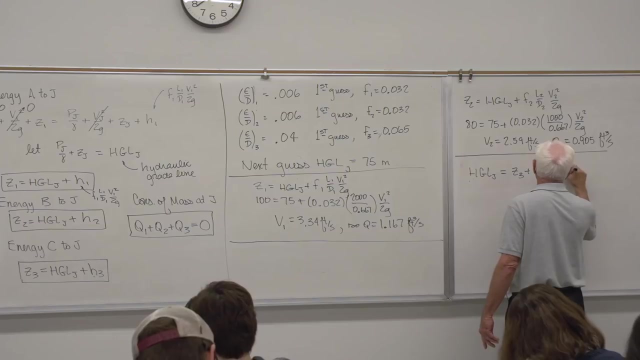 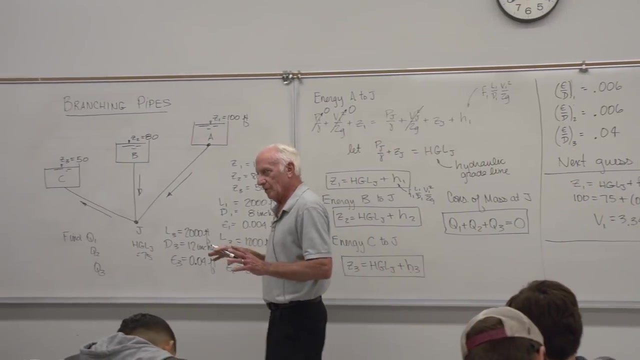 other way. So now this equation is flip-flopped. Hydraulic grade line at J equals Z3 plus F3, L3, D3, V3 squared over 2G. You have to change the equation to fit the way the flow is going. 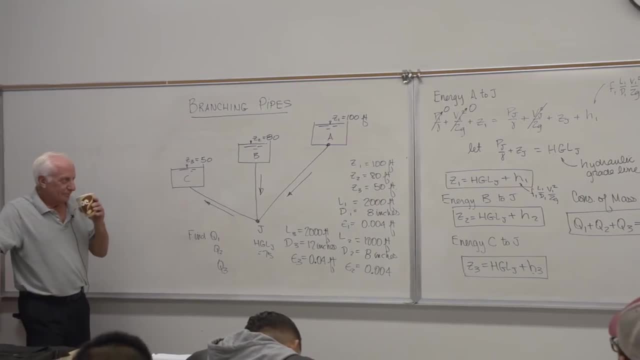 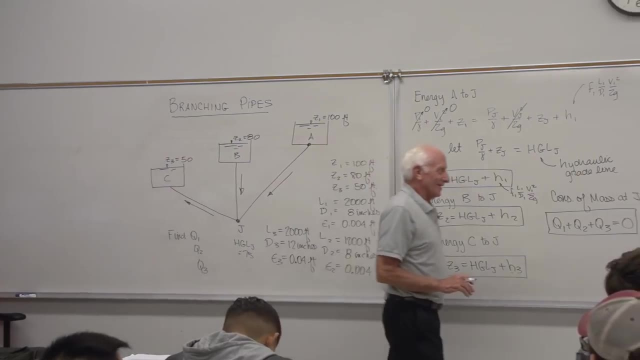 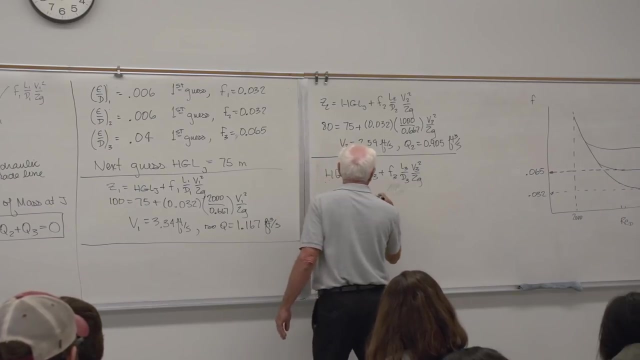 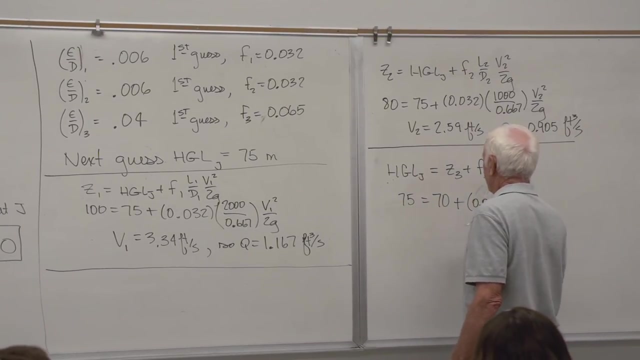 Okay, Hydraulic grade line at J. What did I guess? 75, yeah. What's Z3?? 70, yeah. What's my guess on F3? 0.065.. Did I get it right? I'm sorry. 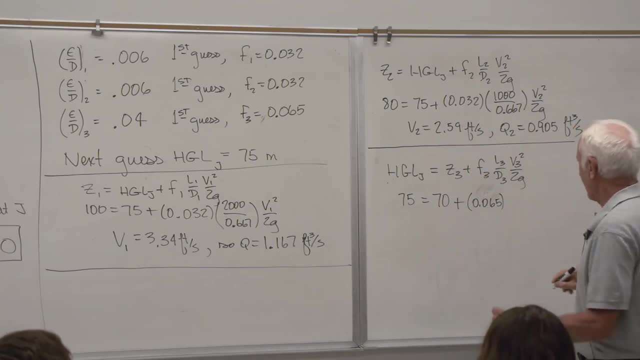 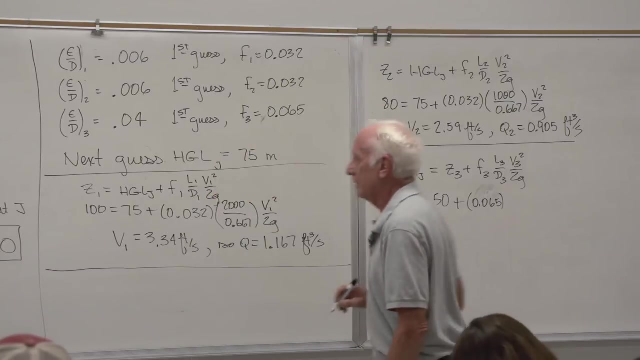 For Z. oh, this one, Oh, thanks, thank you, thank you, thank you. Okay, right, L3 way over there. L3, 2,000 divided by 1.. V3 squared over 2G, So V3 comes out to be: 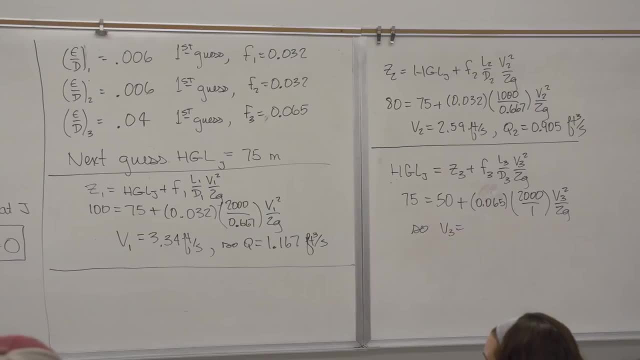 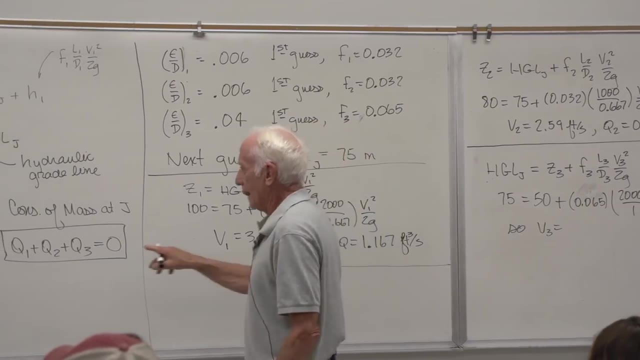 yeah, On the Z1.. Which one now, I'm sorry on the Z1.. This one, Yeah. So for D1, would it be 0.75?? No, 8 twelfths is 2 thirds. That's up. Oh, is he? No, he's 2. 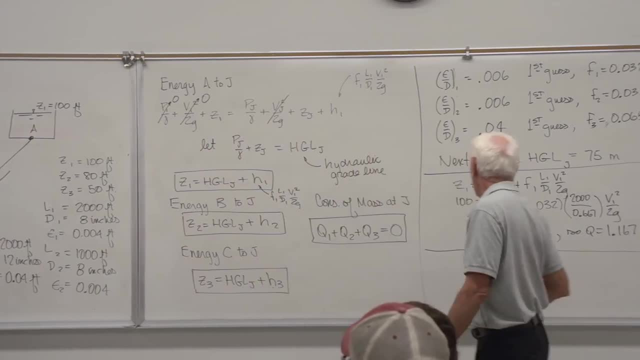 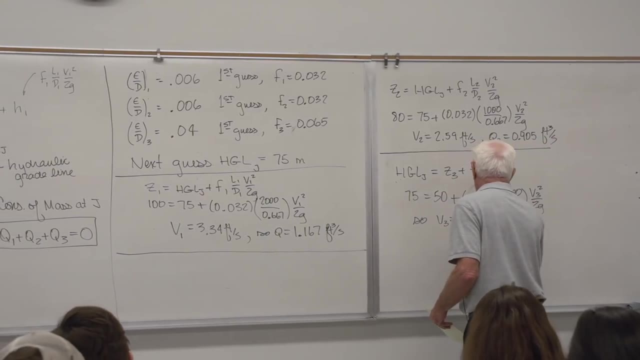 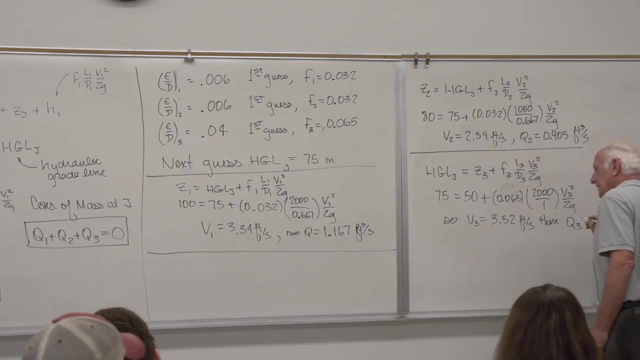 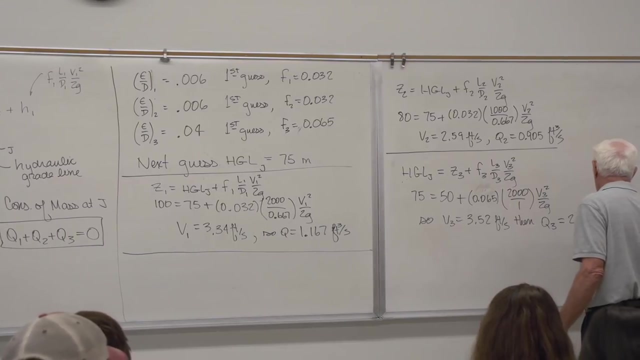 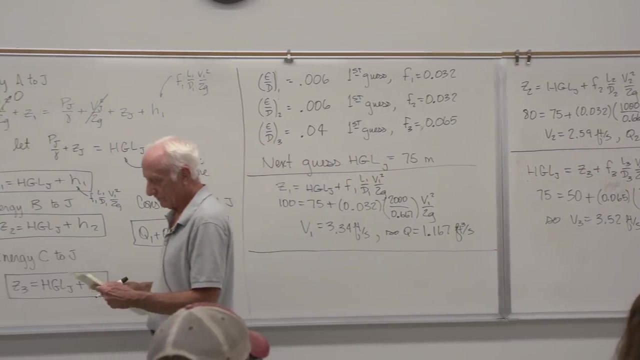 thirds. 8 twelfths is 2 thirds, 0.667.. Right, V3 is 3.52.. Okay, Okay, Okay, Okay, Okay, Okay. Q3 is equal to V3 times A3, 2.763 cubic feet per second. Got it? Okay, we're getting. 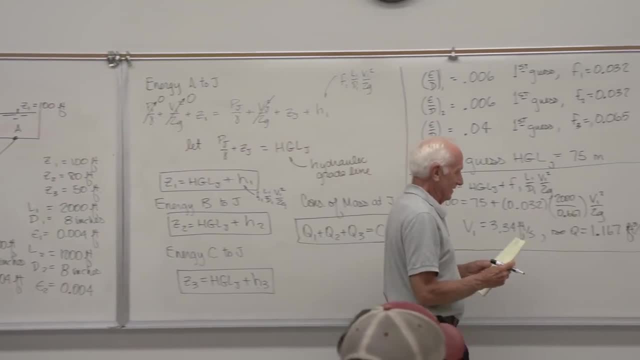 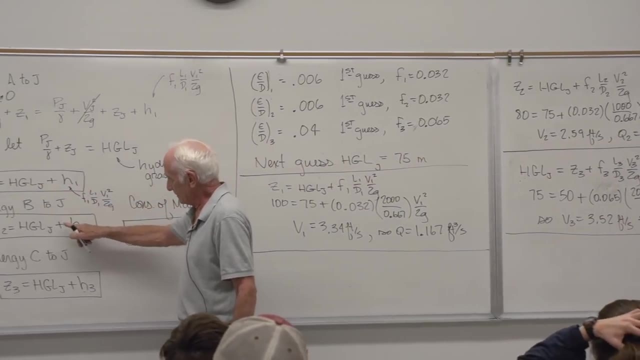 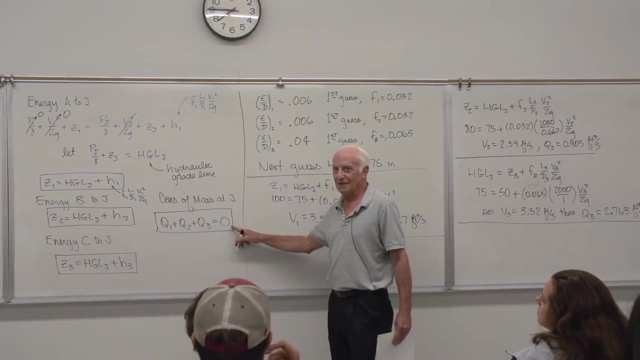 there. All right, I used him, I used him and I used him. I've used three of the four equations. Guess what I do now? I try him, and he better work out to be zero or I'm in deep trouble. Okay. 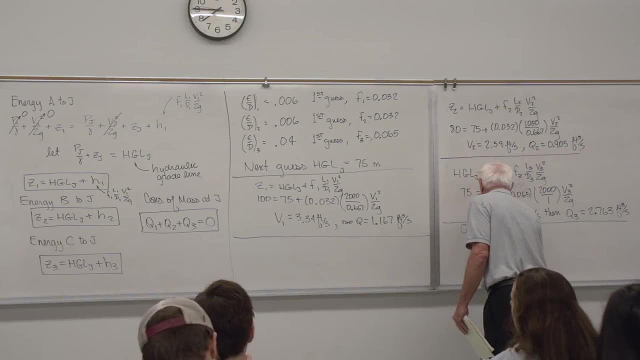 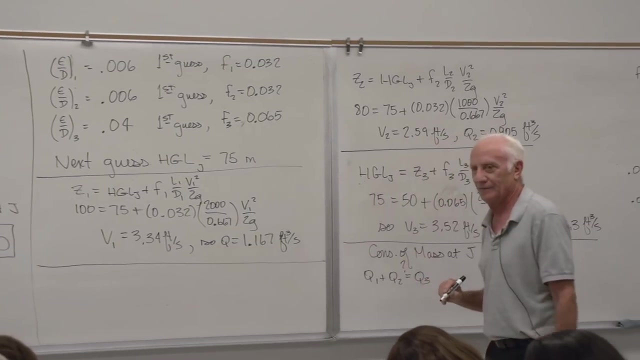 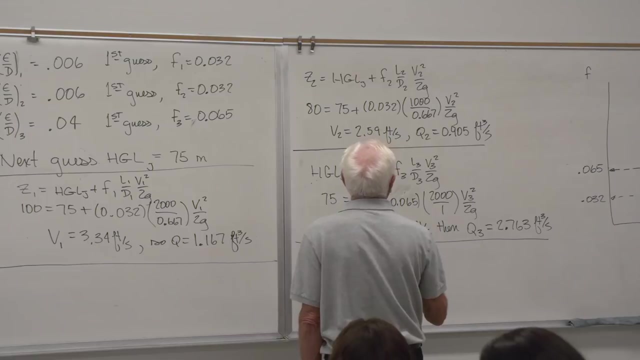 Continuity. conservation of mass. Okay, Okay, Okay, Okay. Q2 comes in, Q3 goes out. I don't know if that's right or not. Let's find out. Q1, 1.167 plus Q2, 0.905.. Does that equal to Q3, 2.6,, 2.7,, 6, 3? 2.072, does not. 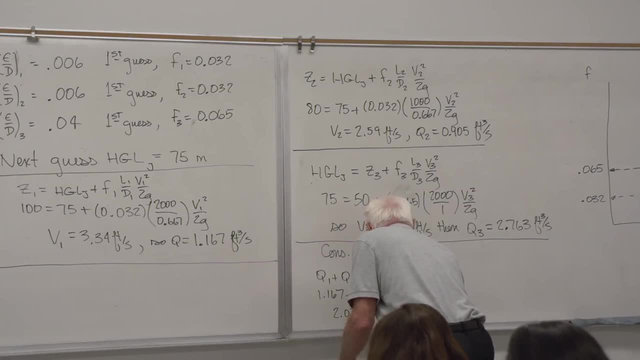 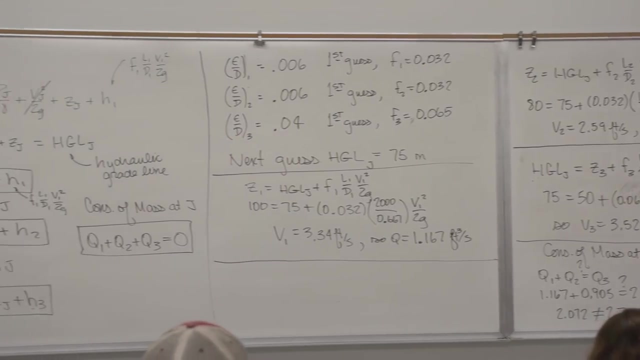 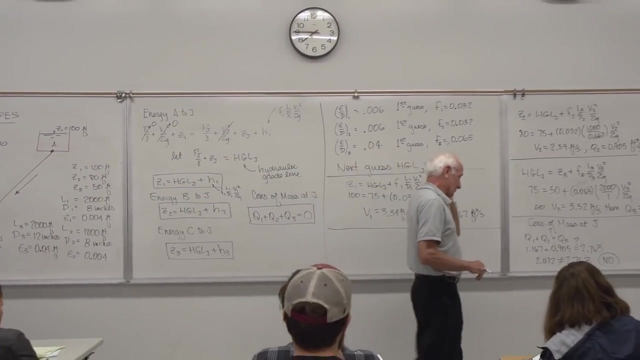 equal to 2.763.. No, that didn't work. Nice try, though, Good practice anyway. Nope, we didn't satisfy continuity, So I say okay, all right. So what's too much and what's not enough? I got too much stuff going to reservoir three. 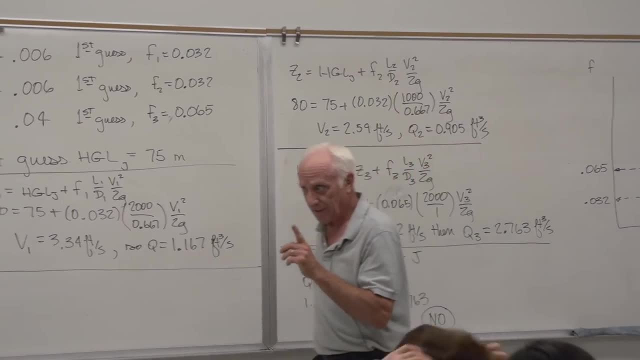 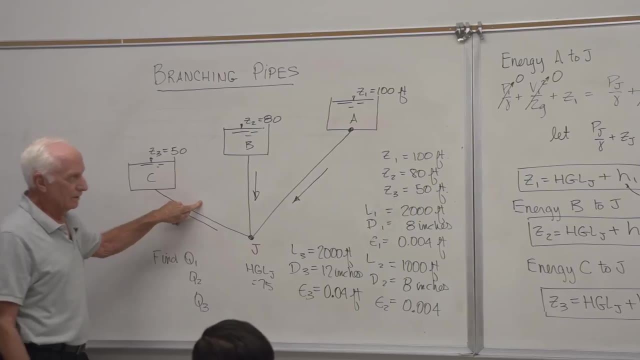 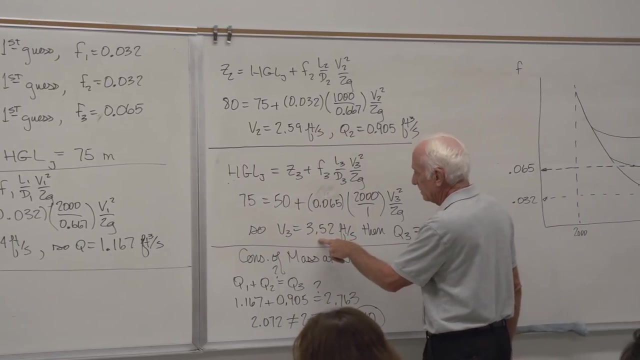 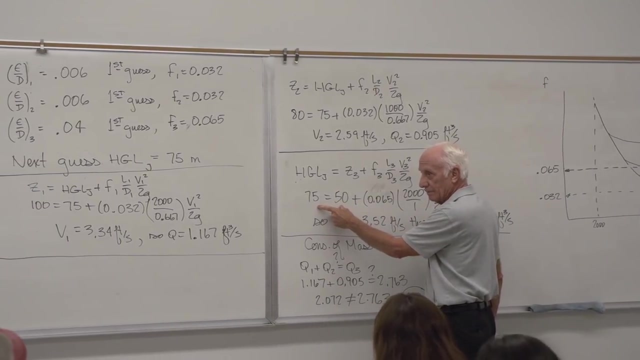 And not enough stuff coming down. Okay, that's the key. I want less flow here. I want less flow here. I want that to be smaller. Only way that guy V3, gets to be smaller is if these two guys are closer together. Okay, now you know what your next guess is going. 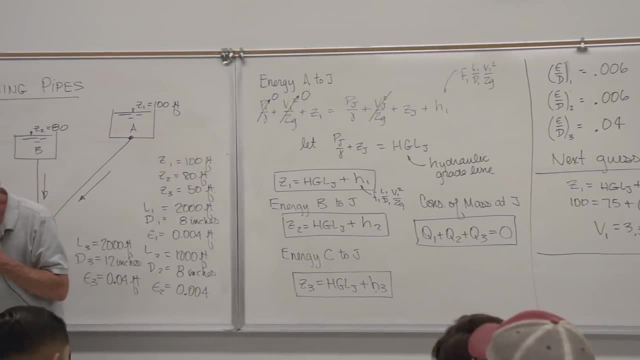 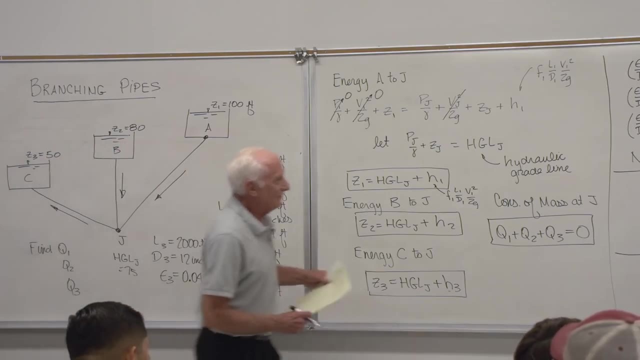 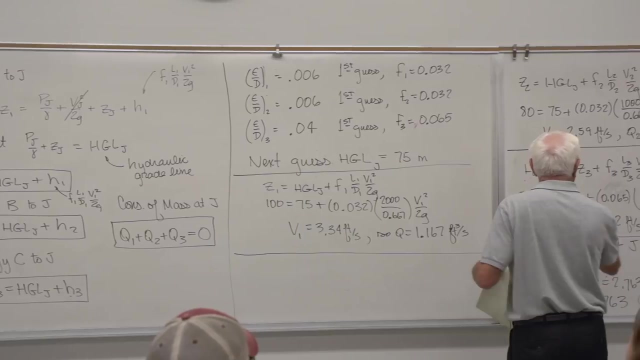 to be. Let's see what I guessed. Where's my next guess? Oh, here we are. I said, you know what I guessed: 75.. What if I make that 70?? That'll mean the V3 is smaller, That'll. 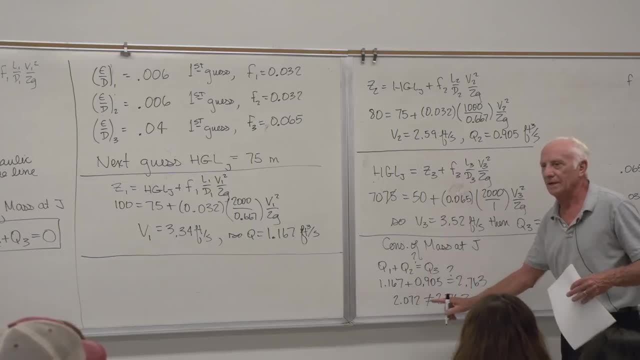 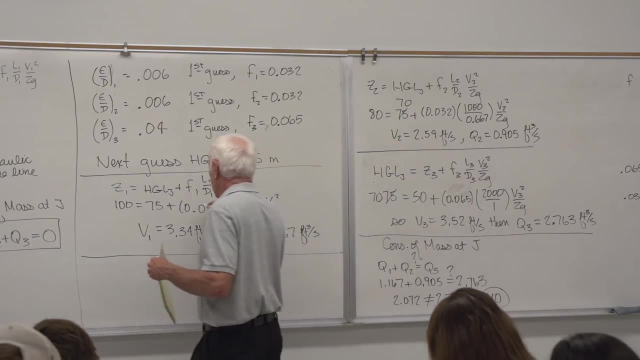 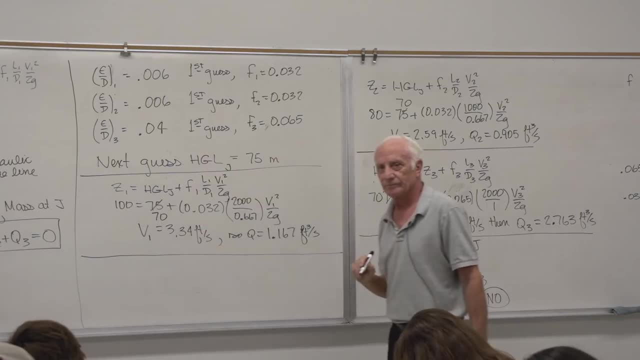 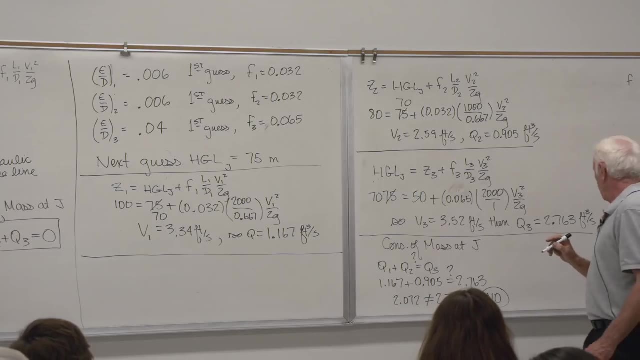 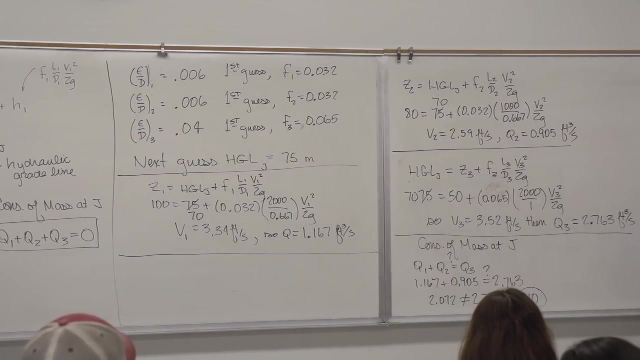 guess 70.. You make those three changes. I'm guessing 70. now I'm trying to save some board space here. okay, Now, when I'm done with this, I'll put in. I'll put in. I'll just put the new. I'll put in the new V's and I'll put in the new Q's. 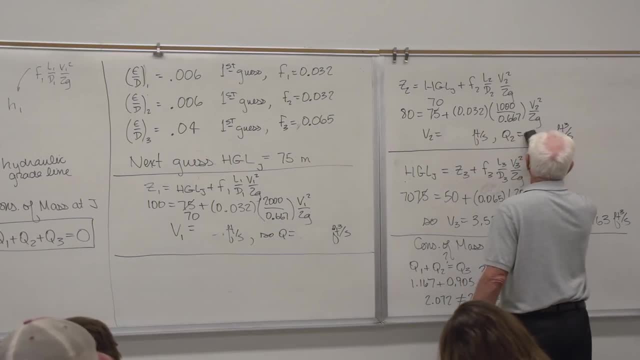 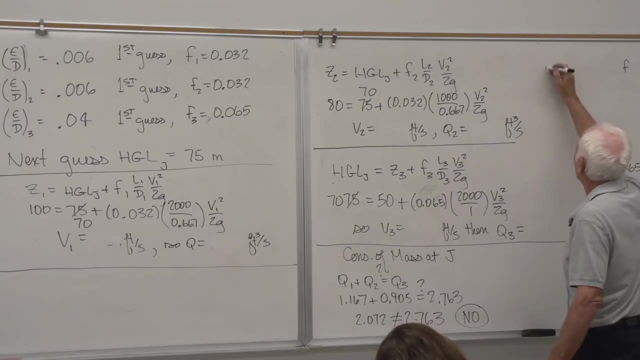 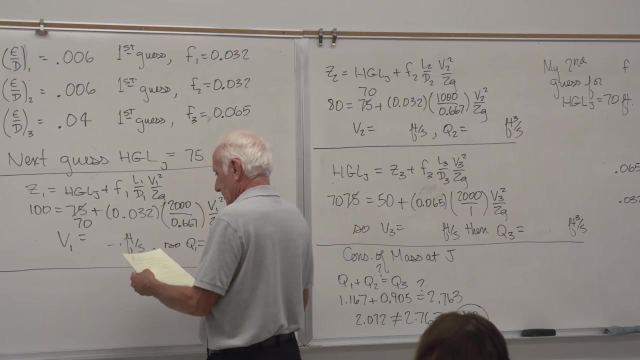 and I'll put in the new V and I'll put the new Q in. Okay, so now my second guess for hydraulic grade line at J is 70 feet. Okay, Let's see, I tried 70.. Okay, I didn't get the velocities, but I got the Q's, Q1,, 1.2,. 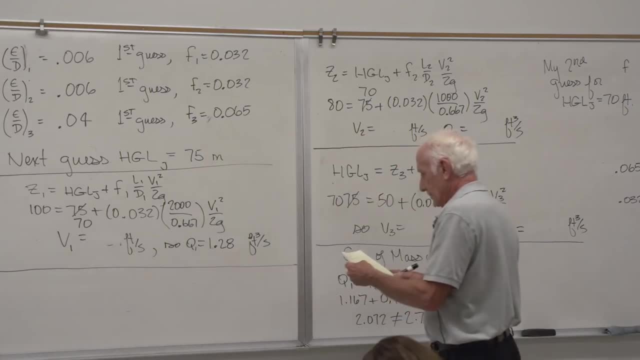 Q1, 1.28.. Q2, 1.275.. Q3, 2.477.. Qn. 2.555.. Q2, 1.2, 1.758.. Q8, 1.258.. Q8,. 2.274.. Q9, 2.274.. Q10, 2.368.. Q11.. Q12.. 2, 274.. Q14.. 2, 2023.. Q14.. Q14.. 2, 274.. 2, 273.. Q15.. Q15.. 2, 275.. Q16.. 2, 279.. Q21.. Q19.. 2, 2735.. Q20.. Q22.. 2, 278.. Q23.. Q22.. Q20.. Q20.. Q21.. Q22.. Q22.. Q22., Q26., Q23.. 1, point 27.. Q14.. 2: precisely Five, five, five. 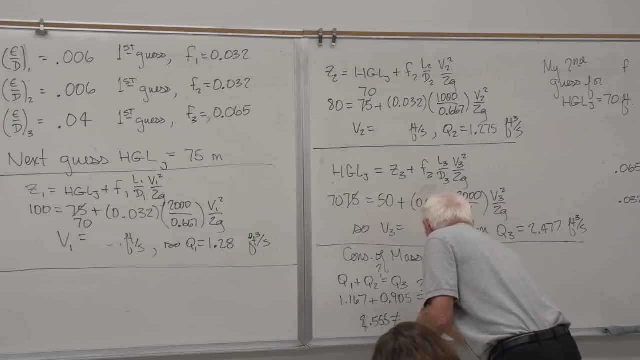 Q out: Two point four, seven, seven. Oh, I'm getting a real close now. 2.6 compared to 2.5.. I might just say, oh, I'm tired, I'm done, But not really you know. no sorry about that. Good try though. Good try I. 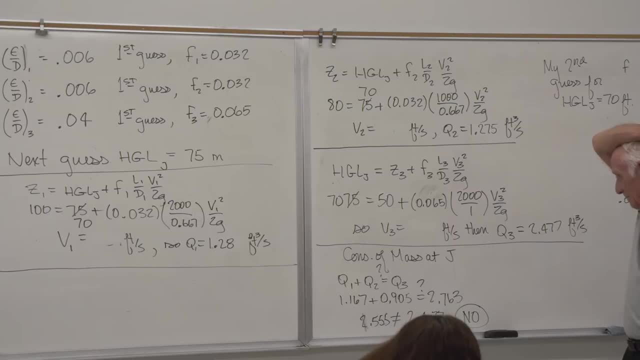 Say: oh my gosh, Okay Now. what's my problem now? This is how much comes in. This is how this is how much goes out. Okay, Two point four, seven, seven. That's good, That guy's got to be bigger now. He's got to be bigger, Oh. 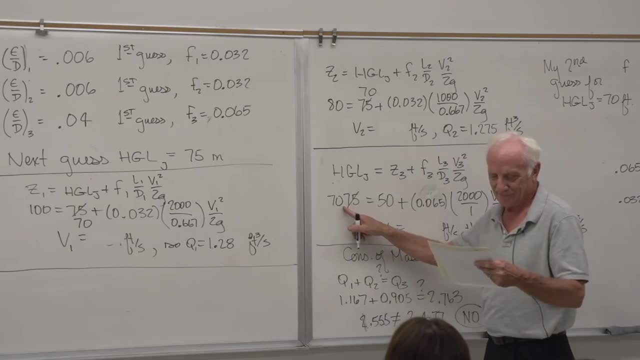 I went too low. I stopped, shouldn't have said 70. I Went through this thing two more times. Okay, by hand. It's, it's a. it's a pain, got it, That's alright. I got lots of time, Real, you know, I'll tell you the final answer. Okay, I was really close. 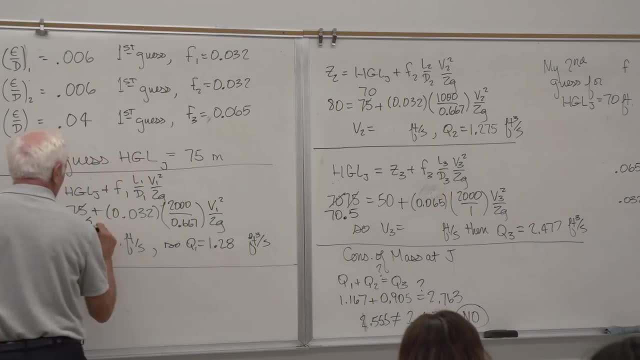 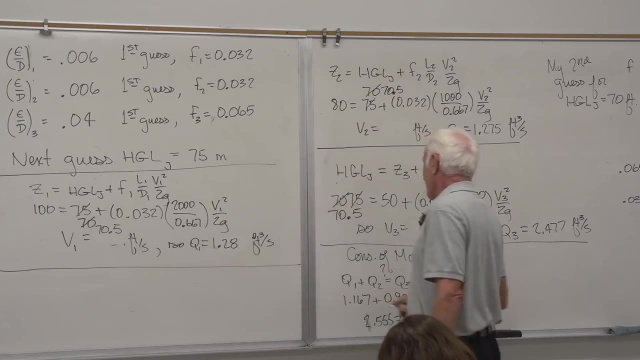 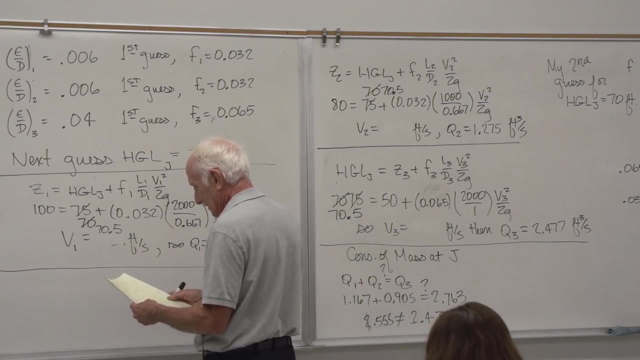 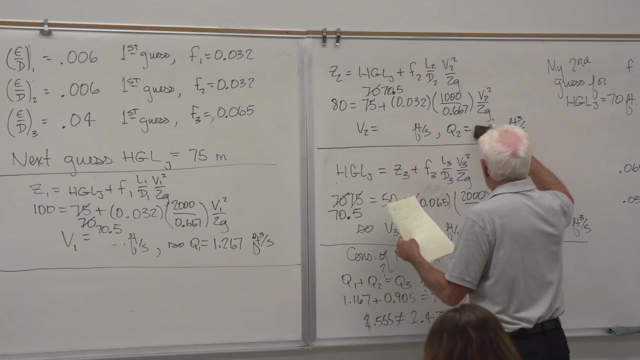 70.5, 70.5, 70.5. When I do that, Here's my new q1. My new q1 1.267. My new q2 1.249. my new q2 1.249. My new q3 2.516. 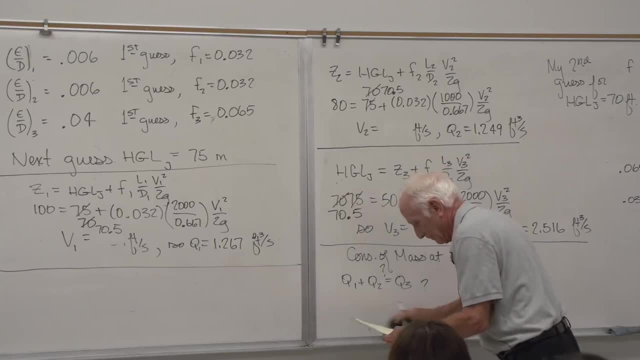 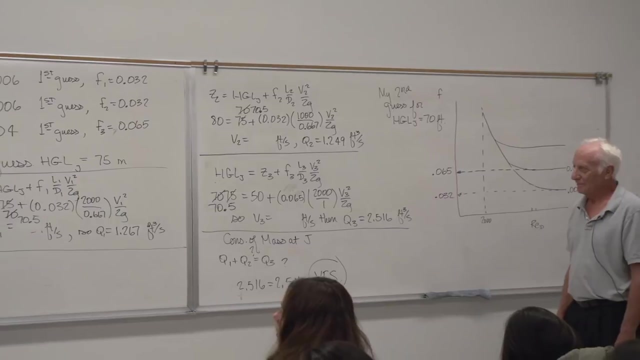 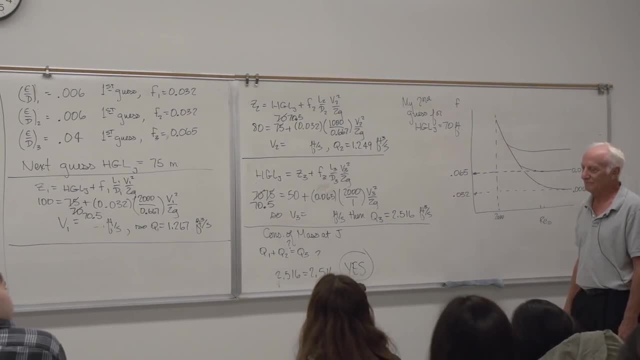 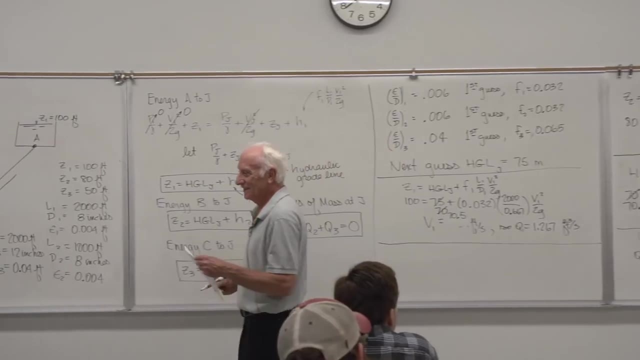 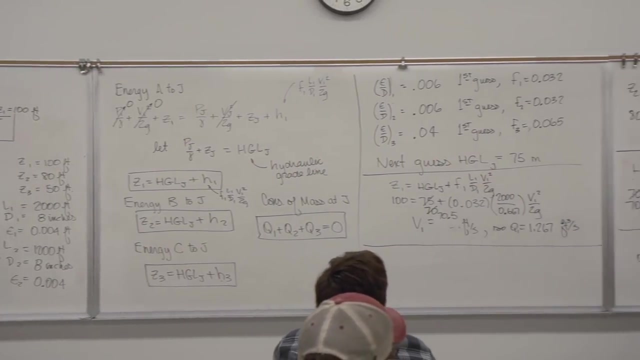 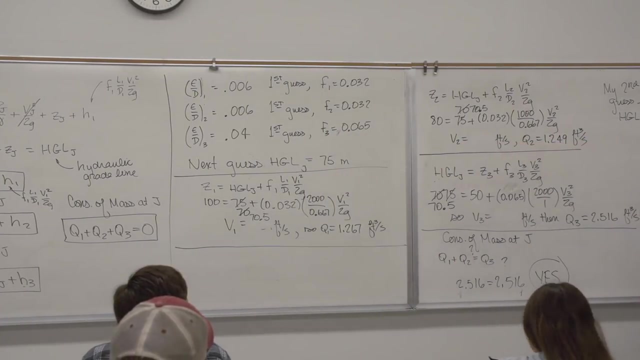 the hydraulic grade line at J 70.5.. Am I done? Oh, I wish I was done, but I know I'm not. Oh, this is miserable. What did I base those Fs on? Where it's flat out here? You know it's not going to be where it's flat out here. What's my next step? 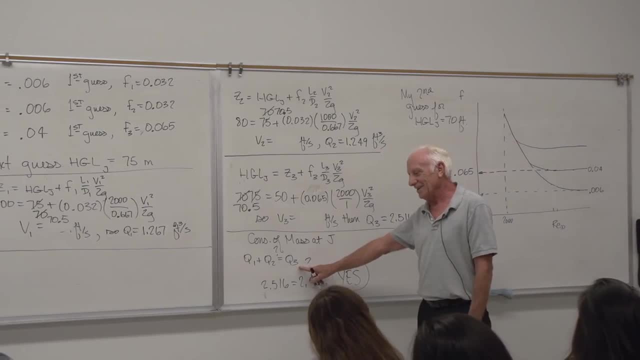 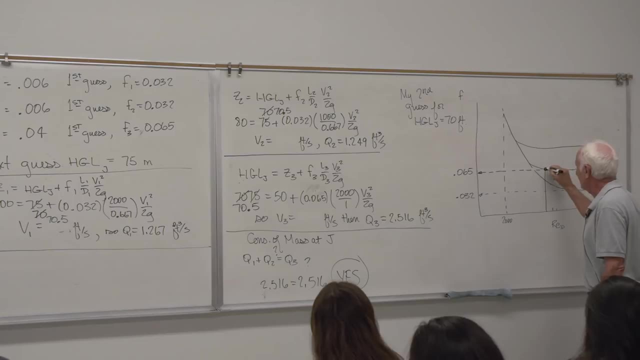 With those velocities one, two and three, I get a new Reynolds number. I go to the Moody chart with the new Reynolds number. I go up to the epsilon over D. I need to read over here and get 0.067.. Here we 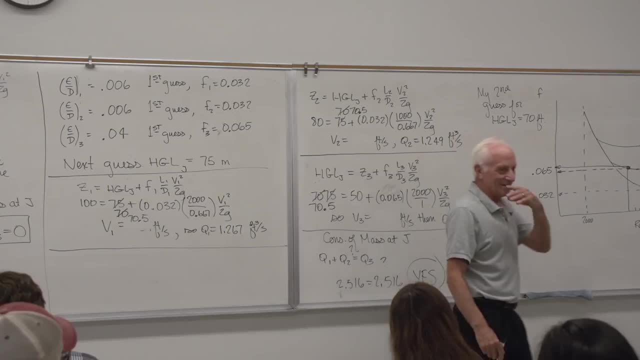 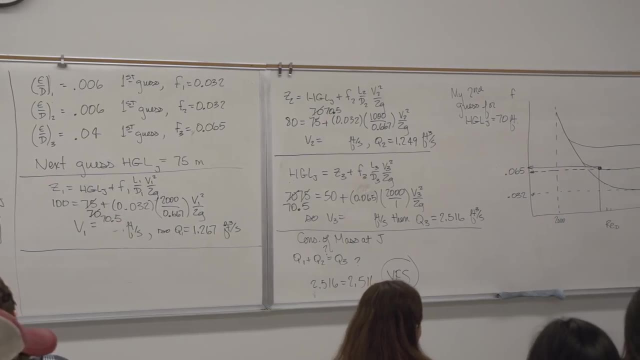 go again. All these equations make a guess. hydraulic grade line. Oh, these are nasty problems, But that's the way it goes in life sometimes. Now you'll never be asked on homework or an exam to go through completely and do this stuff. 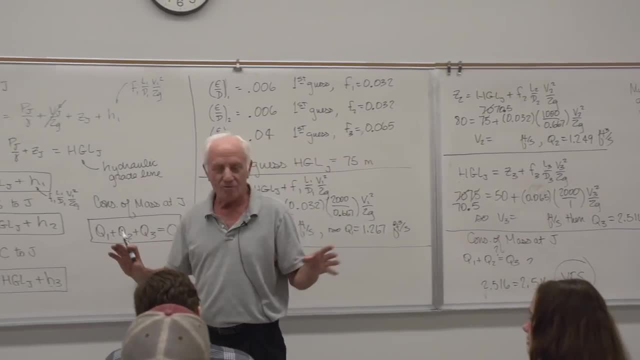 Again. if it would be an exam, I would say, go through it one time. If it was an exam, I would say, go through it one time. If it was an exam, I would say, go through it one time. If it was an exam, I would say, go through it one time. 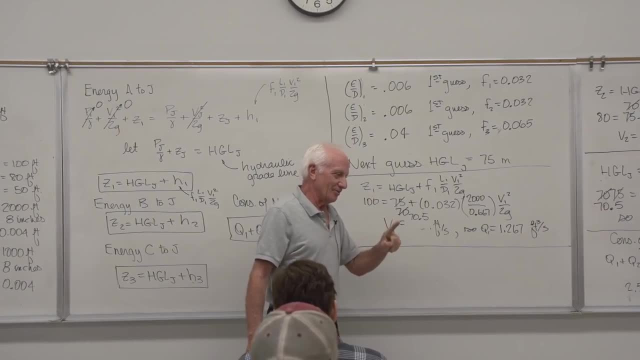 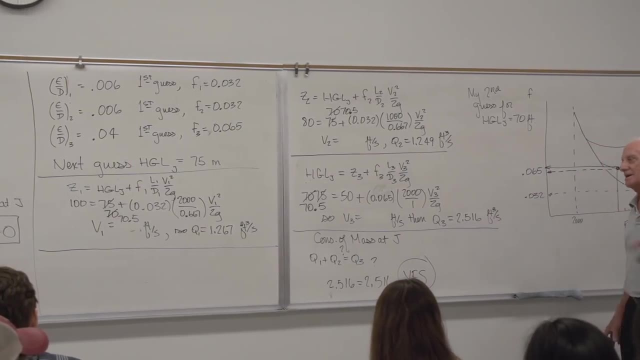 With a reasonable guess for hydraulic grade line and solve and see if you satisfy conservation of mass. But don't do any iteration. Okay, A lot of times in the textbooks they'll give you the F's. They're really nice. They say: assume the. 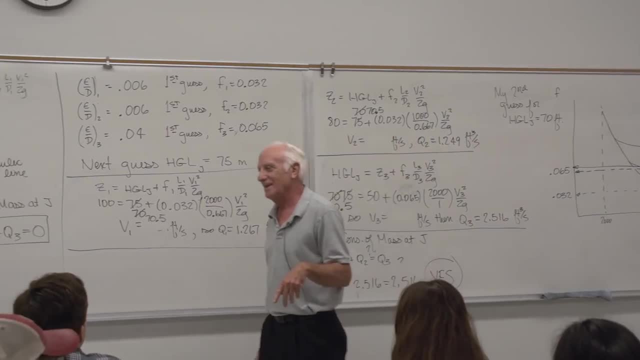 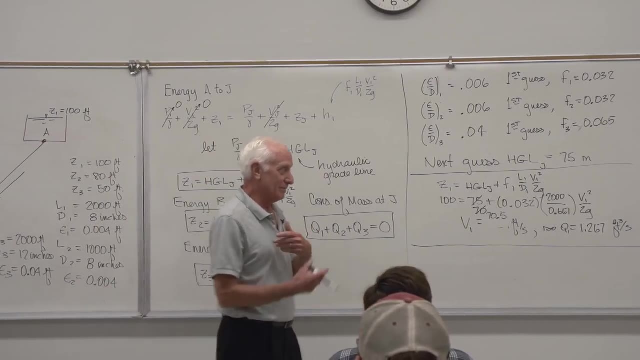 F in pipe one, two and three is blah, blah, blah, blah, blah. Okay, thank you very much. That means less guessing. Now I just guess hydraulic grade line with J, So that's typical of homework or even an exam. People don't ask you to go. 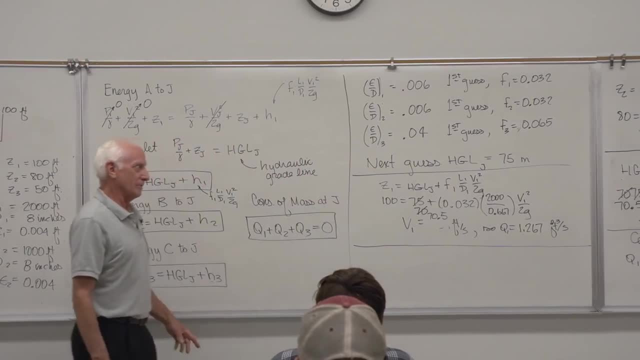 through all that gory detail In the real world. oh, in real life, that's a. You go through all the gory details. That's what you've paid for here. You get the big bucks. You got to work for it. So.